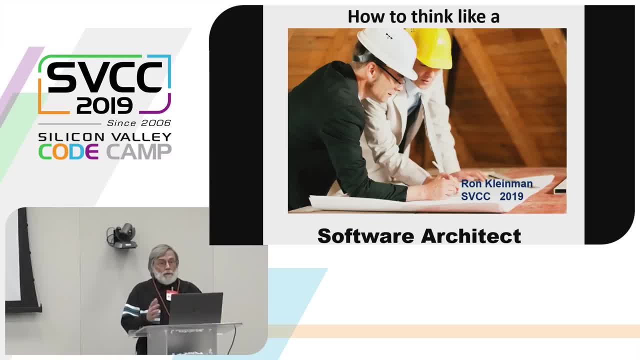 this thing started An awful lot of work with standards bodies in specific industries, like: how do retail all the systems that go on in a retail enterprise? You really want to be doing plug and play, which means you want to have interfaces for the point of sale system. 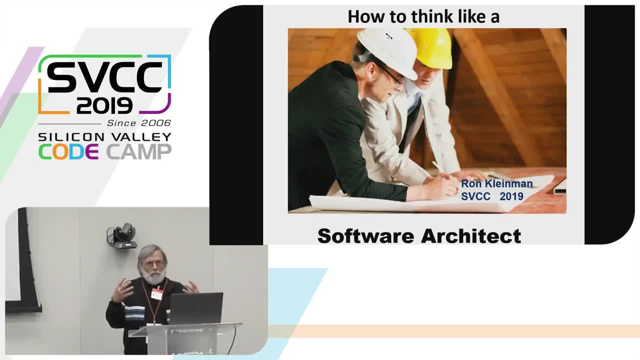 and the item inventory. You want to be able to go so that vendors would do these APIs and so you could plug and play. Actually, it turned out it was more plug and pray, But I was doing that in a lot of different industries and looking at how software architects sitting on those committees 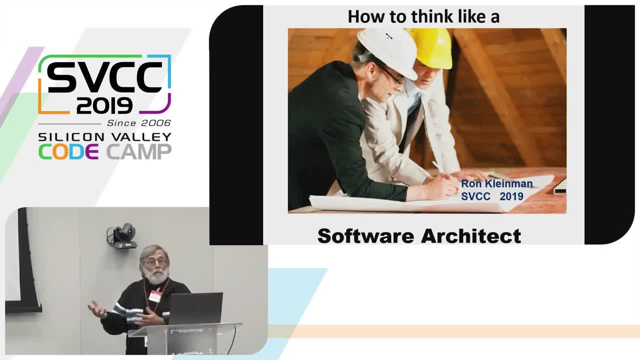 and realizing that a lot of what they were doing in different industries- although I didn't know about it- was a lot the same. So that's kind of where this came from. I actually started object-oriented analysis. Okay, Yeah, I think that's kind of where this came from. I actually started object-oriented analysis. 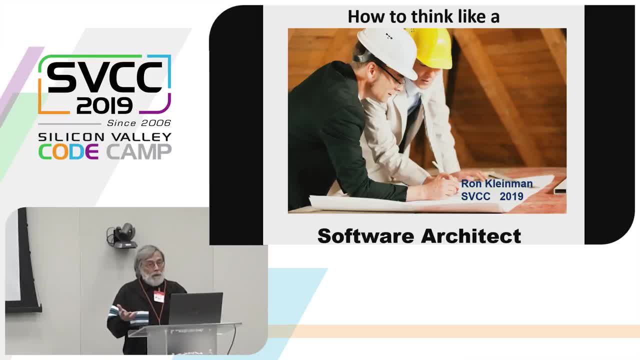 and design at the ANSA, because they introduced some object languages and I said to a student: how did you find it? And the answer was: oh, it's great. C++ is great. Slash- slash is a comment. It's like: no, you're not using the language. So anyway, that started this. 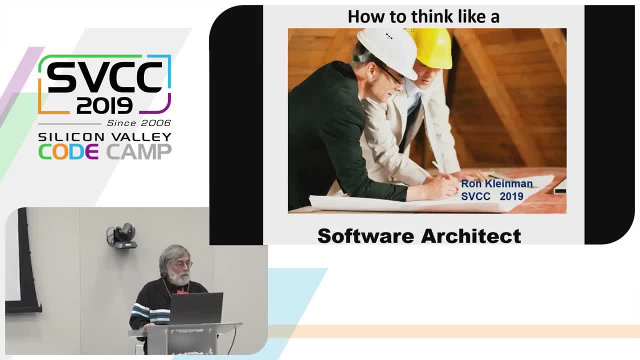 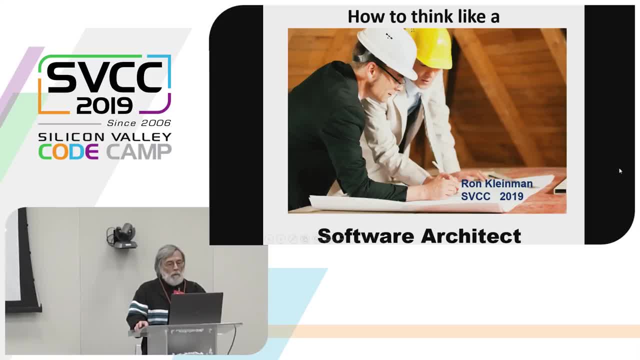 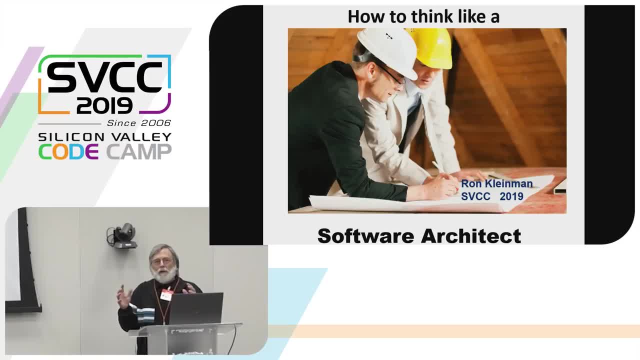 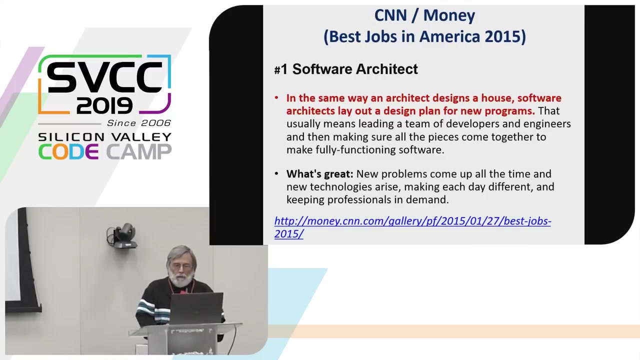 way, and when you look at the series of languages, you start seeing what drove the evolution of languages. And it will look. So I think—are we good? We start, Okay. So the priest thing is down on tape. Okay, So here we go. How to think like a software architect? Now this: 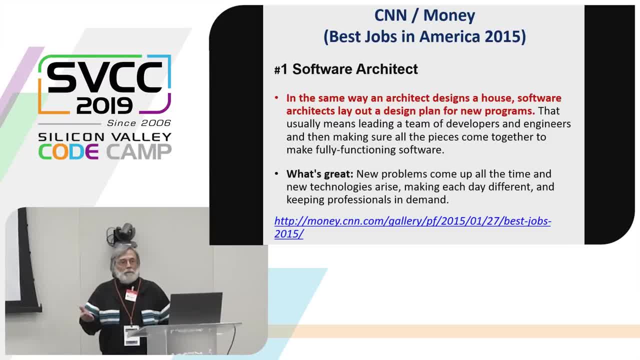 goes back to 2015,, which is admittedly the dark ages in computer science, But CNN Money Magazine- and I love this- it was the number one best job in the United States- was software architect And the analysis to understand what it is. you think about the way that an 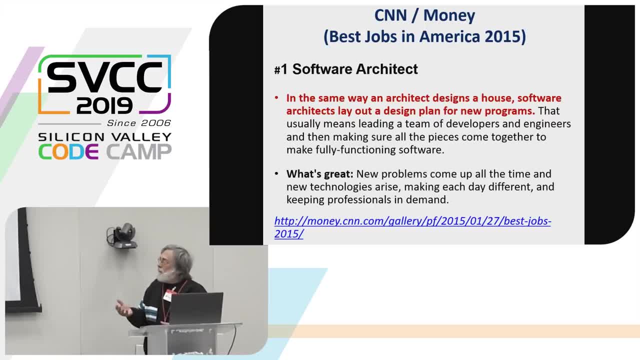 architect designs a house. a software architect lays out plans for new programs. An architect uses blueprints. a software architect may use UML, which is Unified Media Language Diagrams. There's a lot of them. The ones that really matter are the ones that don't document what. 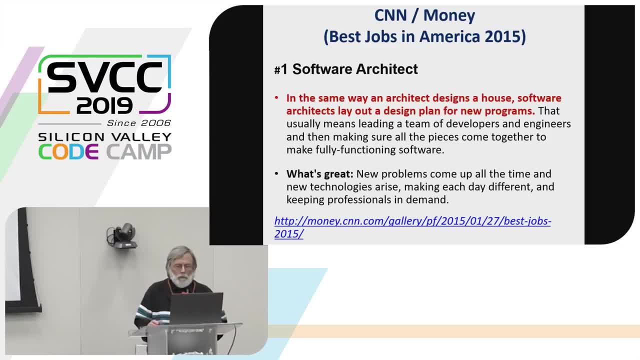 you've thought, but actually have They help? you think about the problem and we'll look at a few of those. You know, new problems come up all the time and new technologies arise, making each day different and keeping professionals in demand. and that is true. One other thing: what we're going to talk, 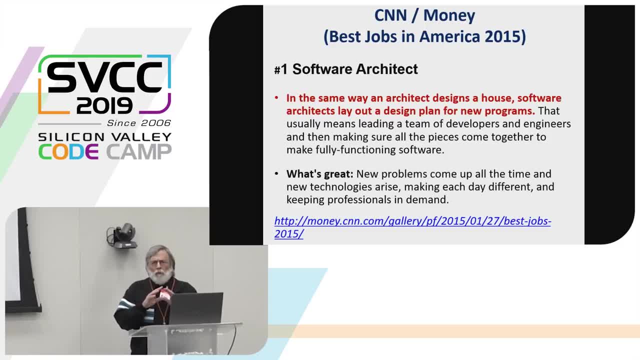 about are the kinds of applications that are ubiquitous everywhere but in the valley, Because in the valley it's all about eyeball capture and customer capture and front end and this, and that The systems that we're going to talk about being architectured in an object-oriented 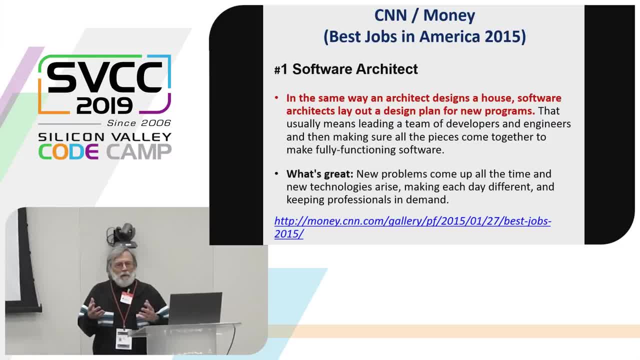 fashion Are the back office stuff. Most of the programming jobs in this country are working as in the IT department of a major corporation- Now that corporation is located in Kansas City or Minneapolis and you don't see it here- Or working for companies that sell to major 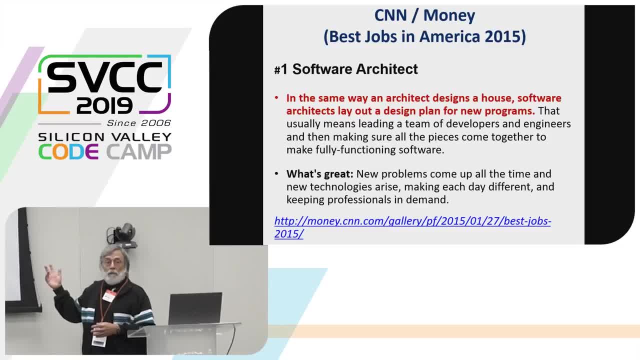 companies, not customer-facing companies, And the systems that we're going to be talking about are the way the world works. Every company, every school, has a plethora of programs that inter-operate and are designed in the way that we're going to talk about, And it's one of. if you're in, everybody knows this, but 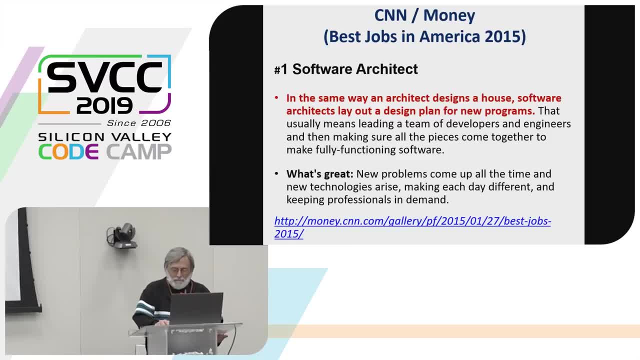 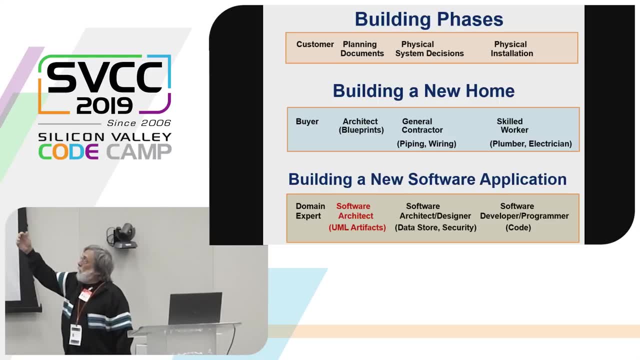 people in the valley. So let's take a look. If you're building a house or you're building anything, really, there's a customer planning documents, some physical design decisions and then the actual installation. This is what we're going to talk about. This is what we're going to talk about in the future. 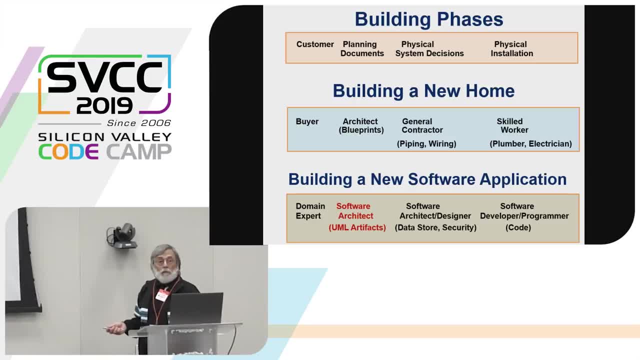 And if it's a house, you have a buyer and you have an architect who does the blueprints. You have a general contractor who makes decisions like: what type of plumbing are we going to use? Probably better to use copper than lead, right? 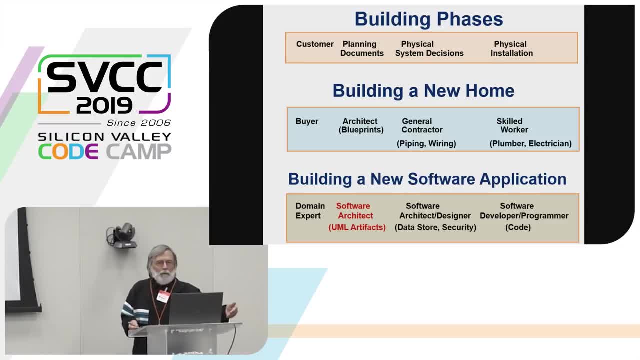 What kind of wiring are we going to do? What kind of plug-in are we going to have for the speaker? And then you have the skilled workers come in and they do the electricity and the installation of the actual wiring and the plumbing and they make it real. 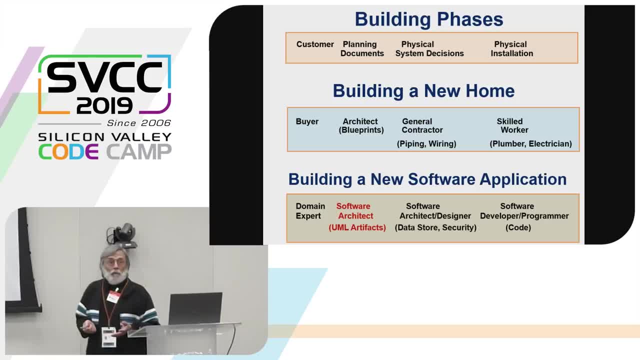 And in a software application. this parallels the development of a software application. The buyer is the domain expert. So if you're in retail, the buyer of that particular system might be the head retail data person. If it's in a college- and the example we're going to do is from a college- it might be the registrar. 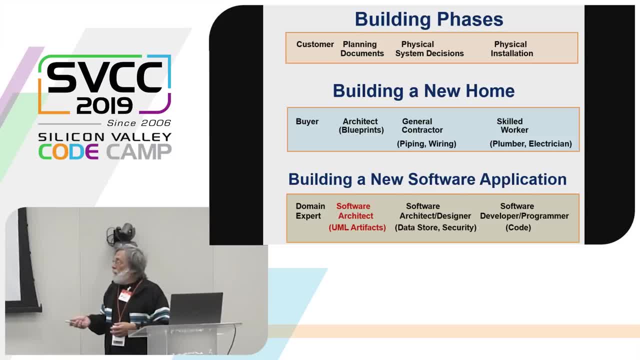 Someone who knows the application doesn't know the programming. The software architect functions as the architect does in a house. The blueprints are these UML artifacts, and we'll see two of them. before of the big five, We'll get a chance to see two of them. 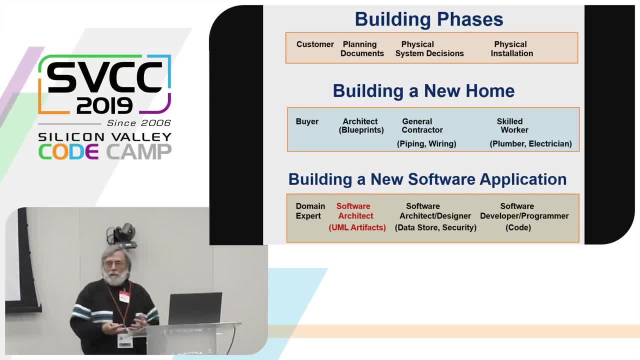 General contracting. that's the aspect of any application. It's the thing that says you've got your application right. How did you do security? Is your data going to be local in the cloud? Is your application going to be in the cloud or in the data center? 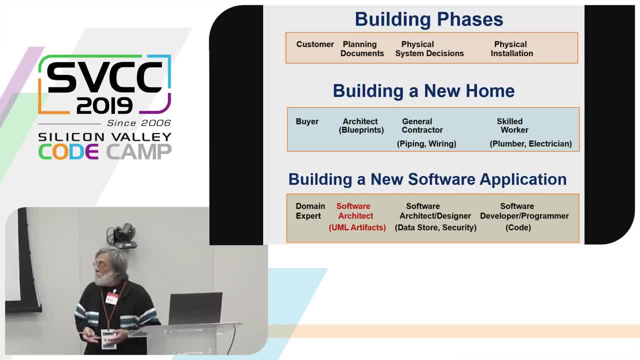 Those are mainstays, Those are major decisions that you have to make, And the people who do that are sometimes a software architect, sometimes it's like the designer, And then, when everything's laid out, programmers come in and implement it. Now, sometimes, admittedly, the programmer can be wearing a lot of hats. 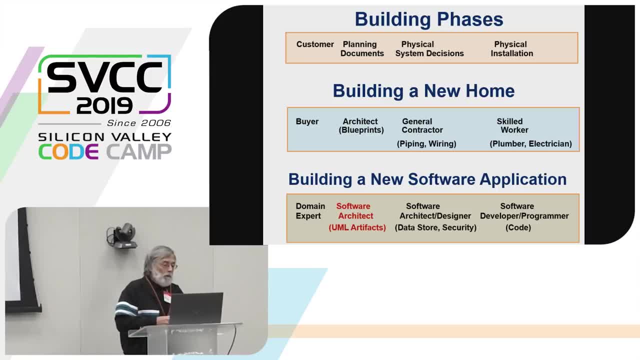 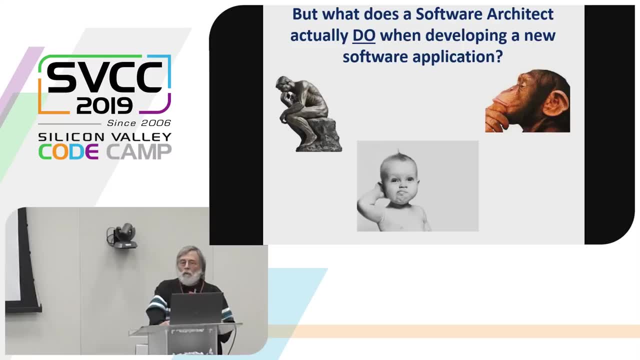 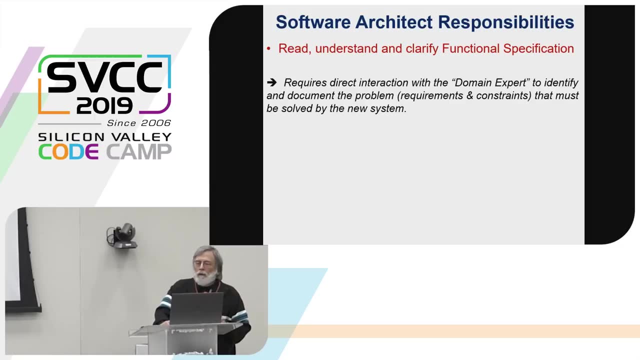 You know, if you're on a small project, you do most of that yourself. But for large projects they really are different. But what does a software architect do? What does a software architect actually do when developing a new application? So the first thing is read, understand and clarify the functional spec. 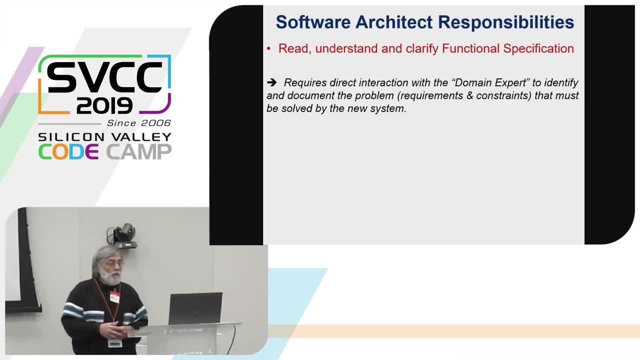 This is typically a one-on-one interaction with the domain expert. What is this system trying to do? to identify and document the problem, the requirements, the constraints and so on. Now the next slide is an example. This was an enrollment system at De Anza College. 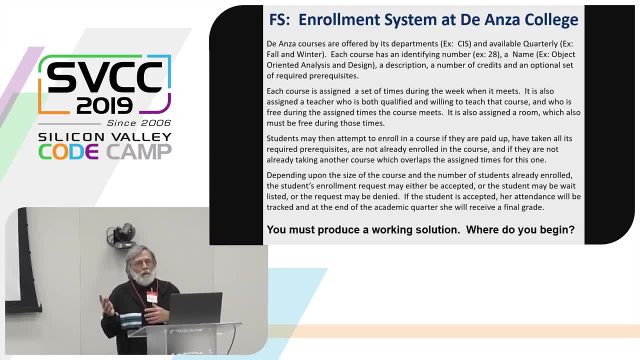 My thinking here is, when I presented this, that I knew that everybody in the audience had actually used a system like that, because otherwise they wouldn't actually be sitting in the room. People here, I'm sure, have enrolled in courses at different schools. 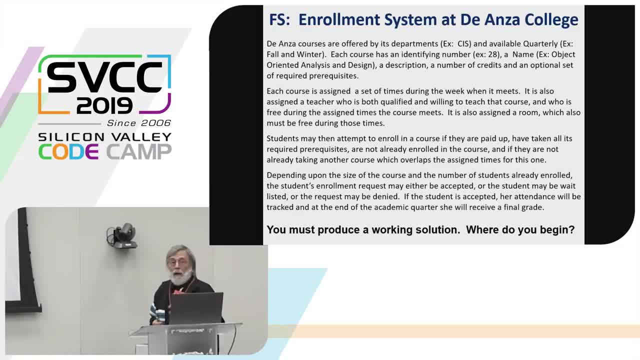 And so we're going to take a look at what's involved with something like that and how you think about it. So, again, this is a very quick read and I'm just going to highlight it. De Anza courses are offered by its departments and available quarterly. 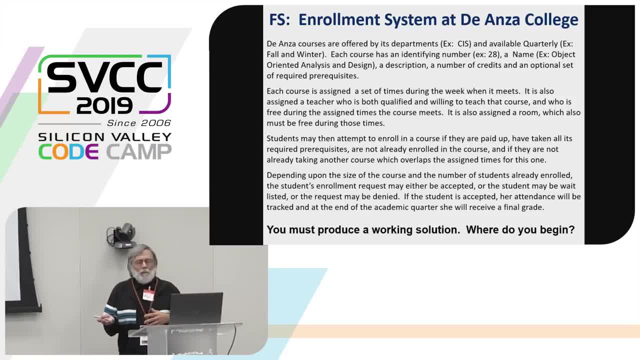 Each course has an attachment, An identifying number, A name- This is, in my case, object-oriented analysis and design- A description, Number of credits, Optional set of prereqs. Each course is assigned a set of times when it meets. 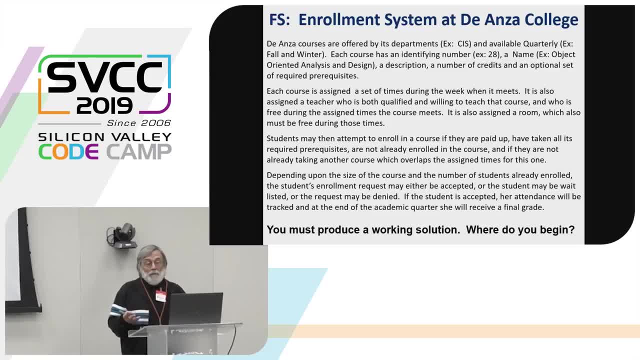 Assigned a teacher, Qualified and willing- You can be willing, but you may not be qualified- And who is free during the assigned times. It's assigned a room, which also must be free. Students may then attempt to enroll, And then there's some requirements on that. 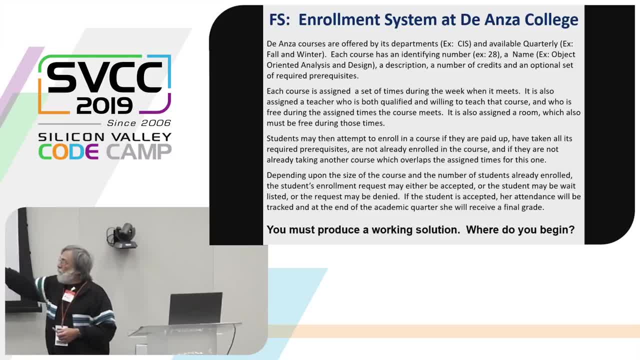 And, depending upon the size of the course, the number of students, the student's enrollment request may either be accepted, or the student may be waitlisted, or the request will be denied. If the student is accepted, her attendance will be tracked and at the end of the academic quarter she will receive a final grade. 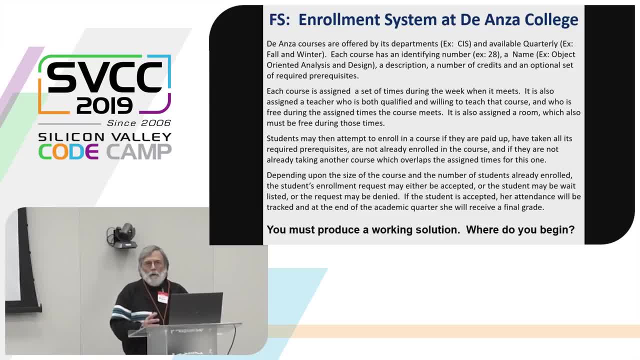 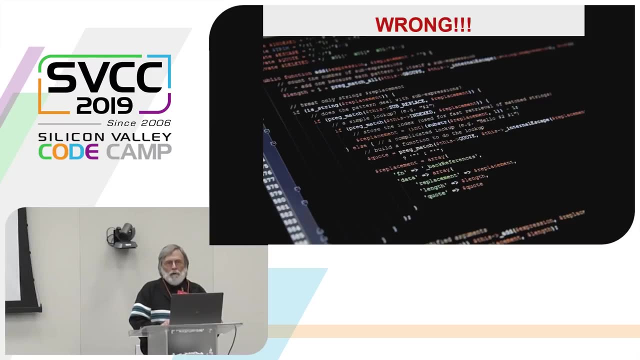 This is a very high-level and brief functional description of a combination of class scheduling and enrollment. It's a system. You must produce a working solution. Where do you begin? This is the wrong answer. You don't start coding, In fact, everything between what I give an entire course on what occurs between the functional spec and this. 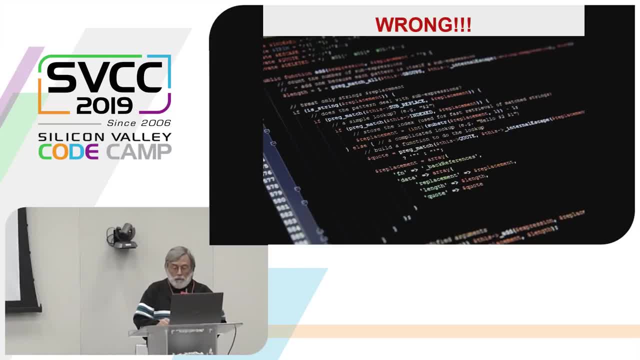 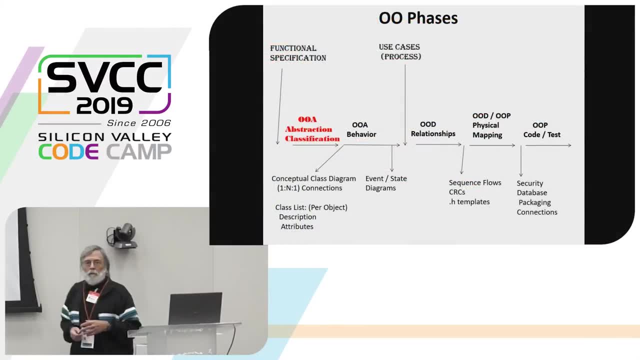 Okay, It's the thinking about the problem. that's really the interesting thing. So this is a diagram for how systems are developed using feature-driven design, And we are. We start out with the functional specification. This is the piece we're going to get to today. 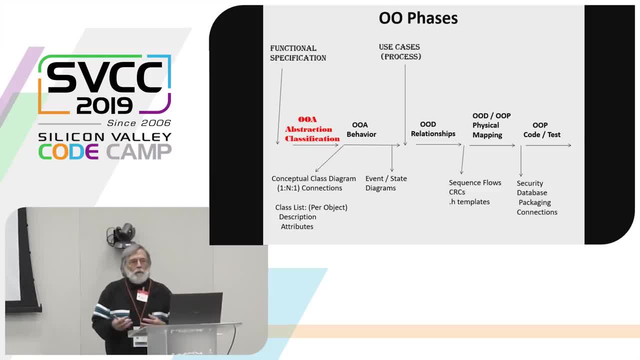 Going through and thinking about what are the basic abstractions in the problem and how do they interact and how do they relate together. When you have the basic abstractions, you then flesh out the behavior. Remember I said that, the section you could know every interface to a course. 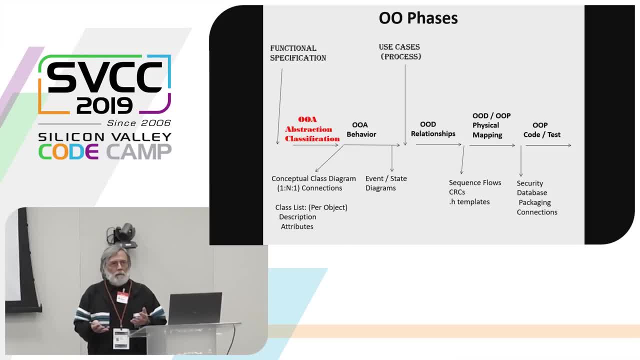 You could know every interface. You could know every interface to a course object, But you wouldn't know. if you said I want to enroll, you wouldn't know whether what the reaction was going to be, Because the course could be filled or the course could be empty. 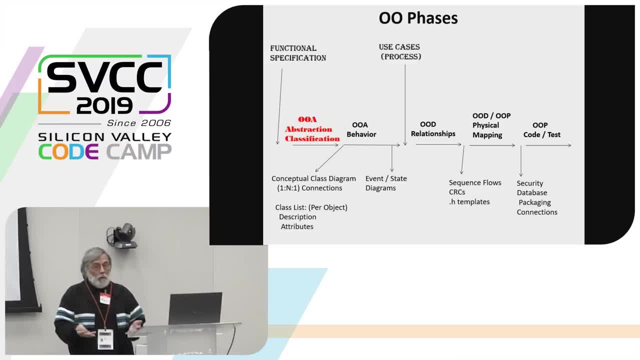 You know. so some cases you'd be rejected, Other cases you'd be put on a wait list. That's behavior, And behavior is stateful information. So once you get your objects and they're stateful, then the various use cases, like enroll student in section. 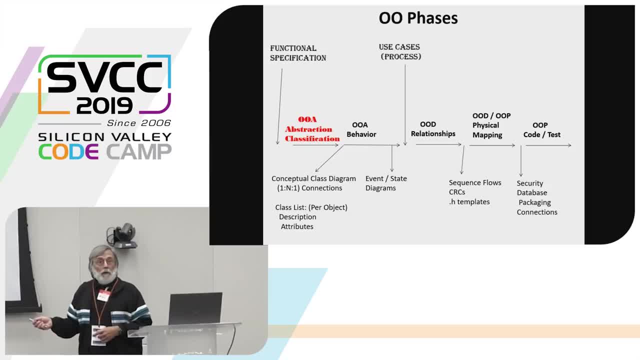 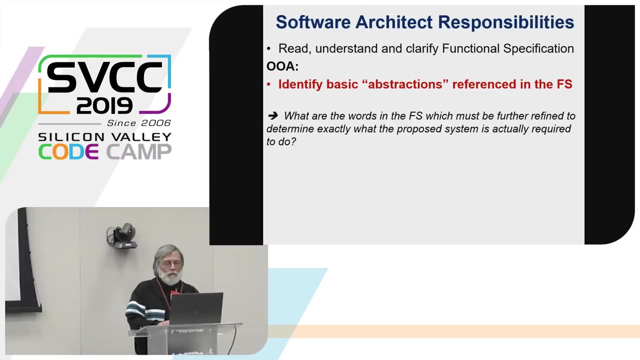 are taken and analyzed against the objects that you have to make sure that you can do the application as defined. So we're going to concentrate on the first part to give you an idea of the thinking that goes into a typical application. So again, number one: identify the basic abstractions referred to in the functional spec. 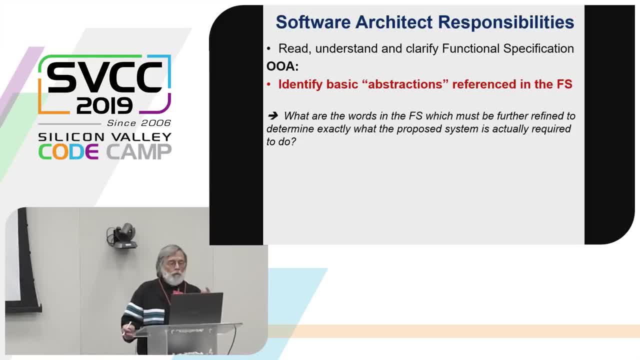 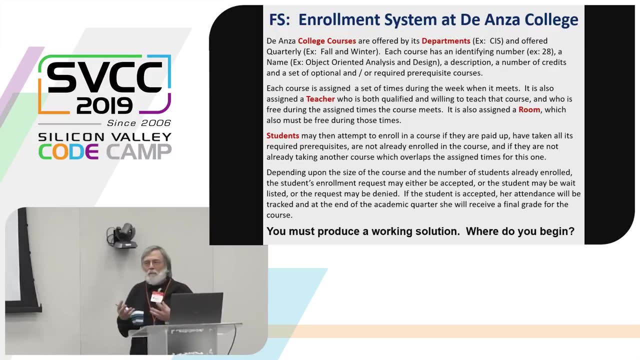 And in the functional spec we looked at there were some words that must be further refined To determine exactly what the proposed system is actually required to do. So we do that. We go. the answer: college, College, sounds like a thing I'm going to be manipulating, right? 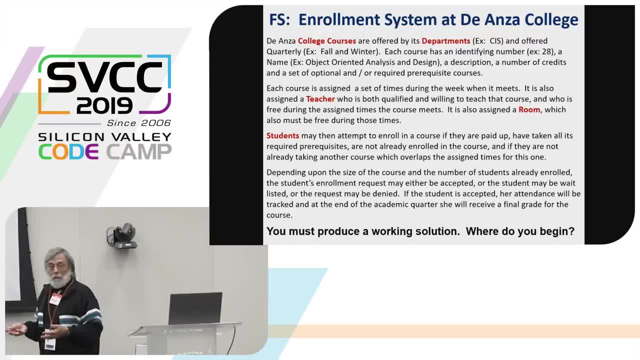 Courses. Courses are offered by its departments. So I'm thinking, okay, I've got colleges, I've got courses, I've got departments. How hard is this? right? It is also assigned a teacher, okay, Who is both qualified and willing. 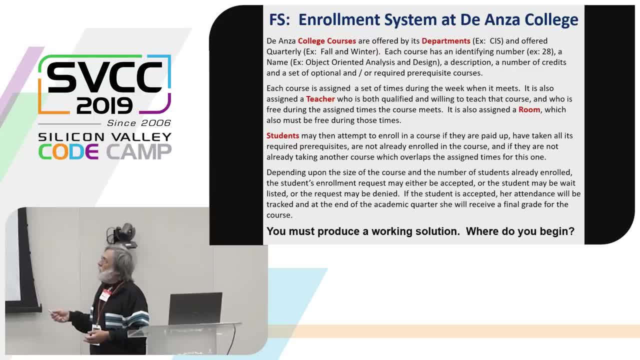 It is also assigned a room Students. And I look at this and I'm saying, okay, I kind of have, at least conceptually, some of the abstractions that I'm going to be dealing with: Course, college, teacher, department, room and section. 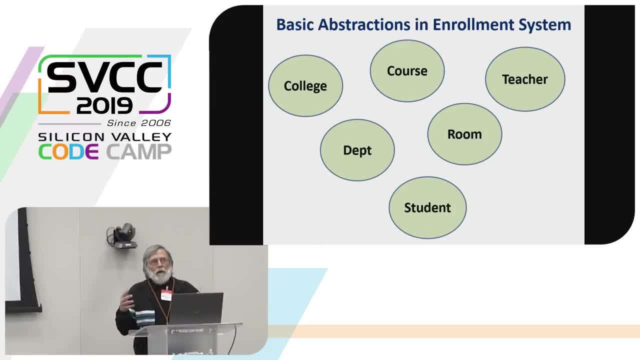 And I start out and I say, okay, so far, so good, right. And then I start thinking about it, Because one of the things that's true when you are designing a system is that words have meaning And everybody on that system design, whether it's the architect. 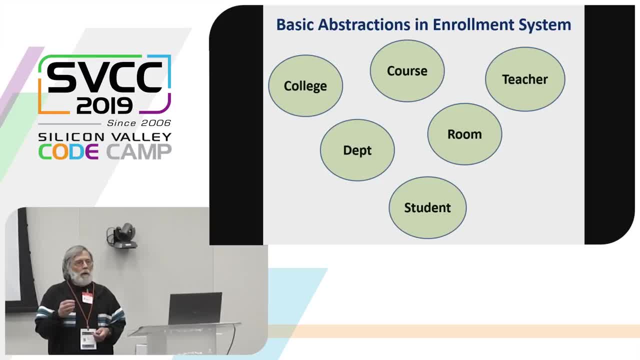 the designers, the programmers, the customer, everybody has to have a very clear and crisp definition for what the names that you're assigning these abstractions, what they fully mean in the context of the application, Because the same word can mean totally different things in different applications. 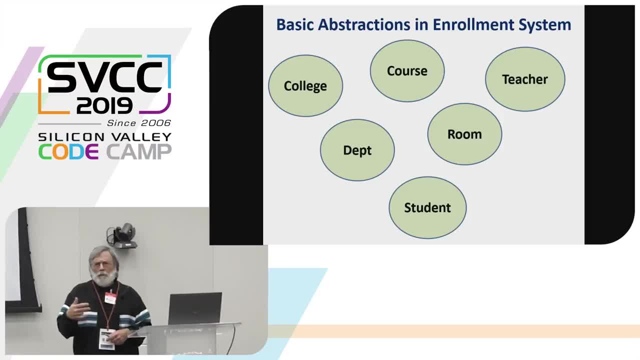 You know, one example I give is a birth record, A birth record system, where one of the things there's an attribute that's like blood type And that attribute is like a string. It's OH positive, whatever If that application is a blood bank. 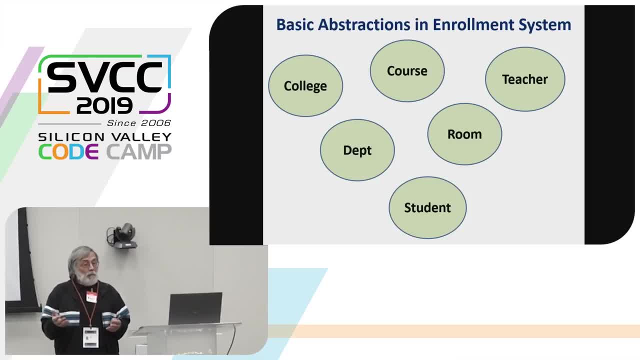 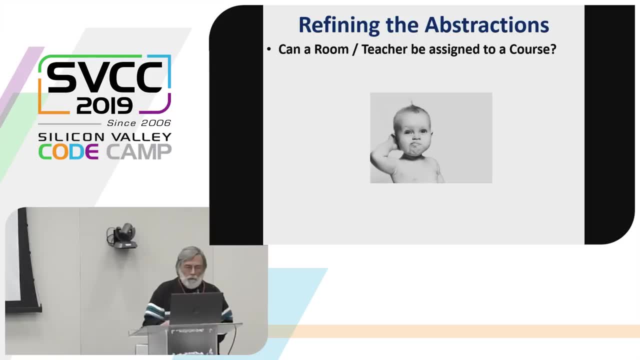 blood type is this huge object with all of the capabilities. Same word, but in a different application It means something totally different. So here I start asking questions: Can a room and a teacher be assigned to a course? In other words, how many people have enrolled in a course at a college? 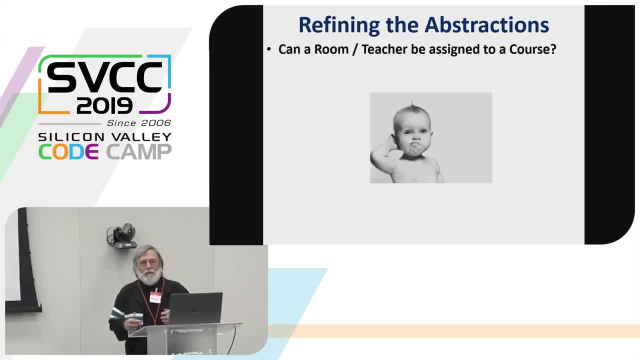 How many people? That's it. Yeah, okay, good, Good, Thank you. One of the things I find in my classes like. I'll do exactly that. I'll say how many people have enrolled in this course, And in a class of 40 people, I'll get 15 hands. 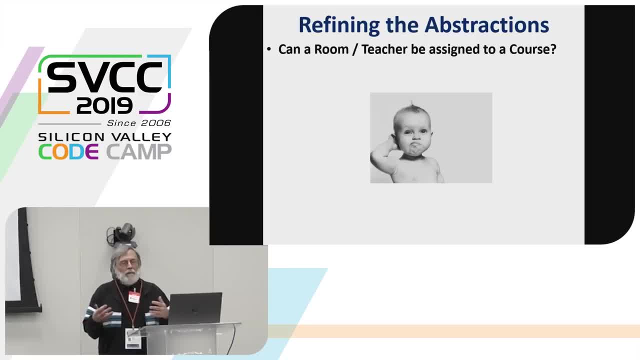 And then I say: and how many haven't? And then I get no hands And I get 15 votes out of 40 people. And I always tell them that's why we have the president. we do Okay, But anyway, thank you. 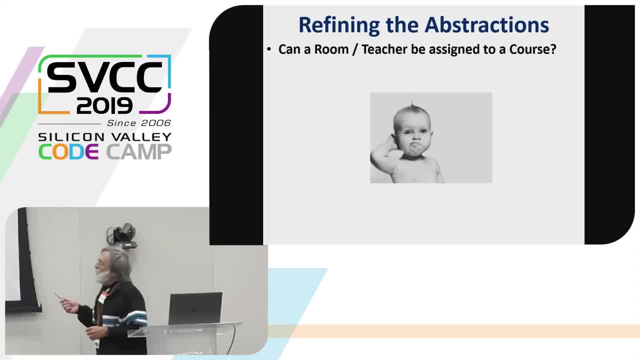 That's on the tape too, of course. So the question is: how can you know, can a room teacher be assigned to a course? And you think about it and then you know you go. well, that's tough, right. 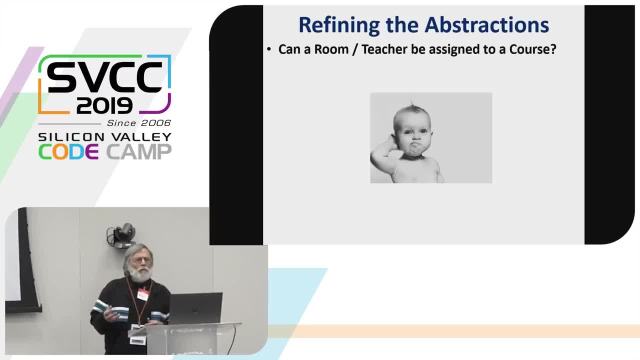 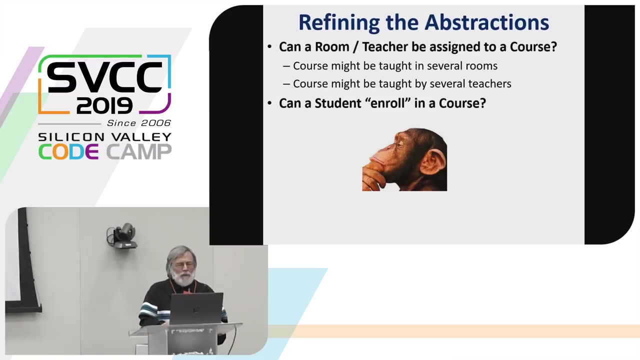 Because you know you've got a course and like introduction to Python, And you know it's given it four times during the week in four different rooms with four different teachers. How can they all be assigned to that course? It's not, you know, it's just. it's a little strange, you know. 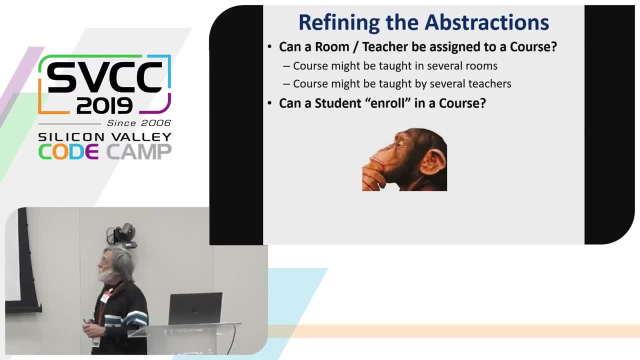 because a course might be taught in several rooms. A course might be taught by several teachers. If you enroll in a course, which teacher are you getting And which room are you getting? And you start to think you know I'm missing something here. 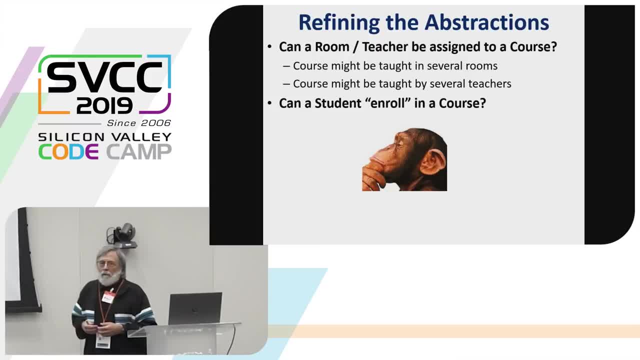 It's that uneasy feeling that you get when you realize that your vision of the problem doesn't really match up with the actual reality, reality on the ground. So we need a new abstraction. There has to be. there's an object or an abstraction. 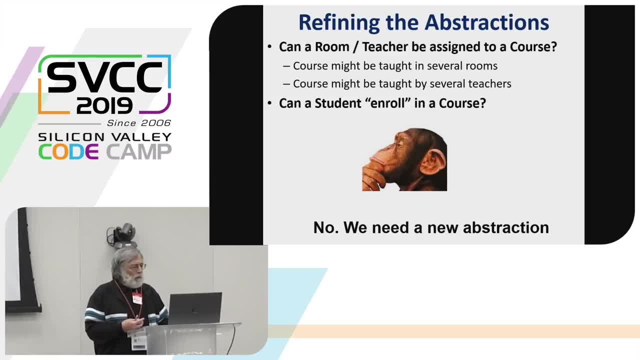 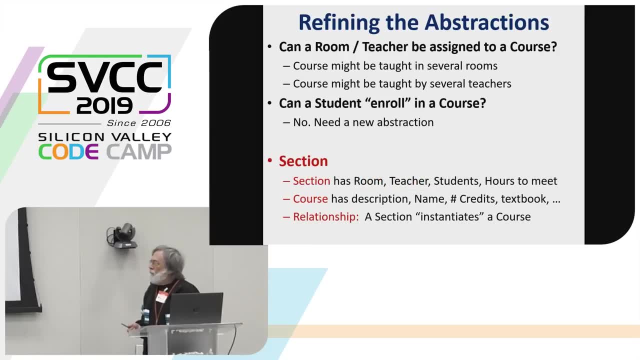 that's missing from the initial set of objects that we had And we need a section, And a section has a room, teachers, students, hours to meet. A course has the rest of it, Has description, name credits, the textbook that you might have. 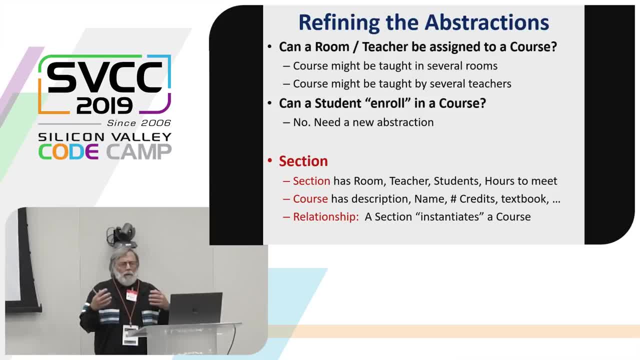 You know again, what quarter is it offered? And there's a relationship between the two And it's a one-to-end relationship And that is. a course has multiple sections And a section. each section is a section of one course. 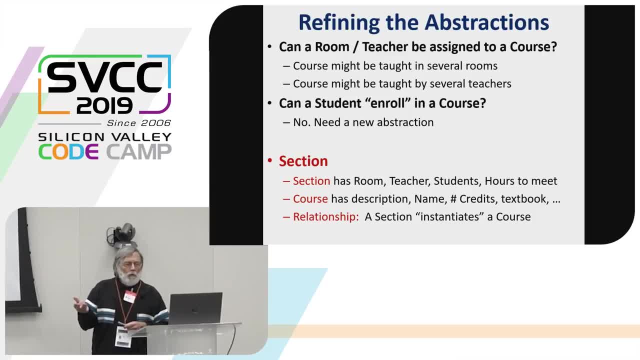 So you've got an end-to-one relationship between course and section And relationship is instantiates, In the same way that an object will instantiate a class. So if you have a class scientist, an object of that class is Albert Einstein or Isaac Newton. 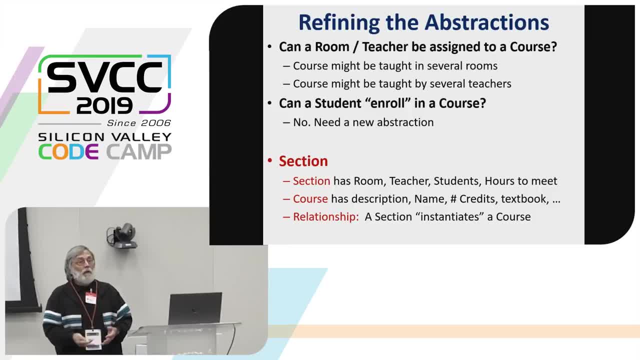 It instantiates the concept, An object instantiates a class. In the same way, you know, conceptually, at least, a section instantiates a course. It's the relationship. Now, again, one of the things you could say is: 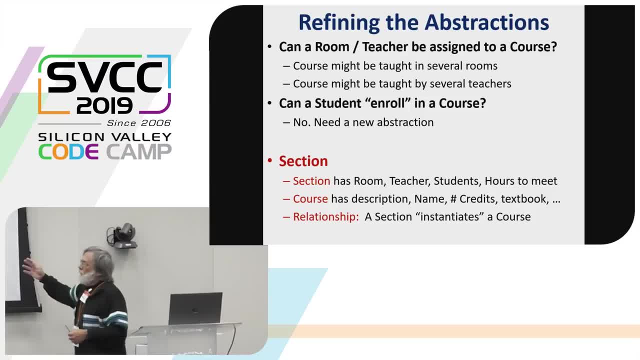 well, you know, you could carry what. do you even need a course? You could carry all this information in each section. Every section could have the name of the course and the textbook, and you know. But then if you have five sections of one course, 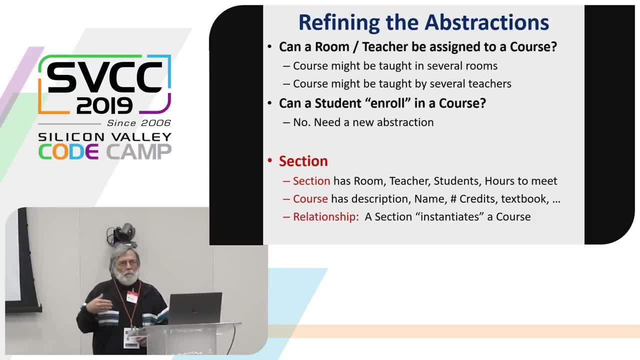 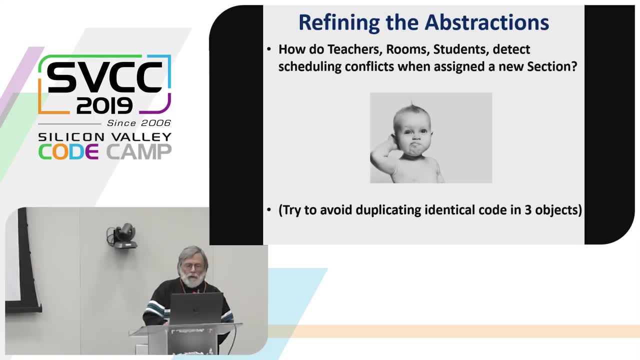 you've repeated the information five times. It's much better to keep the abstractions separate and relate them through an instantiate relationship, Refining the abstractions. So now we've got a problem here when we start thinking about it more. We've got sections now right. 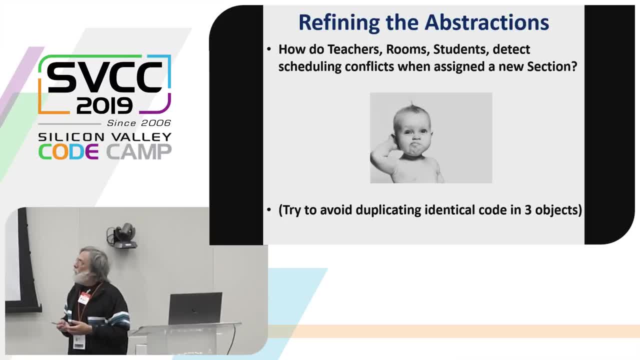 And the question now is: how does do teachers, rooms and students detect scheduling conflicts when assigned a new section? Because one of the requirements is obviously, you can't attend two sections that overlap. You can't teach two sections that overlap. 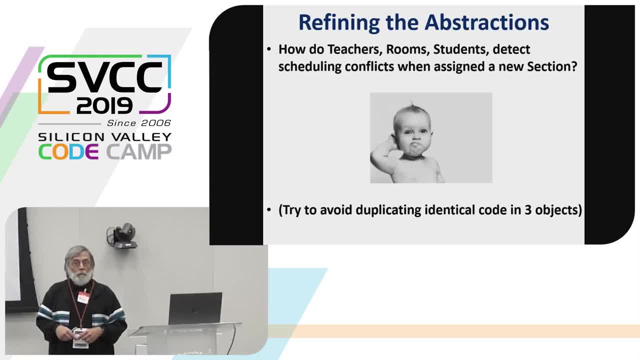 And you can't host in a given room two sections that overlap. So there's obviously going to have to be some scheduling stuff you're going to have to do And you're going to have to do it for teachers, rooms and students. 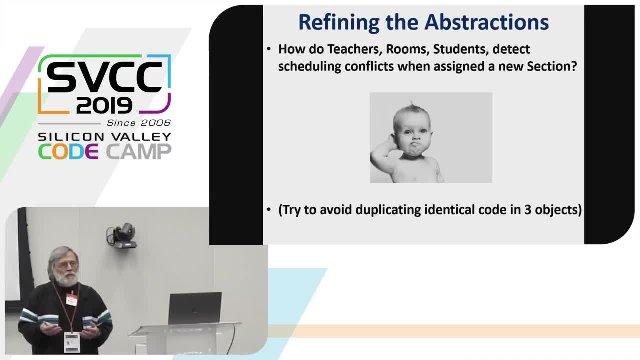 And so you're looking at this and you're saying: you know the same logic is going to be presented three times. I'm going to have to write the same logic three times to be able to schedule teachers, rooms and students. You have duplicate functionality. 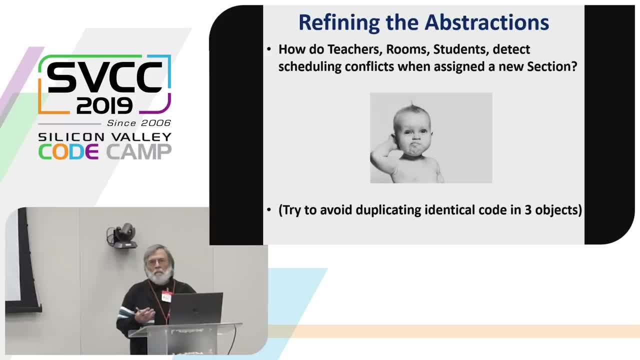 in three objects And that seems wrong. And at that point you think- or you should think if you're a software architect- duplicate functionality in three separate objects. this is a design challenge. I cannot possibly be the first person to encounter this problem. 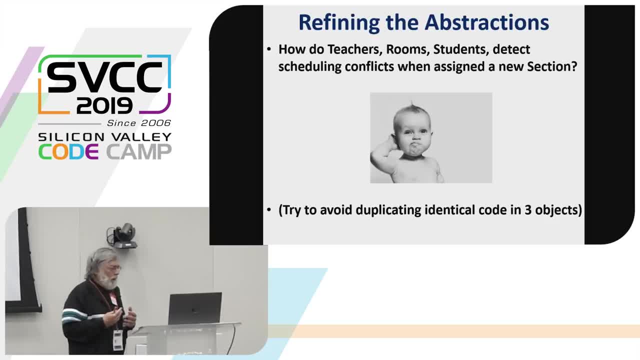 And you're not. There's a thing, and I'll ask for a show of hands seriously voting. how many people have heard of design patterns? Oh, fantastic, That's fantastic. Okay, design patterns. for the two people that didn't raise their hand. 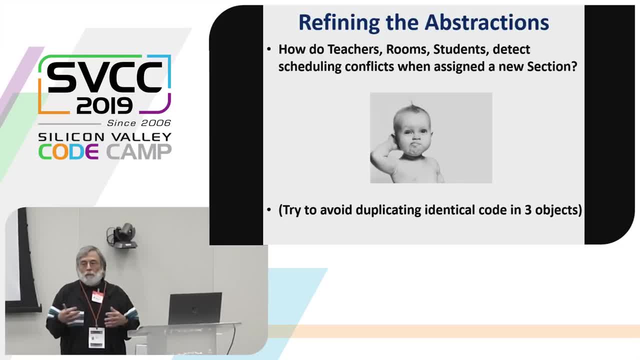 Design patterns are kind of like object libraries. It gives you a chance instead of reusing code, it gives you a chance to reuse thinking, And so a design pattern here is each assigned their own schedule, When in doubt, when you've got, and you can refactor. 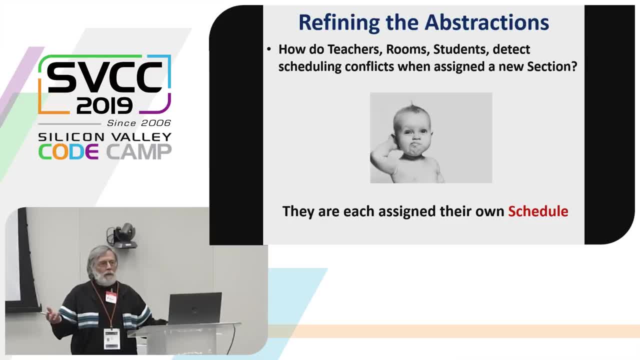 when you have the same logic that's being repeated again and again, what you realize, or what you could do, is to incorporate all of that in an object- one object- and have everybody else use it. This doesn't sound like a great step forward. 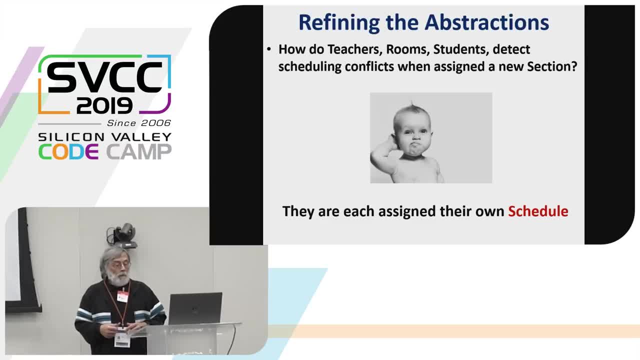 but schedule is a particularly good example of this, because with schedule you don't even have to know how to write that, You don't have to know how it was set up. The only thing the schedule object does externally right is, you could say, 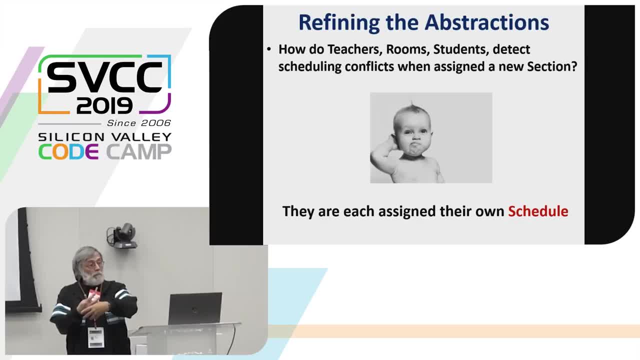 here's a schedule for the section. here's my schedule. is there a problem? And the schedule comes back. Your schedule object comes back and says nope or yep, There's no you could say to your schedule object. 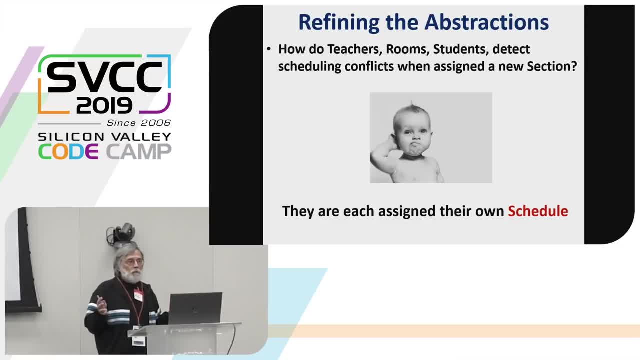 please add this schedule, and it does. You have no idea how that was done. The person who implemented the schedule has the idea how that was done. That's why they're objects. The thing about objects is they encapsulate their implementation. So we started with these six. 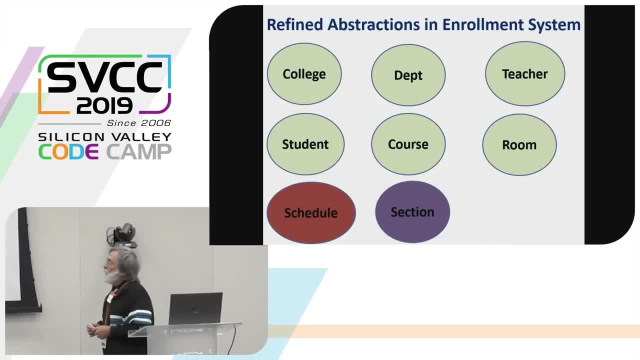 and now we've got two more. We said, you know, in terms of the abstractions in the enrollment system, we've just added schedule, which is going to save us a lot of problems in figuring out how to make sure that both teachers' rooms and students. 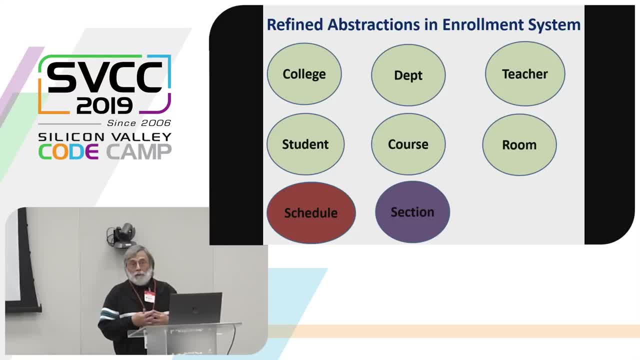 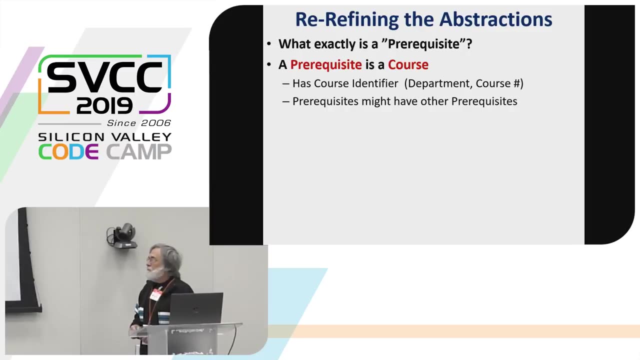 don't have schedule conflicts And we have a section which is distinct from what we thought was a course And we're starting now. that's been the morning staring at the ceiling. Okay, what's a prerequisite? Prerequisite means it's a requirement. 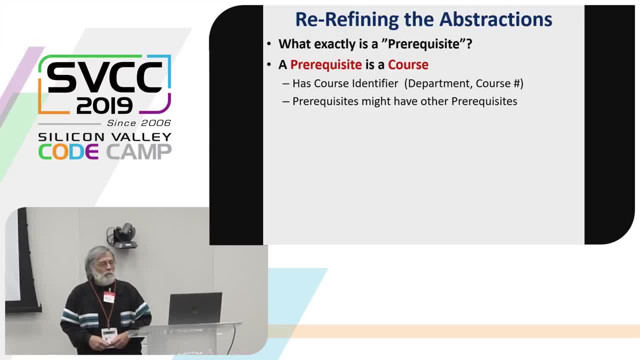 you know right. You say: well, you know a prereq, it's a course, It has a course identifier, right. Like you: can't take CS28 until you took CS3.. So the prereq is CS3.. 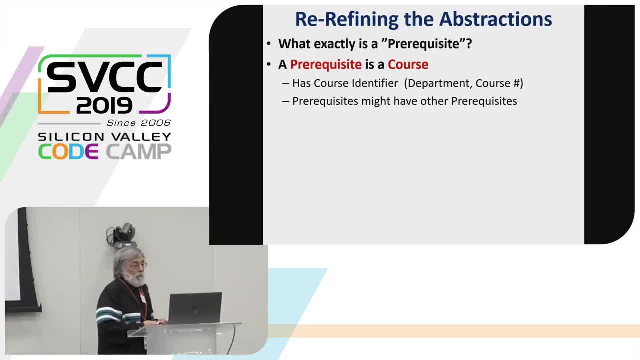 Probably the prereq is a course. Prereqs might have other prereqs: Cool CS3 might have CS1 as a prereq, and so on. So it's going to be a course. No, it's not right. 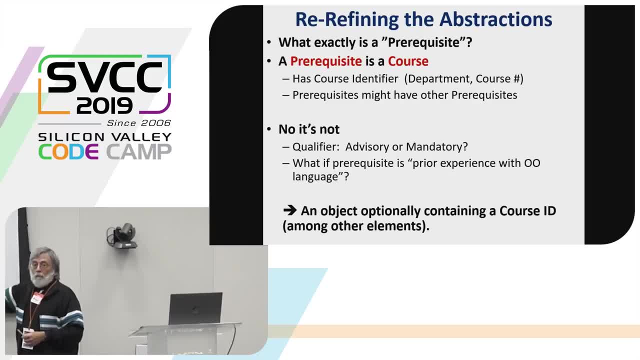 Because the, if you look at most catalogs, prerequisites are either courses or- and they could be advisory and mandatory. You've got to have this or you maybe need this. It would be good if you had it And in fact they can be text strings. 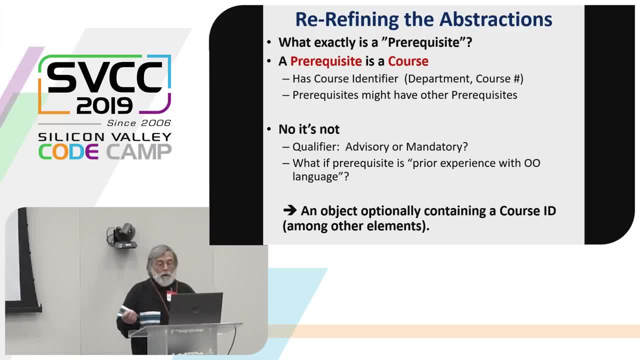 You can either have this course or you can have some prior experience with an object-oriented language. So what a prereq is when you think about it in this particular application, thinking about the application and how it's going to get solved, a prereq is probably an object optionally containing: 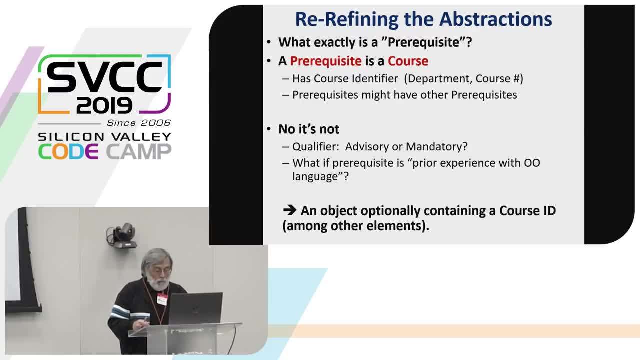 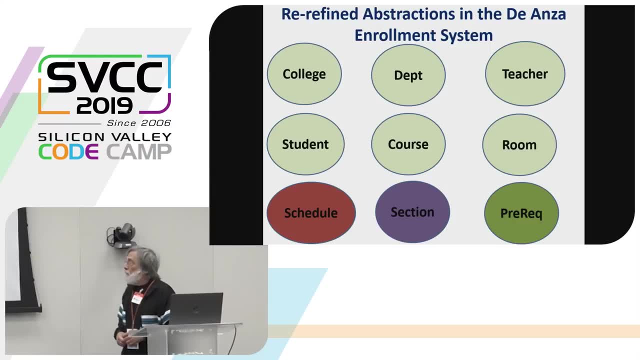 a course ID, among other elements. So we're now at nine. Just in terms- whoops, sorry- Just in terms of thinking about the enrollment and the fleshing out and creating sections. we've now got nine objects that we thought about. 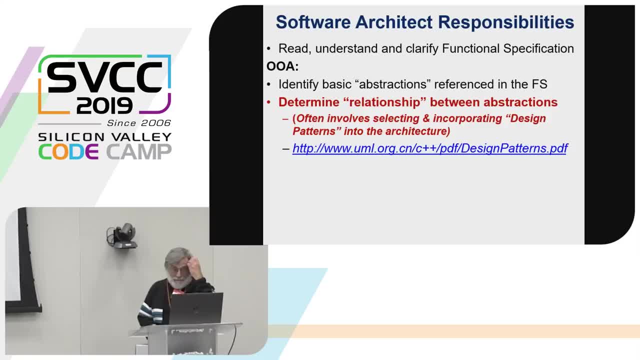 And so the second piece of this- determine the relationships between the abstractions- often involves selecting and incorporating design patterns. This URL, it's a marvelous URL. Nobody in my class is on it, but I get the feeling here. people have- how many people know, have heard of the gang of four. 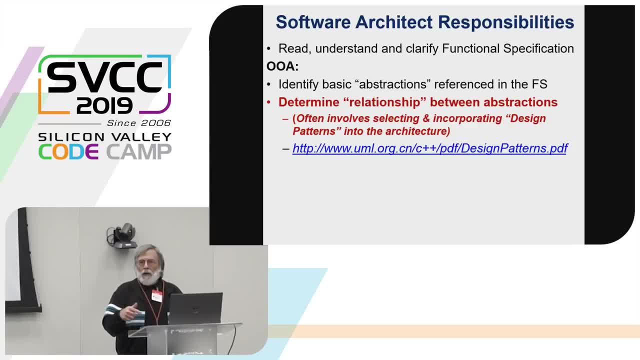 Okay, how many people think that was China right after Mao? No, okay, okay. There's a second gang of four. okay, It's the gang of four who wrote the book on object-oriented- well, actually on design patterns, who took the collection of designer successes? 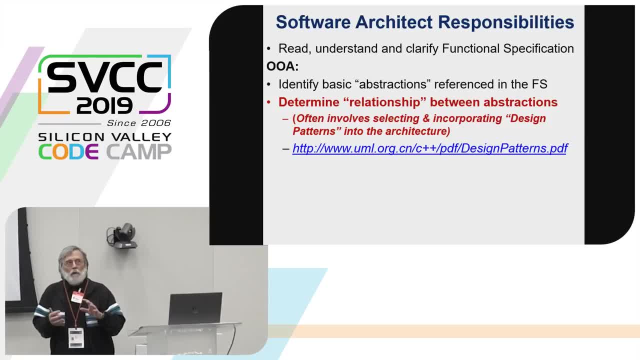 and found a formalistic way to define them so that they can be reused easily. Now the book the gang of four book was a landmark. You don't have to know the contents but you really want to know the index, Because the index tells you what's there. 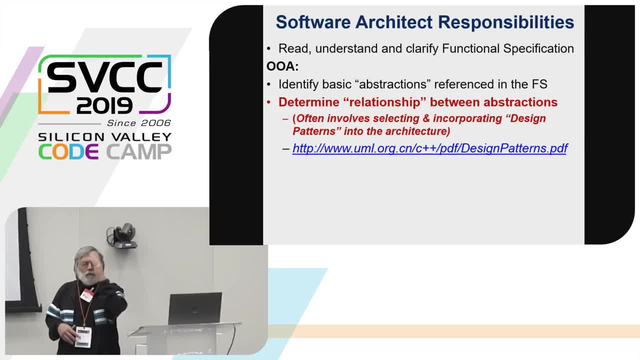 And if you need it, you're going: oh man, I've got all of this code reduplicated And you look and there's the pattern that says: why don't you put it refactor and get a separate object and put the code in there, and so on. 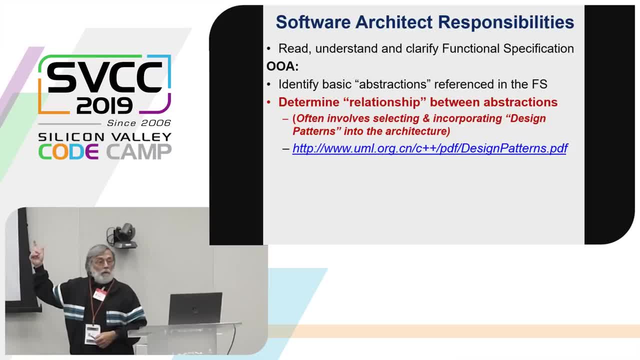 So this is free on the web. It's a PDF file now. It's really cool And I would urge. if you're serious about programming, this is the original one. There's a lot more, because every grad student wants to get his own pattern. you know her pattern. 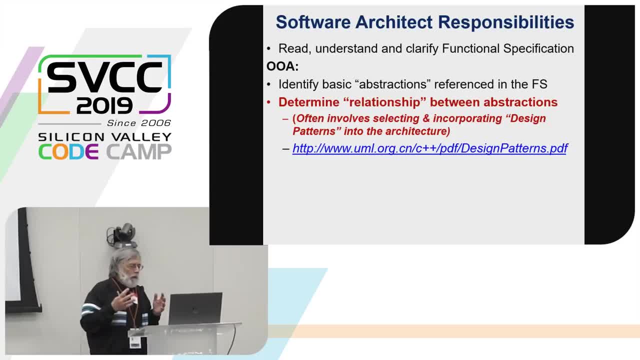 But this is the original. These were the ones that were felt to be important. Again, if you're doing something specific, like you know, the cloud or something, there's books on cloud patterns and so on which are going to help you think about. 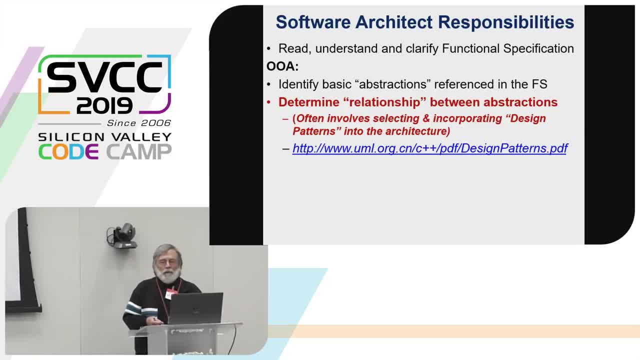 reuse the thinking of those that come before. It's very much like in science. they always say: you know, I stand on the shoulders of the generations that have gone before. In programming it's more like I stand on the feet of the generation that have gone before. 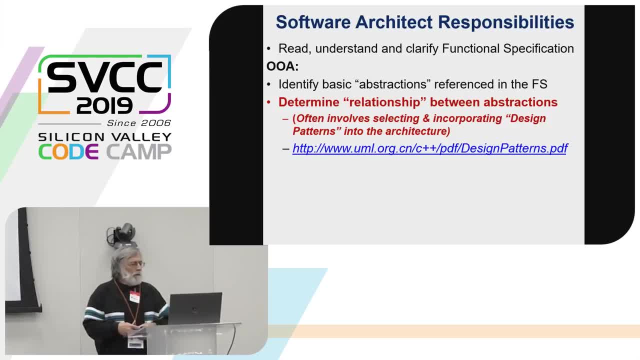 and you're always. you don't get up very high and you're always tripping and falling over each other, But design patterns are supposed to be the way that you really do reuse the thinking of others. So this is a diagram. It's the conceptual class diagram. 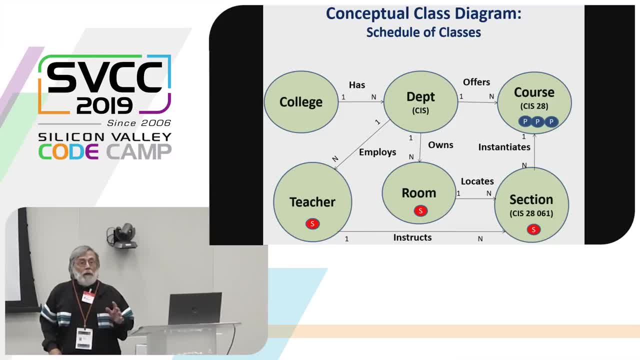 It is a UML diagram And if you're starting an application, in fact, if you're coming into a company that has an application, this is the thing you want to look at. Yes, This It probably does. You know the people that put together. 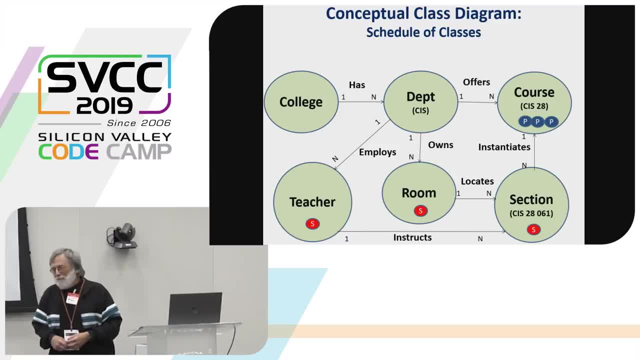 the unified modeling language, were using the work of the people that had come before them. This, but in this particular diagram, if I was starting work at the company that was making enrollment systems and so on, this tells me kind of what I'm dealing with. 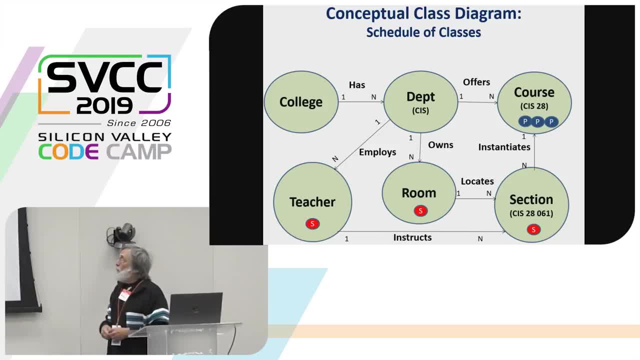 One college has n departments. Each department employs n teachers. Teacher tends to be employed more for the department than the college. Each department owns rooms. Sometimes they don't. Sometimes the rooms are owned by the college, But in our particular case we're going to find out that that's true. 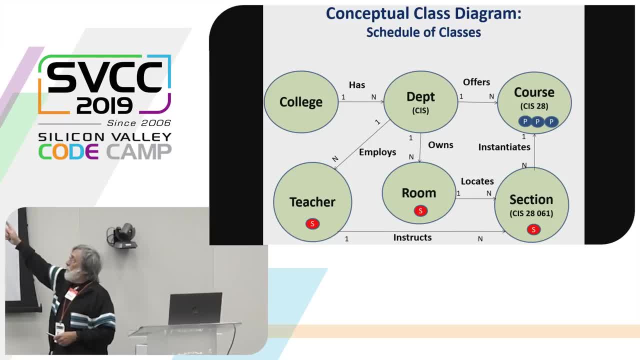 Each department offers courses. Courses may have prereqs. Each course is instantiated. They're initiated by n sections And notice section room and teacher incorporate schedules And if you look at this it's an overview and one teacher instructs multiple sections. 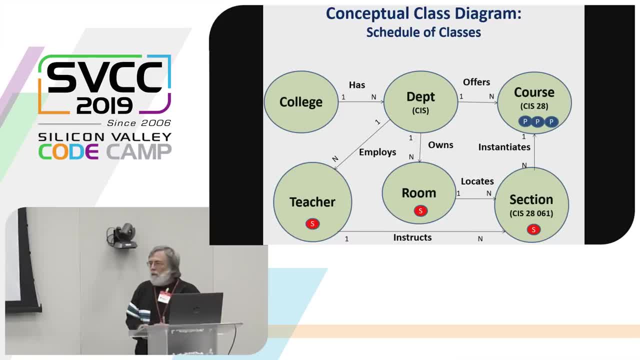 Now you could say: well, maybe it's team teaching and stuff and there's a little bit of arm waving here. But in general, if you're trying to get your mind around what it is that the application is doing and what are the basic abstractions, 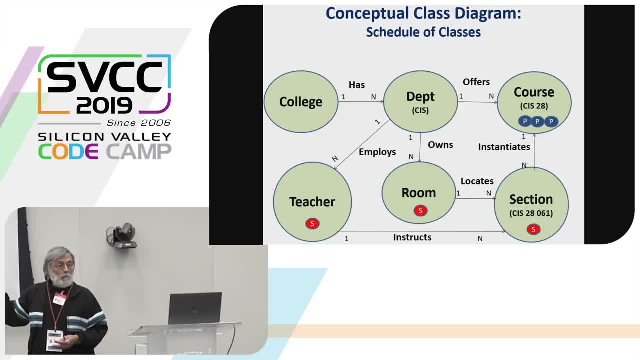 that are going to be manipulated. this is not a bad diagram. How do you designate if a room can belong to more than one department? Well, we don't here, And this is the high-level conceptual. And now again where it gets interesting. 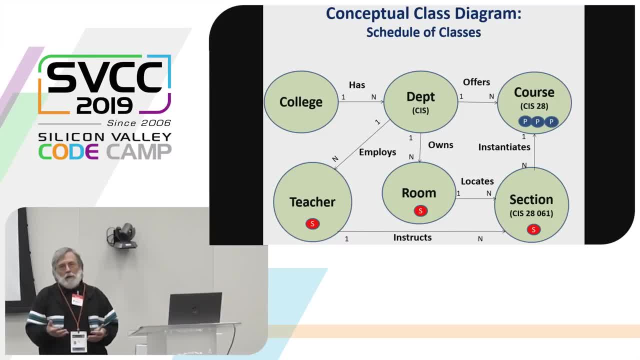 is. let's say that we are all this is a company meeting of the enrollment. you know, we are enrollment company right And we sell these things And your point is well taken. We've sold it into three colleges. And now the fourth college says: 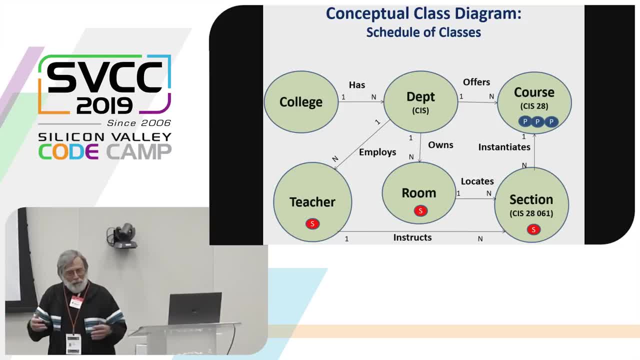 well, wait a minute. We allocate rooms to multiple departments, and how is that going to work? And we have to think about that. Yeah, stuff moves right, It's not. this is just in our simple case, Because we could clearly spend a day. 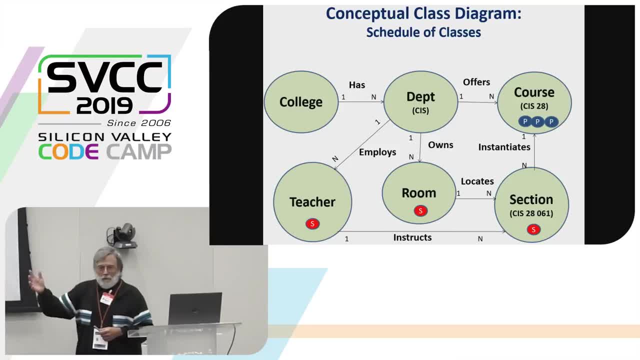 refining this with all of the things, But conceptually this is at least the first pass. If you came in then, at least you now, because look at what you did. You looked up here and you said: I don't think that fully reflects. 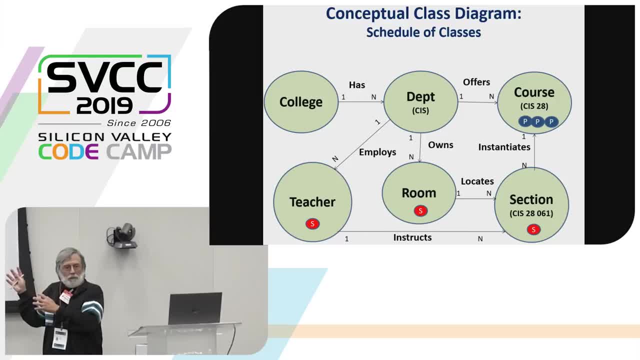 a requirement I have, But at least we've all got the same thing to shoot for. We're all talking about the same you know description of what the problem is, So the question was for the people that couldn't pick that up. 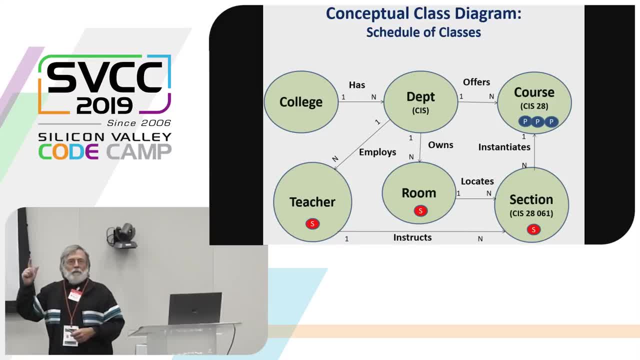 on the video thing. the question was: it makes sense to the domain expert. You can show this to the registrar and he or she can look at this and say, yeah, that's right. And if, in fact, you said something like: 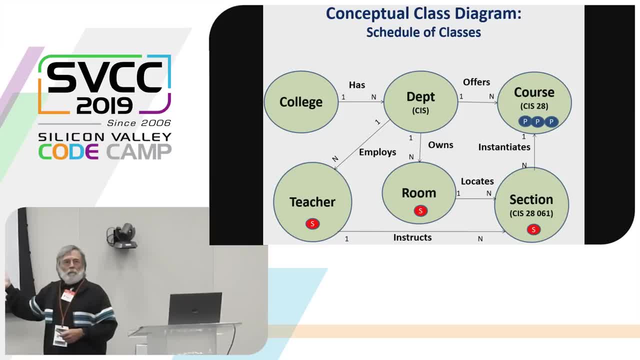 well, you know, we have some sections that are virtual. okay, and you're now. so you're looking and saying, great, we're going to have a virtual room. that's always free. And the point is, you can take the requirement that. 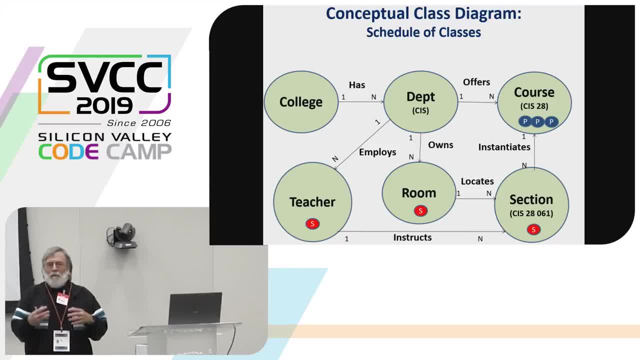 the registrar has the right to say. the registrar has said, and you can map that into the particular object or objects that are going to be affected by trying to meet that requirement, because you're thinking about the problem in the same way that the domain expert. 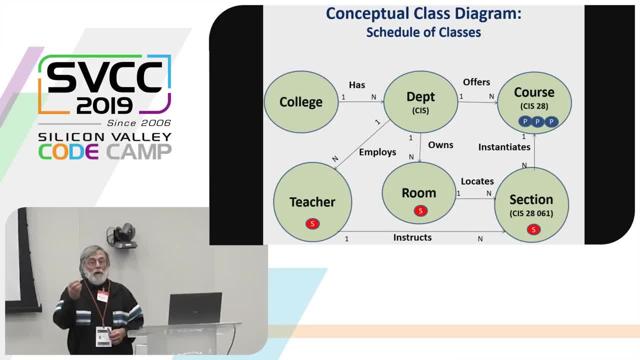 is thinking about the problem. That's the key thing. It's why, if an architect for a house, you know, if the you know, if the user says, you know, and I want an aquarium in the bathroom, well, you kind of know where the bathroom is. 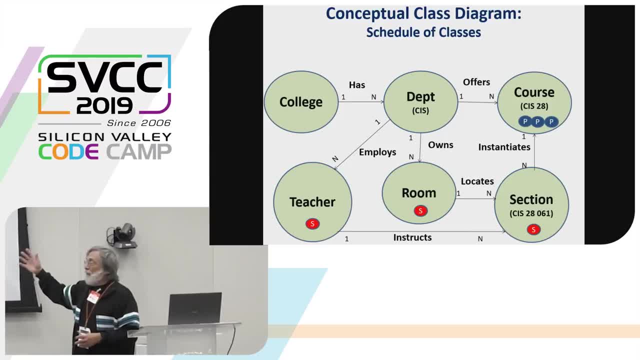 and you kind of know where an aquarium is and now you start. but the point is, that's kind of what this is, And requirements change Right. there's one of my favorite cartoons, which I had hanging over my desk for a couple of years. 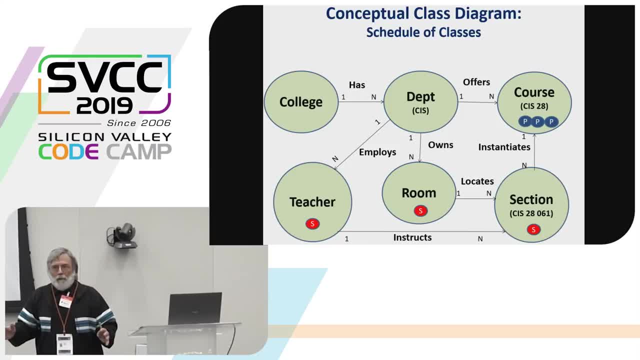 was it was. it's ancient Egypt and there's a pyramid and it's not quite filled. it's huge in the distance but the top is still not quite done and there's lines of men in the distance heading toward that pyramid. 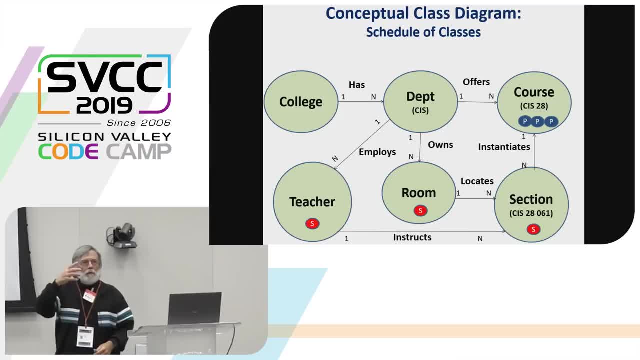 and going up the sides to fill it in. and there's a gentleman standing on a hill overlooking all of this and he's got a megaphone and he's screaming into the megaphone: stop work. there's been a small. 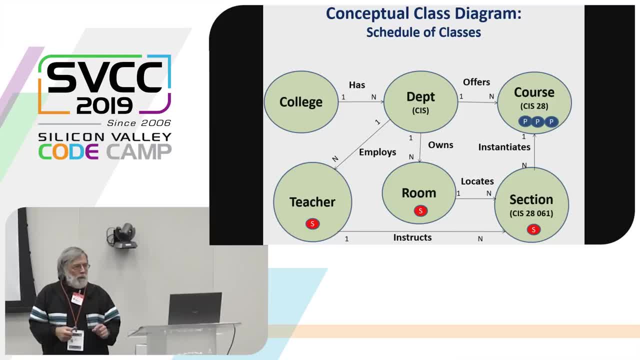 change of spec. the pharaoh wants to be cremated. Okay, now that's an example of a rather a larger change of spec than we normally see on these things, but your point was valid. Well, you know what if you had virtual sections? 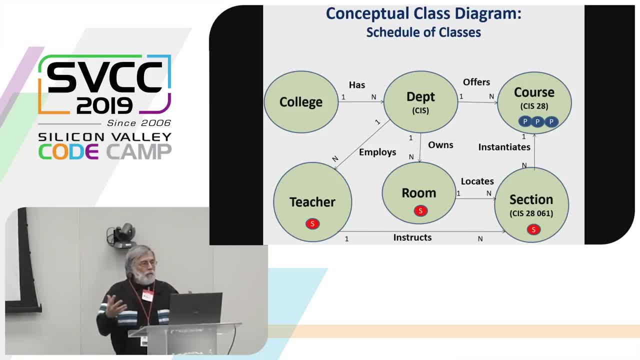 what if you had rooms that are shared? what if you had? and you're trying to expand your application, but conceptually, at the top layer, this is what you're seeing. Yes, Yes, I can. So the arrows typically. 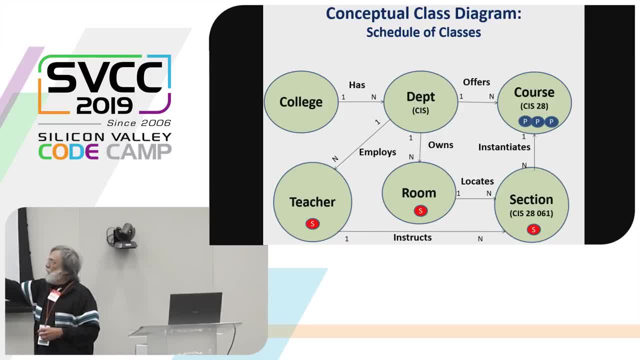 the way the arrows work is. the arrows indicate how the word applies. So one room locates end sections Right, but here end sections instantiates one course. Had I said instantiate by the arrow would have been the other way, Like one course is instantiated by end sections. 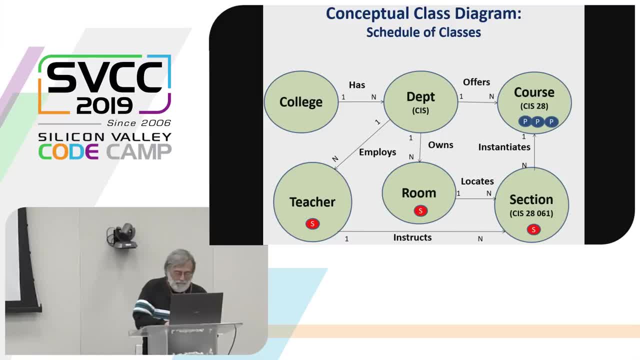 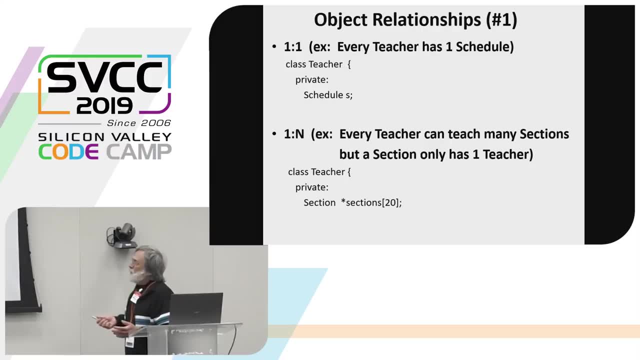 Yeah, Yeah, sure. So relationships, If a relationship. and these are some C++ coding examples, but they're very small. it's not necessarily that you need to know how to write C++ code, but you should know how to read a couple of lines. 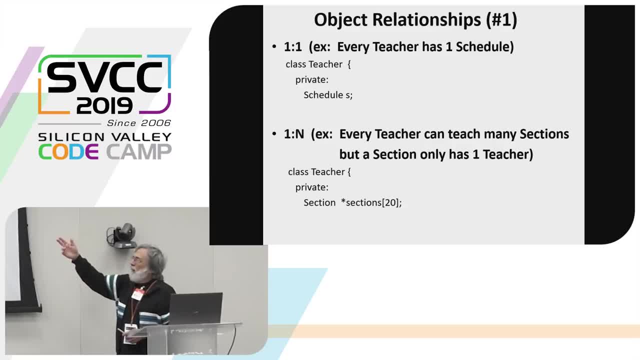 So this is class teacher and inside of class teacher is a private schedule. object: That's a one-to-one relationship. Every teacher has a schedule, One-to-end like. every teacher can teach many sections, but a section only has one teacher. 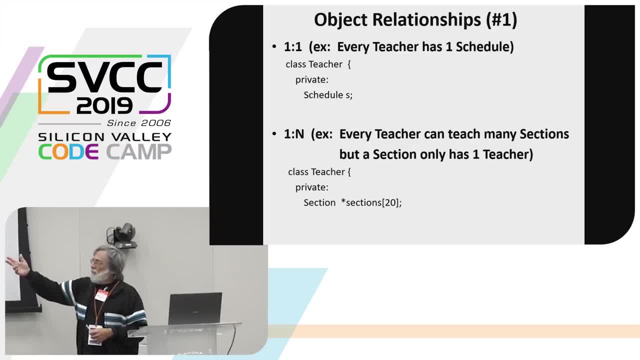 So in this particular and simple case, you have a teacher and it has. every teacher has an array of. this is really bad code. has an array of up to 20 sections And basically has an array of up to 20 section. 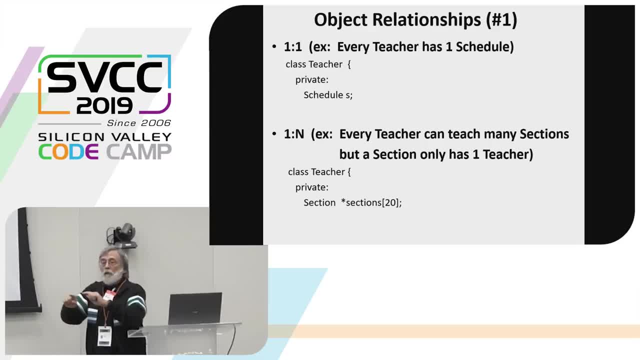 pointers, because the teacher object isn't going to contain the sections. It's going to point to 20 sections that the teacher might teach. One teacher end sections. what you're really saying is: a teacher has a collection class of sections. 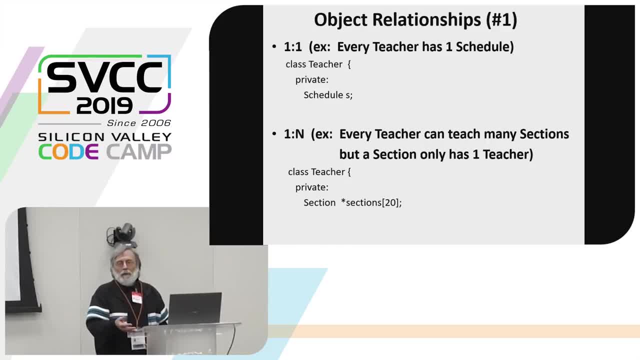 And the collection class, and it depends, and if you're the architect, you'll specify right. There's the vector, which is everything that an array always wanted to be when it grew up, You know. there's hash tables, there's 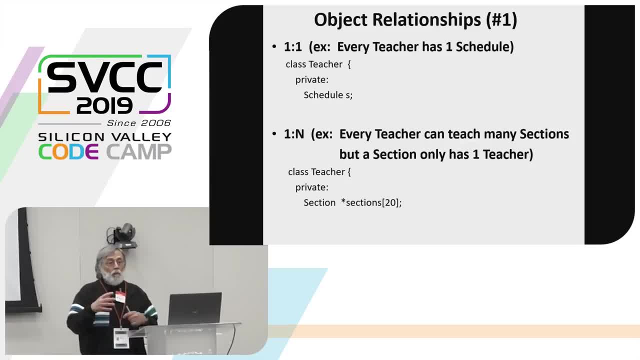 a linked list. there's queues and stacks, and these are all ways that one thing can collect other things And the architect will determine. and there's, you know. if we had another hour we'd talk about the appropriate use of collection classes, But 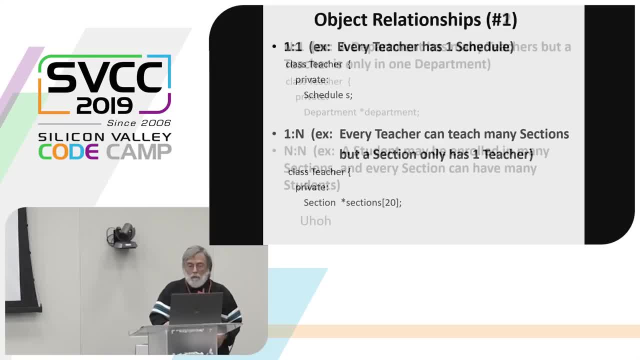 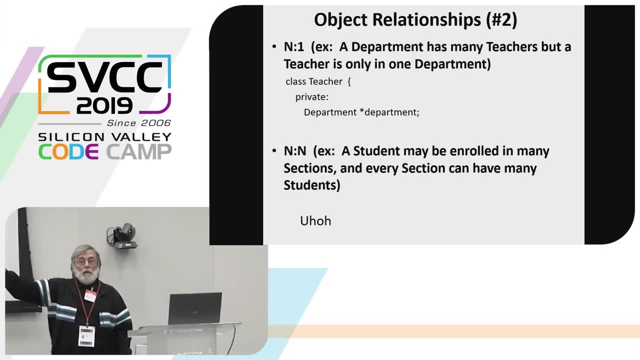 this is one-to-end right And to one is, in this particular case, every teacher end. teachers point to a department, So if the department name changes and that at the end of the answer may be happening, we may be going from CIS. 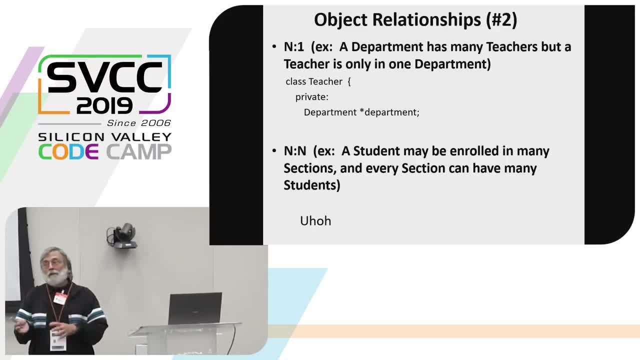 finally to CS, from computer information systems to computer science. If we did that, it's not like every teacher would have to. every teacher would see that immediately because teacher points to department and department names change. so if you ask the teacher, what department are you? 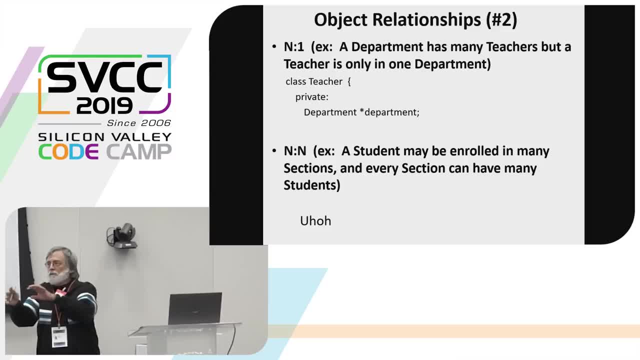 you change the name of the department and you don't have to run around in all the teacher objects and change the name, because you just end things with pointing to the same thing, And that's an example of end-to-one, End-to-end. 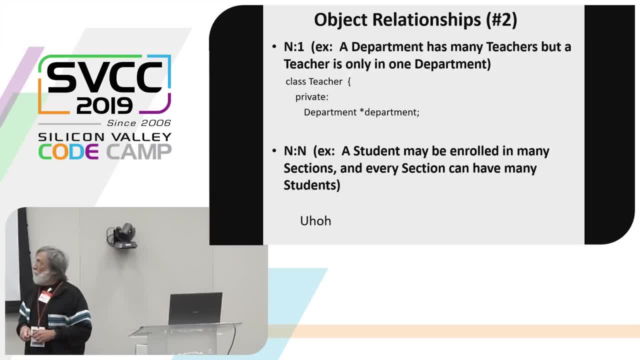 This is the bad one. A student may be enrolled in many sections and every section can have many students. So if you're a student, you're enrolled in five sections one-to-end. If you're a section, you have 40 students. 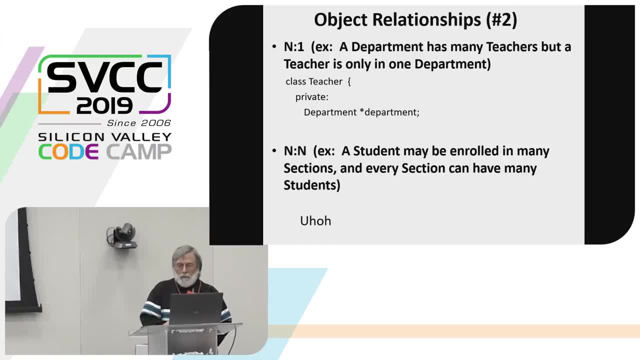 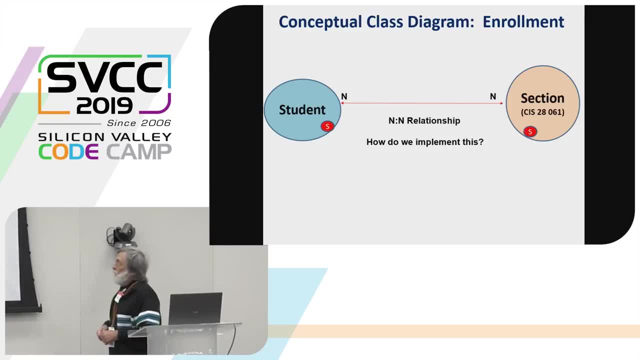 that's end-to-end. That's called the uh-oh inter- relationship. And here we are: You have a student and it's got a schedule, and you've got a section that's got a schedule. it's an end-to-end. 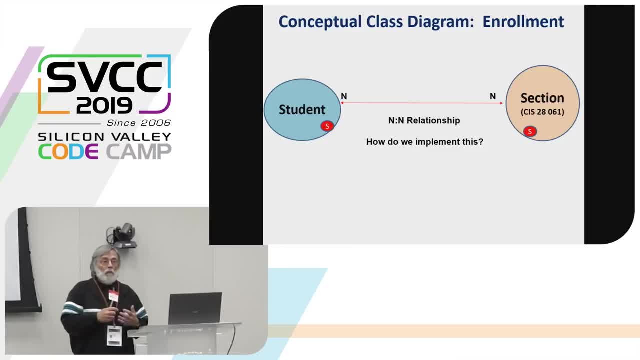 relationship, One student and sections. Every section has its students. How do we implement this? Well, the first thought is: why not? why not have arrays of pointers, just like we did before? So you're a student, you point to all. 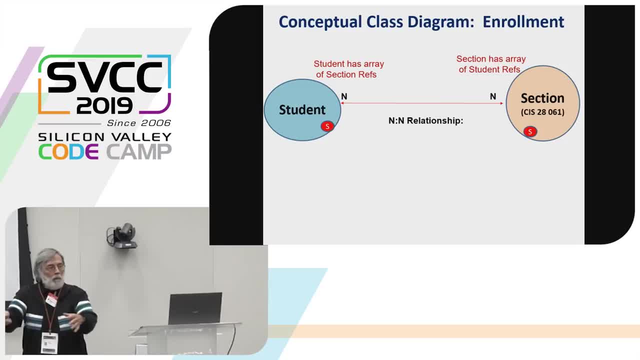 of the sections that you think, and if you're a section, you point to all the students that are enrolled, and if you're a programmer, you're done, And if you're an architect, you're not done because you're thinking about it, right. 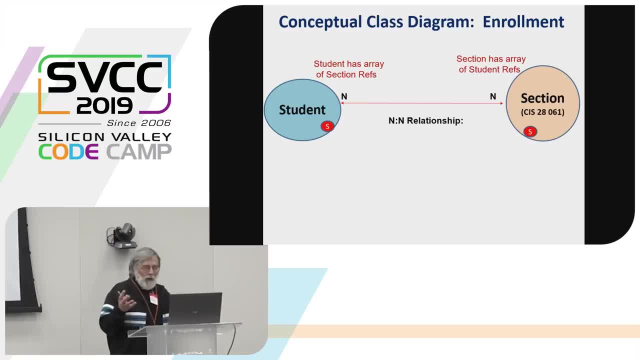 And you're saying: well, wait a minute, You solve the problem for inter-relating end-to-end. but this problem's a little different, Because each relationship has its own data. So if you're a student in a section, you have. 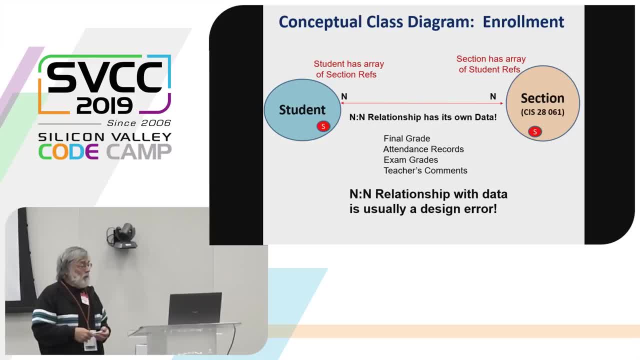 a final grade that's assigned, You have an attendance record, You have exam grades, You have teachers' comments, Works and plays well with others. I don't know. The point is, all of that goes along with your relationship to the section. 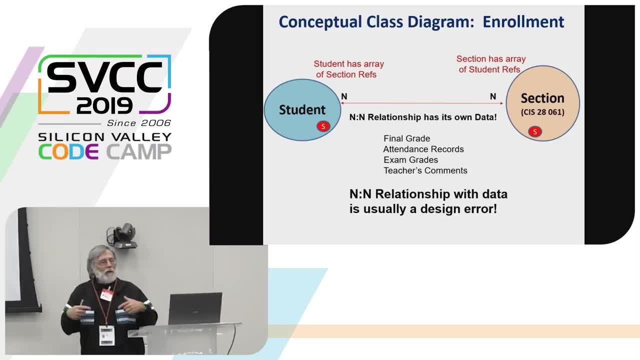 Now the arrays. where do you carry this information? If do I carry it in student, Do I carry it in section? for each one of these, For each student in a section, I have this. Or for each section that the students take, I have that. Or, worst of, 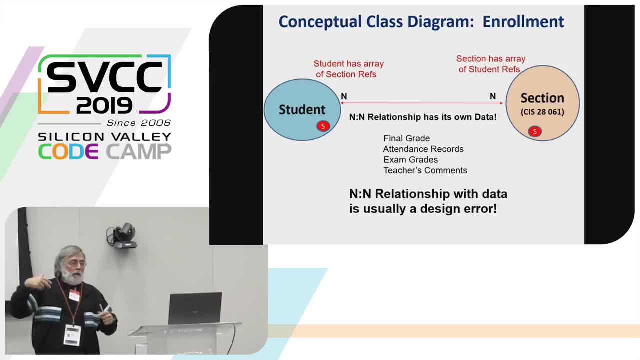 all, do I have it in both places, Right, And you're thinking I have an end-to-end relationship with associated data. What am I going to do? I'm probably the first person in the world that ever ran into this, And you slowly. 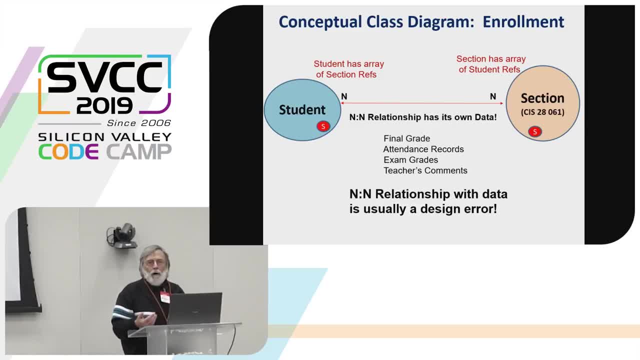 think, wait a minute, wait a minute, wait a minute. There's probably a design pattern. So you go to the gang of four or whatever you're using for your thing and you say, ah, A junction class puts something in the middle. 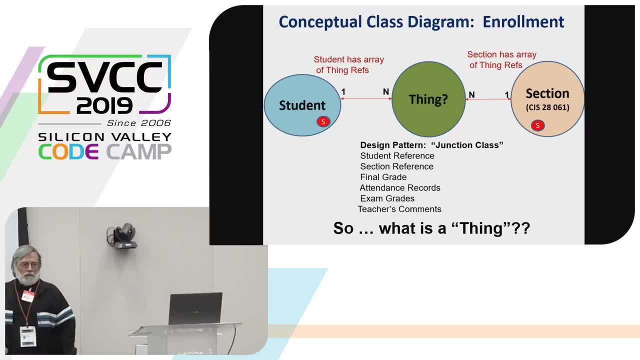 So you know, every student has any of these things And every section has any of these things, And this thing, whatever it is, has a pointer to the student and a pointer to the section, because it's an end-to-end relationship with both of them. 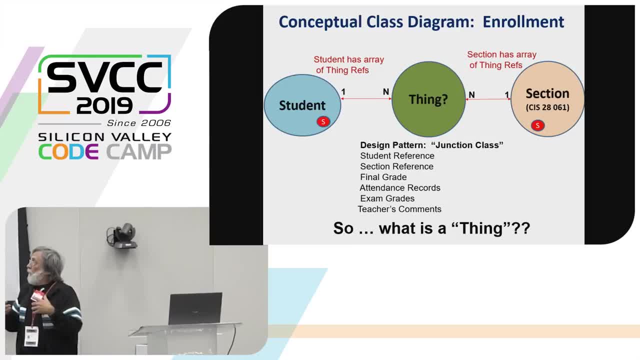 And it has the associated data of the relationship. So one student can walk through these things and find out everything for every section it's in it now can find out. okay, I can get the section to find out, the section information, and I can also. 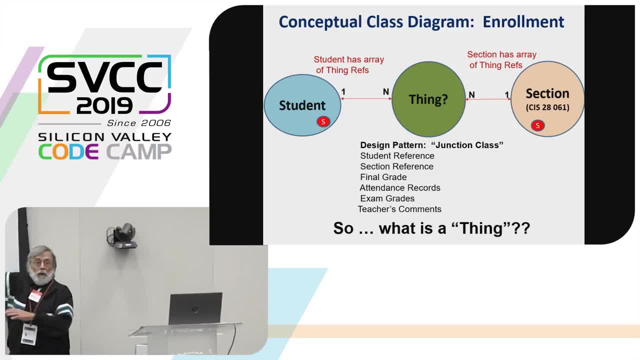 find out how I did in that section. And every section says: okay, for all the students that I've got, I can come in here and find out what their grades were and I can get the name of the student And we solved it. The question is: 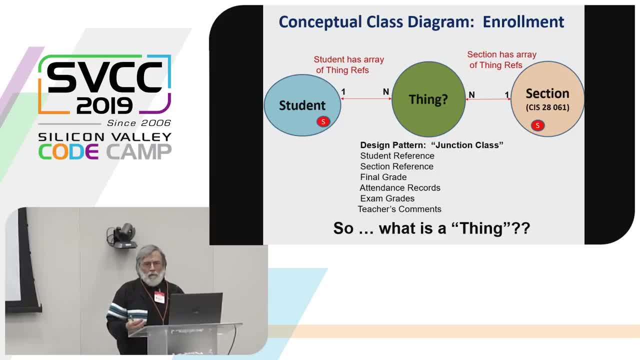 what is a thing? Let's talk about that. So someone said it's the enrollment. But the problem is enrollment works for the section And in fact enrollment is probably the name of the collection of these things. You know, if you have. 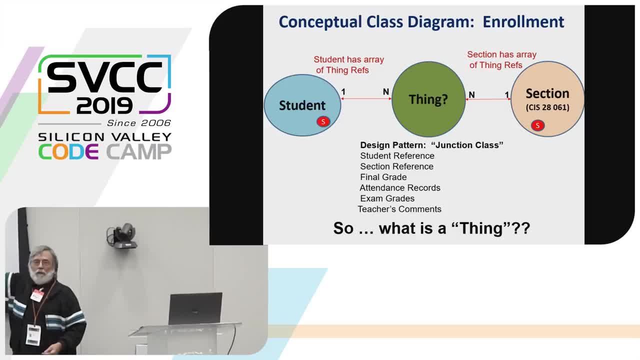 40 students enrolled. right, each one of these it's an enrollment, But the- yeah, I mean it is, but typically enrollment is the collection of- I mean it's not bad, but it's the collection of all of the students. 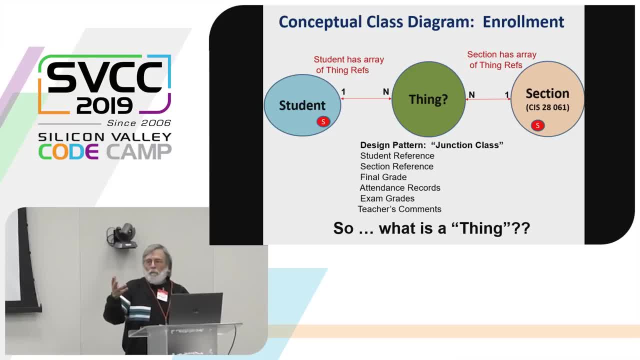 in a section is usually what enrollment? is A data table, Meta table? So you could say every student has N meta tables. You know, I mean you could right, but that may be how it's implemented. and particularly, are you a database? 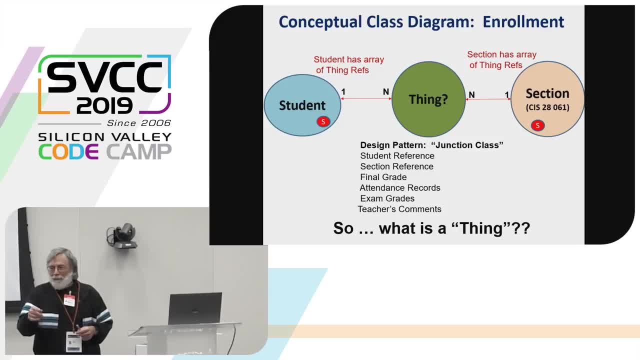 guy. Okay, that was a lucky guess on my part, because meta tables typically, I mean that's, there is a different thinking between database people and object-oriented designers, Because the databases, you know, they're into junction, junction, but anyway they're. 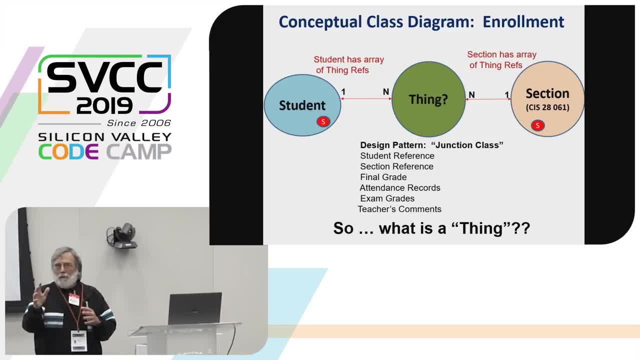 different And sometimes you trip over it. But that I mean because metadata, in a way it may apply, it may not apply, but that's not the name of it. You're looking here for the thing that binds. yes, 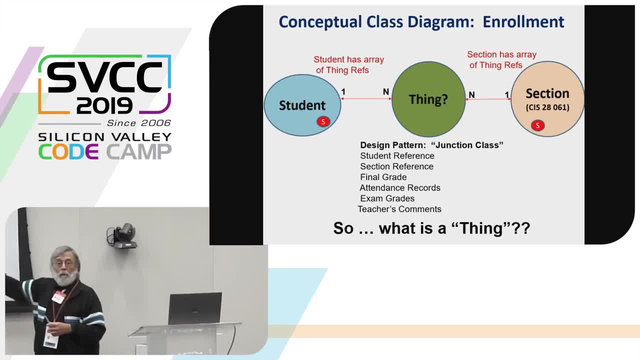 I was going to call it an array, The word grade, and a grade is just a part of this. A what It is, It is and yeah, right. and if you're an architect, people always say: guys don't. 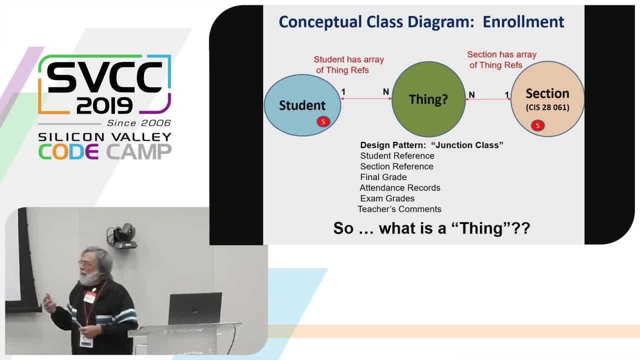 understand relationships. Well, if you're a software architect, yes, you do, You know. But yeah, but I mean that wouldn't help. It's like because what are you going to say? You're going to say to the domain, to 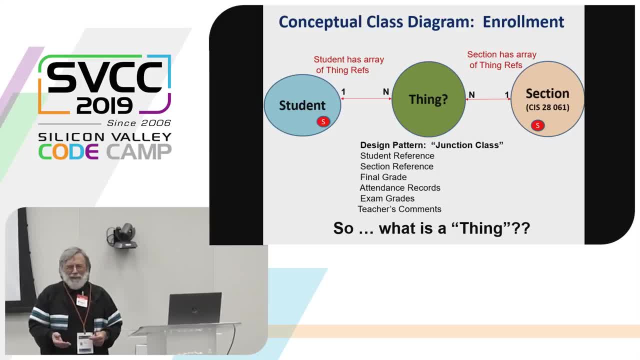 the registrar. every one of your students is involved in many relationships. You know it's not what you want. You want to say something to the registrar that's going to. you know he or she is going to go. yeah, okay, I. 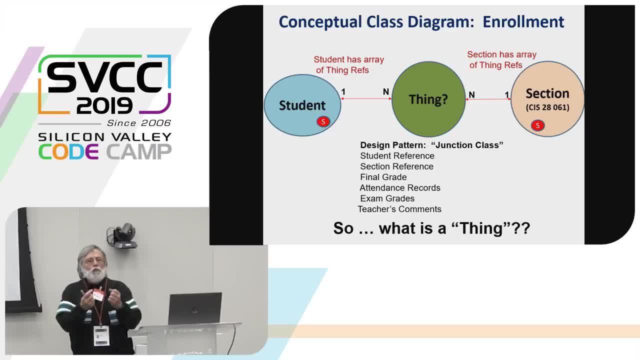 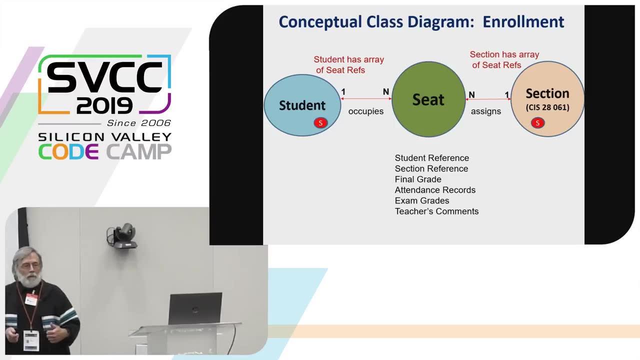 get that? What binds you to every section? you ever sat in Hint Dollars A seat. If you, a student, occupies N seats and a section has N seats that gets occupied by a student and every seat says this is the student. 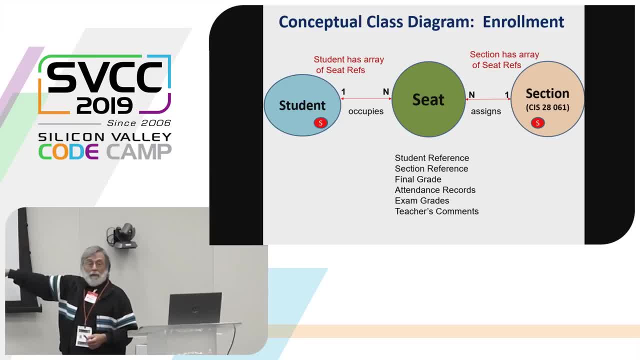 that's the section. that's the final grade. you got in that seat. That I mean. the point is. I guess the point here is you had the junction set right, but it's, if you can find a name, that absolutely nails. 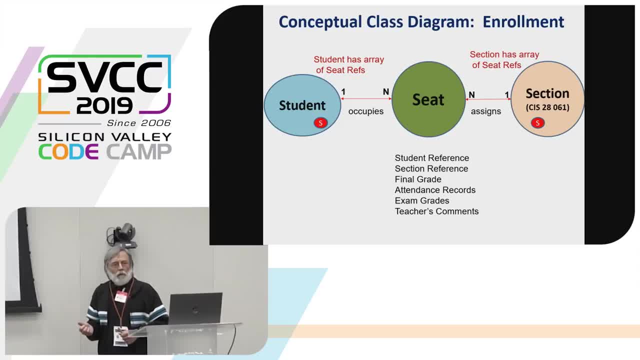 what this abstraction is. you're way ahead of the curve, Because this is something that the domain expert will, like the registrar will understand immediately. Yeah, we open up a section with 40 seats, 27 of them are allocated to students, so 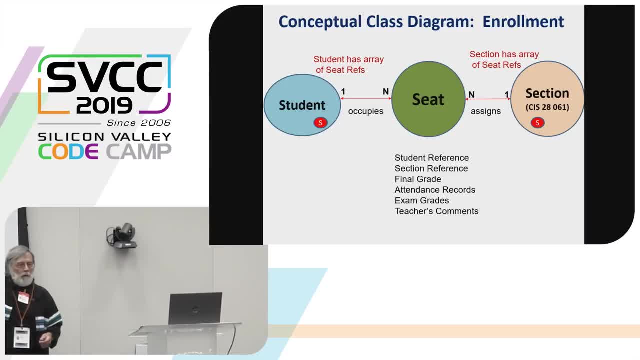 you've got the 40 seats, but only 27 of them have a reference to show that there's actually a student there, And again seat is a very useful abstraction. An example might be: well, you know, kind of you think of it like: 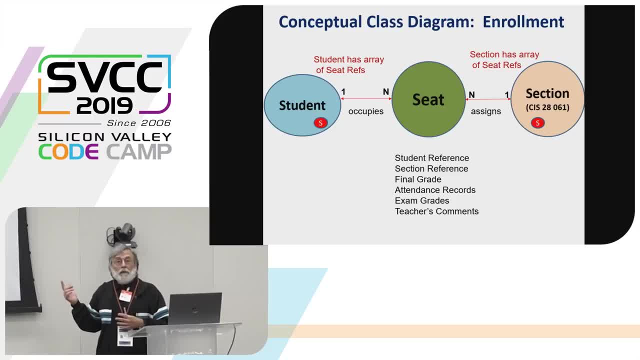 well, an airline right, an airline seat. An airline seat is very different than this kind of seat, because an airline seat has an identity. You walk into a room to sit down. you're just going to sit down in any room. 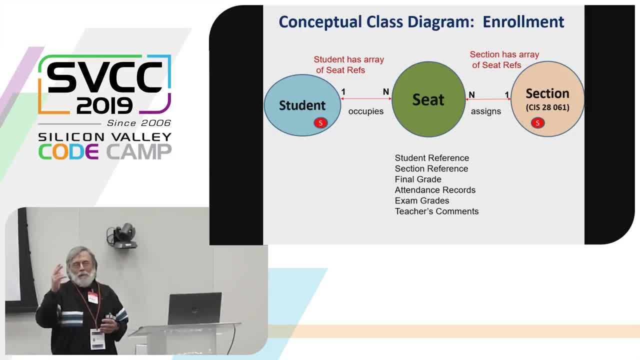 But that's not true on a plane, unless you're flying southwest. But so that's a difference. The other difference is you know how many of you are in a first class seat here. So the same name, the same seat name, but 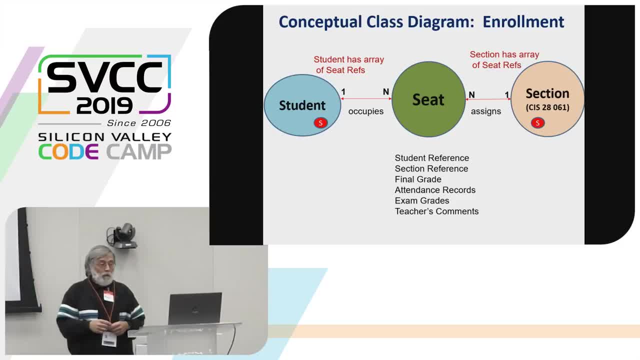 a very different abstraction. We need to define what a seat is, And once we do that, a lot of the problems we had go away. We used the design pattern and we've now got a new abstraction, And so guess what We're now up to. 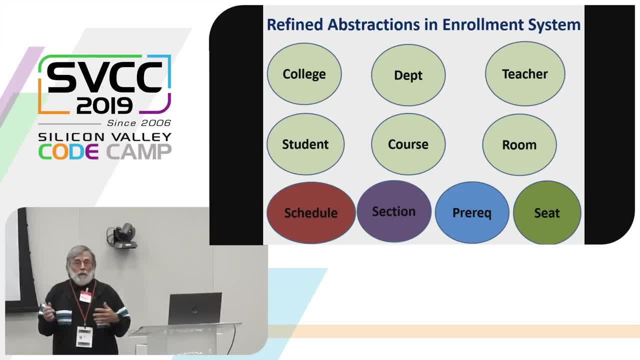 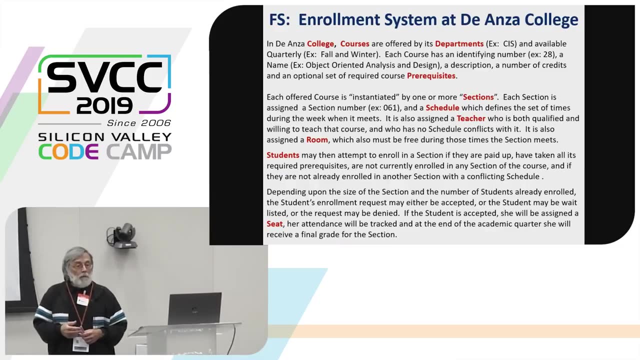 ten. We originally had six. We've thought about how we're developing things and we're up to ten, And so now we go back to the functional description and we put in our abstractions and we go back to the registrar. 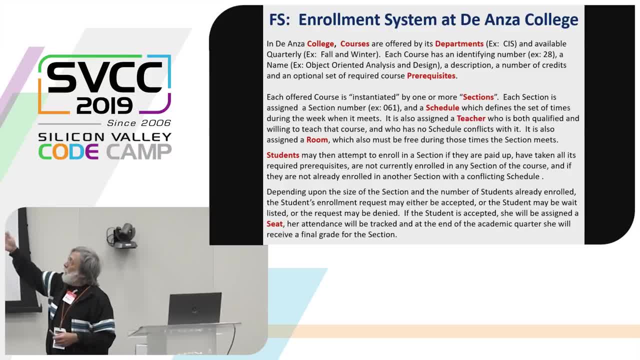 and we say: this is what we're solving In the hands of college. courses are offered by departments a set of prereqs. each offered course is instantiated by one or more sections. Each section is assigned right And it has a schedule. 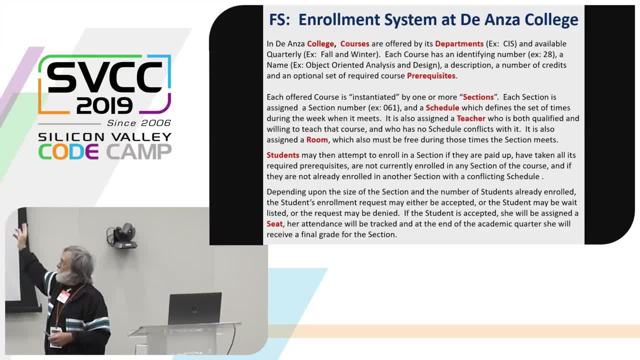 which defines a set of times. It is also assigned a teacher, and so on, and so on. It is also assigned a room. Students may then attempt to enroll in a section if they are paid up, and so on, and so on, Depending upon the number of students. 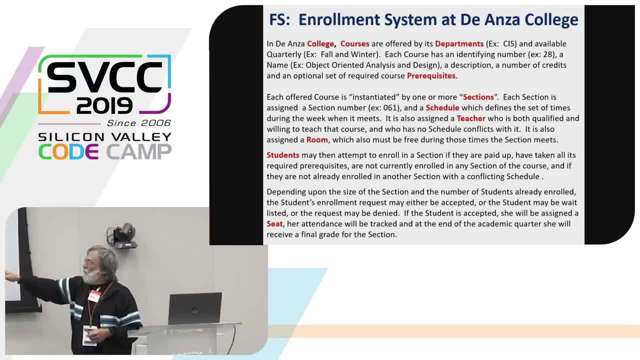 it may be accepted, the student may be waitlisted or it may be denied. If the student is accepted, she will be assigned a seat. This is the same description, except this is now a description that we can implement because we have an idea. 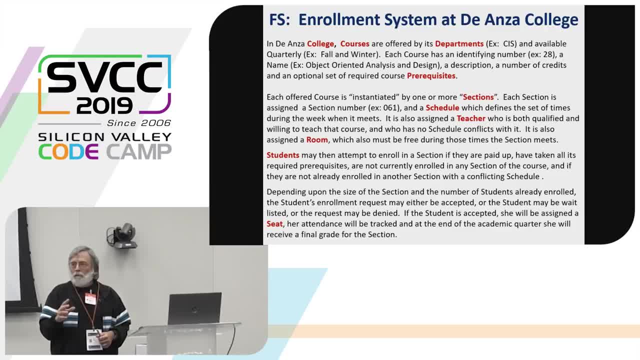 of what the abstractions mean in terms of the application that we're trying to solve. It's the first step, because typically you get a functional spec and you're going: I don't understand it, I don't understand what this means. 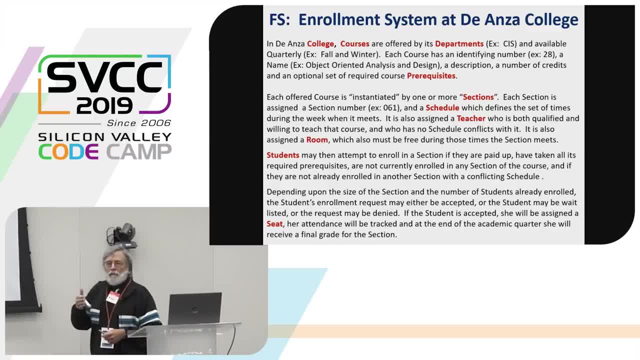 I don't understand what that means. So the first step is at least getting the functional specification defined using words that you understand how to build and use in solving the application. Yes, sir, Could you also leave the notion of a quarter? Yeah, maybe. 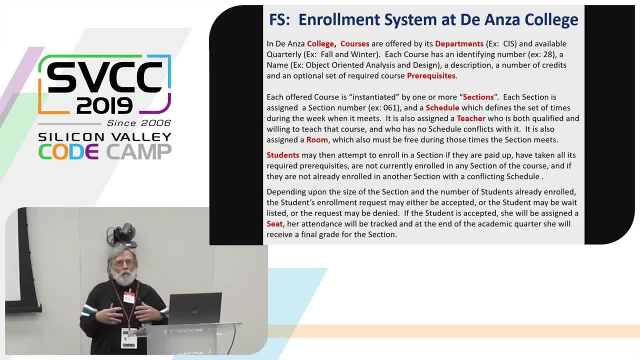 I mean a quarter is. my first thought would be to say a quarter is an enumerated variable that has four values: summer, winter, spring and fall. And I'm not sure what else it has with it, at least as far as enrollment goes. 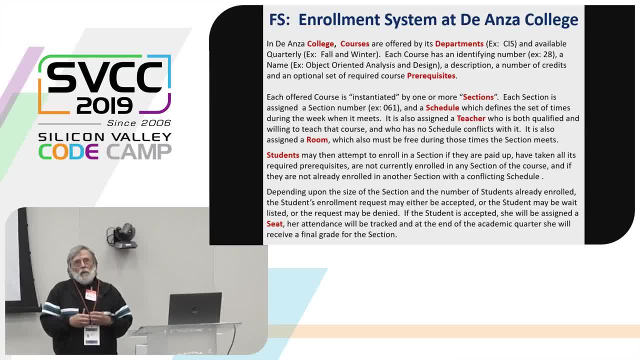 For example, you have a list of courses that are offered in that quarter. Yeah, you could have that, And that might be a division. Or you might just say I don't need that because every course indicates when it's offered. So typically it depends how you're looking for it. 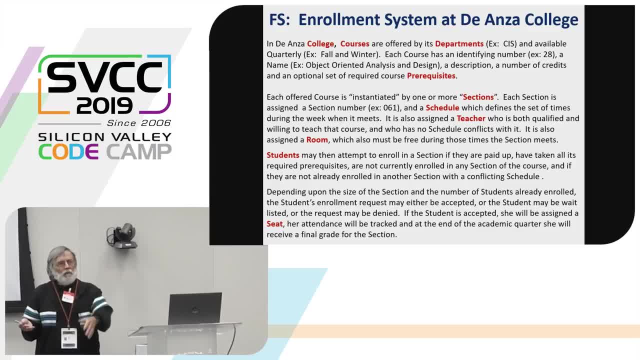 If your average user is going to come in saying what's available in the fall right, as opposed to saying when is this available? They're coming into a course trying to see That'll be the use cases and that will determine. 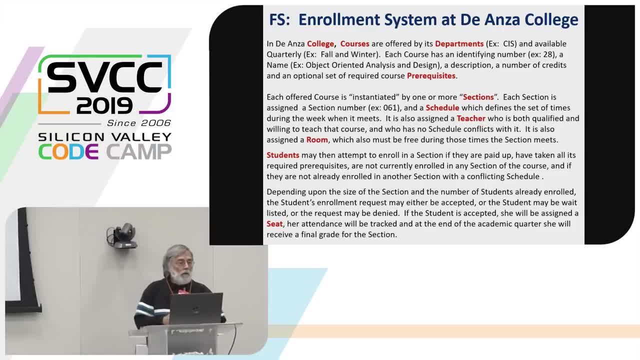 whether that object exists. Yes, sir, Do you use date-time as sort of a universal, abstract object? Sure. So the question was: what about date and time? Date and time are great objects because you encapsulate, because again it's like schedule. 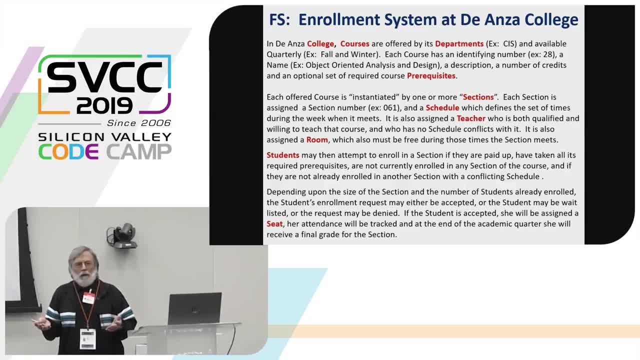 It's like: what do you want from a date and time? What do you want it to print out right? Guess what? Today is okay. no, it's not going to work today, But typically you see 4-11,. 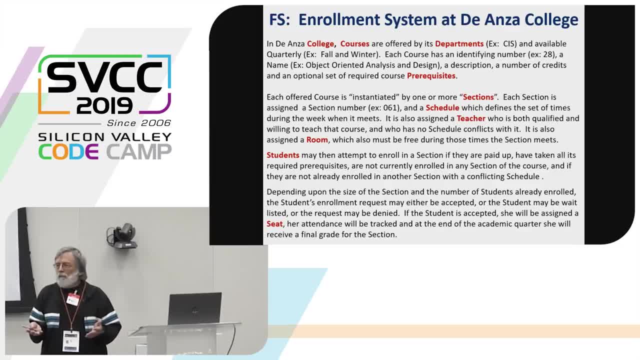 right, and we go: that's April 11th and every European says that's November 4th. So if you- because they do it differently, so you'd like your object to print itself out internationally, right, You'd also like: 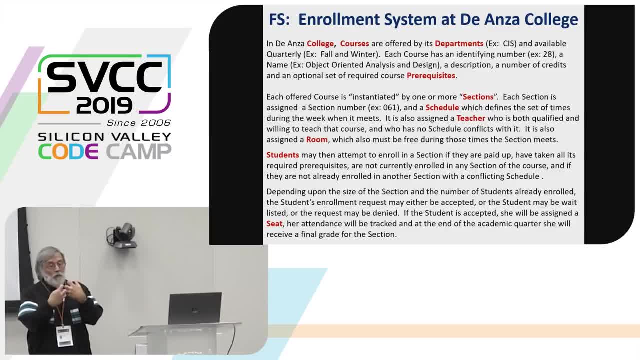 an object to say how many days between yourself and this other date object. There's all kinds of things you could want. so you're going to go down and you're going to, you encapsulate all of that and you now make the calls. 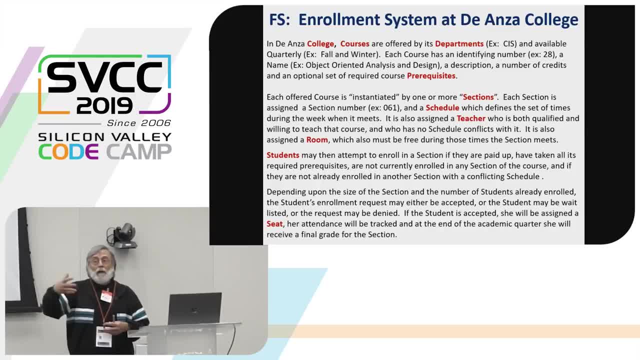 and you only have to do that once and it's in an object library and it carries over from application to application. Name is another good example of you know, last name, first name, what about middle initial? you know, and we've got to change the name object because 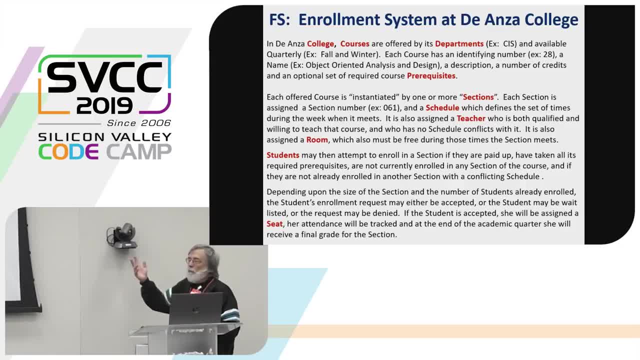 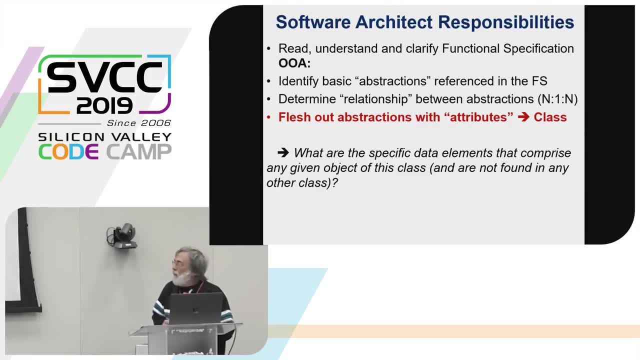 now gender can change. you know things that you hadn't expected. The point is, you encapsulated it and there's only one place where you have to deal with it. So you've got your basic abstractions and you know, you've defined them. you now kind of know. 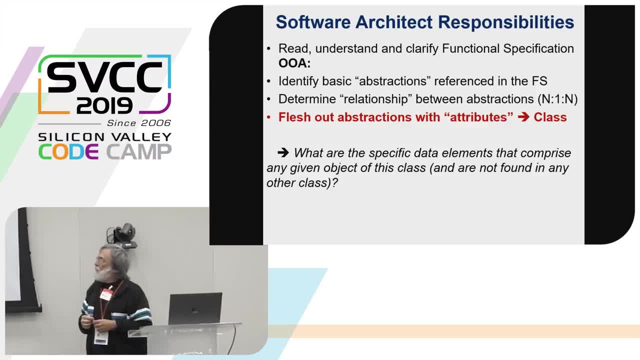 hey, they're n? n to 1, or 1 to n or 1 to 1, now you want to flush it out. So what you're saying really is: what are the specific elements that comprise a given object of this class and are not? 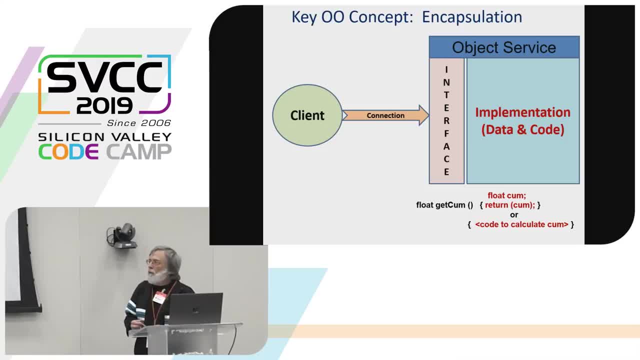 found in any other class, And this is key object-oriented analysis stuff. right, You have a client which connects in some way to an object, an object service, client and service. The connection can be. and, by the way, oh, there it is, it's just. 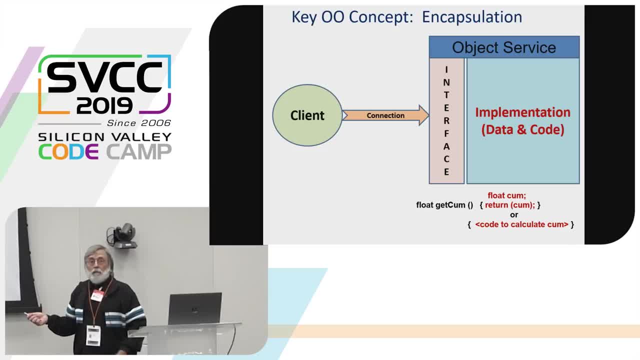 kind of hibernating. The connection can be anything from across the net to calling into an object library, to whatever The interface. again, if you're in sequence, plus plus, plus coder, or even if you're not, objects tend to be. 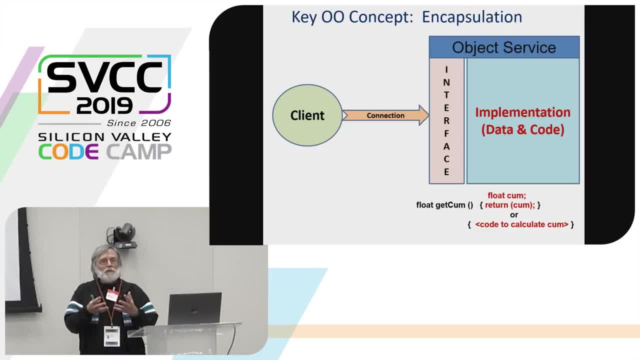 divided into two things. well, three things. One is what attributes, what physical elements do they manipulate? The second is the code to do the manipulation. And the third is the interface, the public methods that you can call, And the goal of an object is to 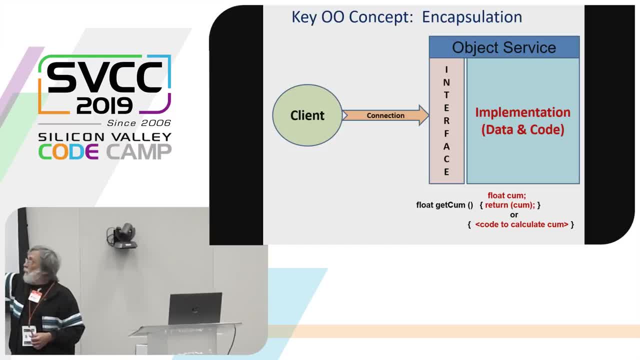 encapsulate the implementation, which is the data and the code behind the interface. So you're going to be defining, for every object that we looked at, the set of public methods that other objects can call to change, to affect and use the data. 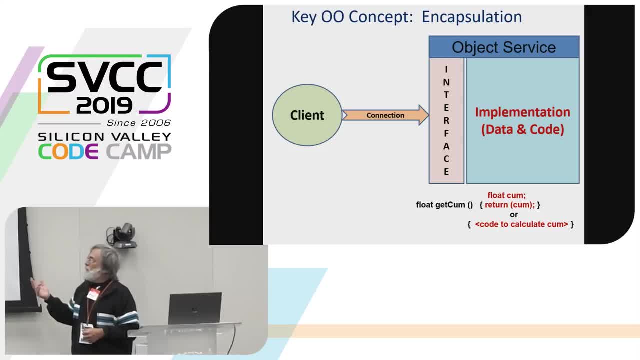 that's in that object. Encapsulation, because all of this, the implementation, is encapsulated hidden behind the interface, which means you can change the data and the code and as long as you don't change the interface, nobody else breaks. 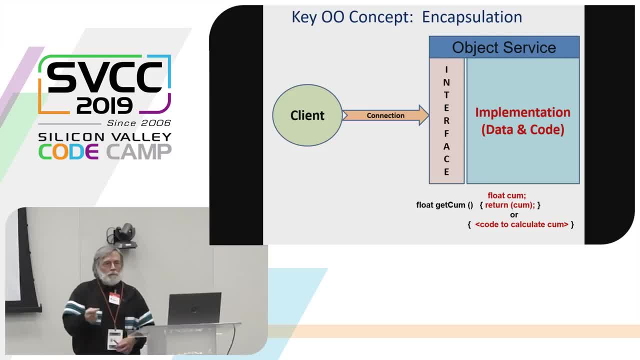 One of the design goals of object-oriented design is robustness, extensibility in the face of change. very easy to do that. One of the goals is not performance. Dirty little secret, right If you? because you're going to be calling methods instead of going. 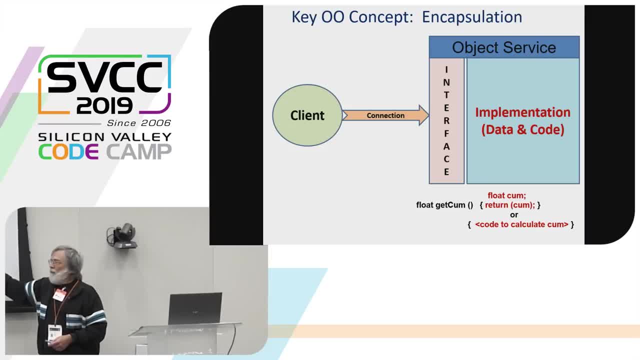 to get the data directly, And that means if your system's running too slow, you know, wait six months, there'll be a faster computer If your system can't be extended. that's the thing we're trying to fix. There was a question. Yes, 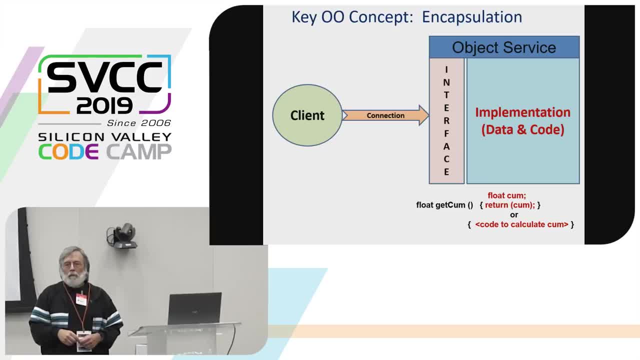 Audience Member 1. Audience Member 2. Audience Member 1. This is we gonna look. if we get how much time we got, we're gonna get to the point where we're gonna look at how this actually fits into a three-tier or four-tier. 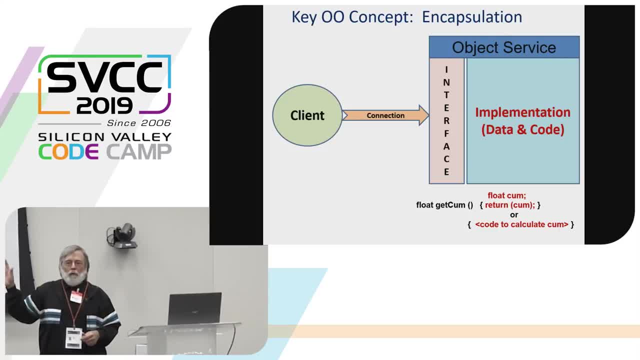 architecture. User interfaces are not what, okay, the the applicant- i'll talk to it in a minute- but the applications that we're talking about, pieces that are being designed like this. it's for when you say do it right, it's when you it's not to say i'm browsing all of the sections that are offered, or for that quarter, for example. 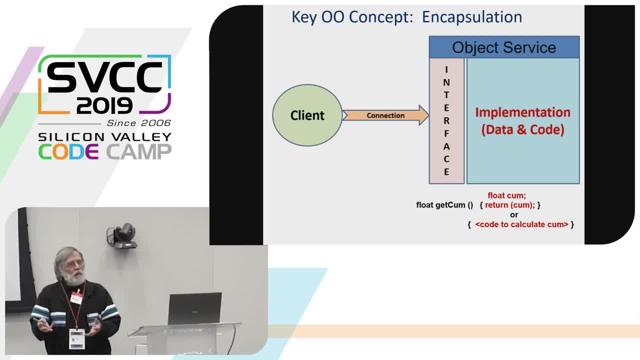 and i'm, i'm, you know, and i'm looking and i'm getting reviews you know of, of, yeah, i've gone to rate my prof and my review is up there, whatever you know. and now i've made the decision. now i'm going to say enroll, or buy it, or book that ticket, and or far away from the user interfaces which are 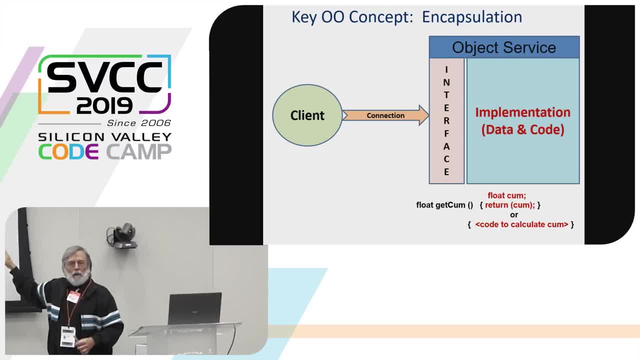 external to what we're doing. this is the back-end stuff that's going to make the world work. so that that's- and we'll see examples of of that. uh yes, wouldn't something like performance be an nfr? an nfr- non-functional requirement? oh oh, um well, if the performance is too slow, then it doesn't. 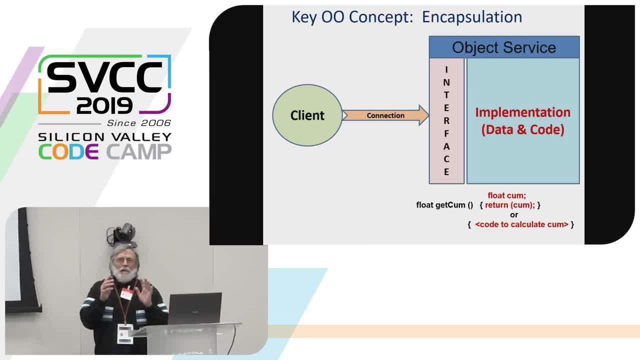 function right. no, but i mean you know, yeah, it's it's, it's it's it's it's important. people worry about performance. the programmers mostly worry about performance, but when you're doing a design, that's not your primary concern. your primary concern is usually encapsulating things so that change doesn't. 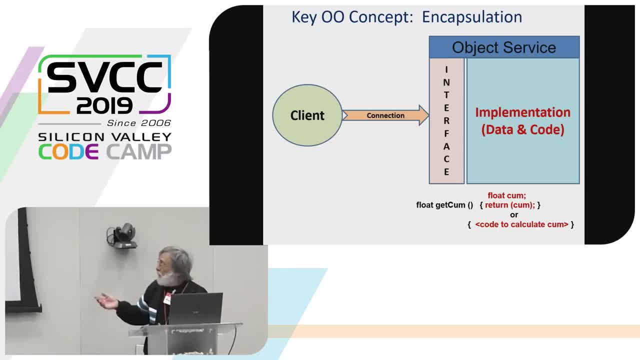 knock everything, everything over. and here's an example: right, um, you know you you've got some uh in a student record. you've got the cumulative average. right, it's one of the variables inside the cumulative average right now. if everybody could see that and go at it directly, if you then decided 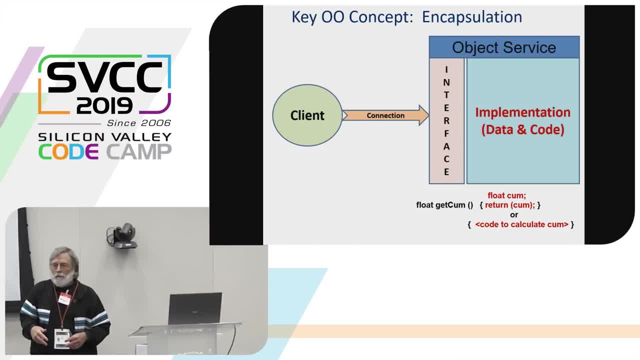 no, i'm going to calculate it. you're going to break everybody. whoever thought the cumulative average was an element in the structure of a student, whereas if you encapsulated it with getcume right, which is a function you call to get the cumulative average, you could decide: i don't want. 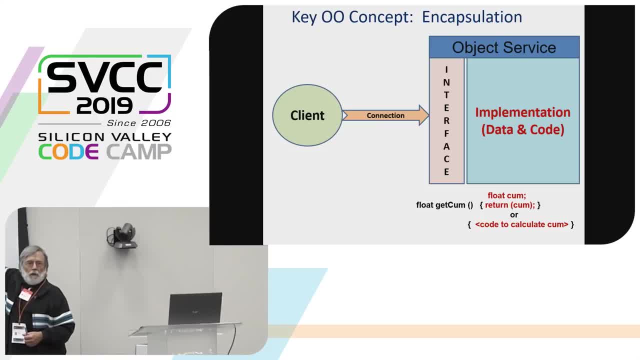 to store it here. i'm going to calculate it and you totally change the, the code and remove the object of the, uh, the attribute from the, the object and nobody else sees the change, because they only ever were calling the function to get it and the function has now changed the. 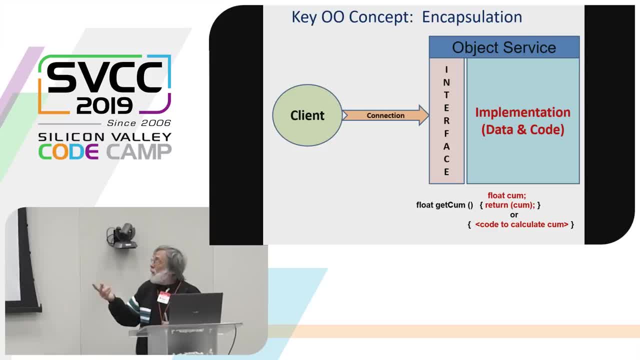 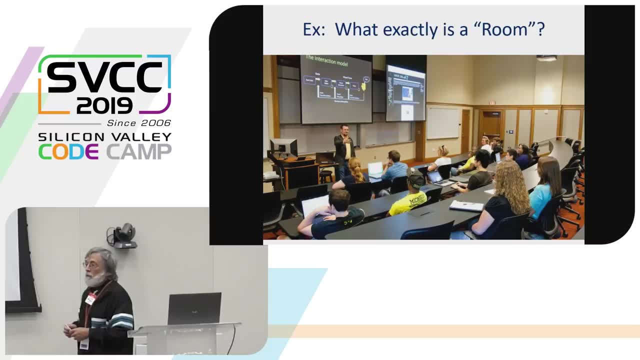 way it's going to get it, but it still has the same interface. so all of the clients never, never, see the change. that's one of the advantages of encapsulation. so, having said that, we're sitting looking at one of the objects that we've talked about. now we're it. we've stopped staring at the 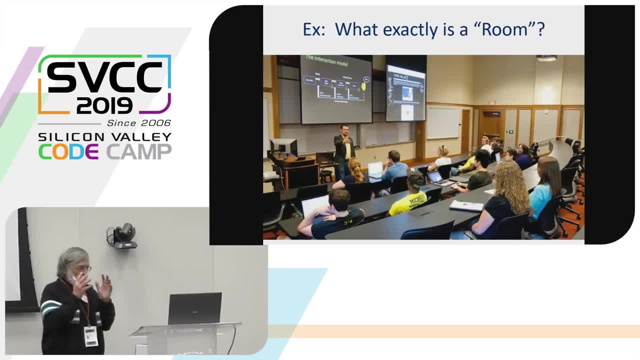 ceiling. right now we're coming in and we're saying, okay, we've got this room, we've defined this room. what exactly is a room? what are some of the attributes of a room? sorry, size, absolutely, size, capacity- well, capacity would be so right. the location right, because you're wandering around you. so it has a location, it has a size, it has 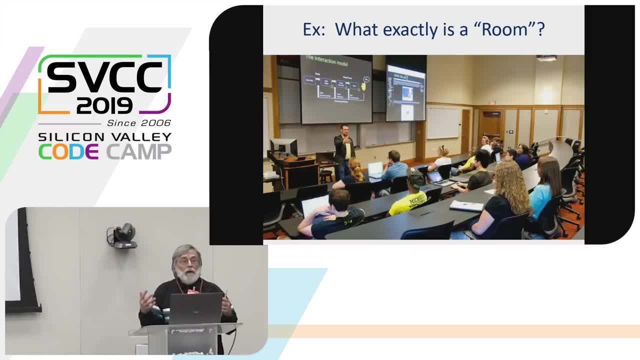 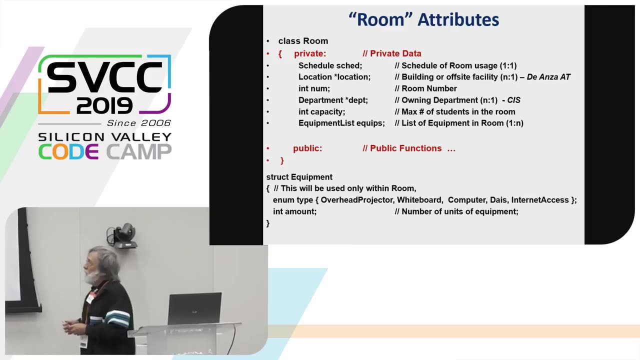 equipment, absolutely right. and it has some other stuff. it has a schedule. this is great. you take my course. um, all right. anything else all right, so let's look right. um, so, this is room attributes. uh, it's got a schedule. it's got a location. uh, it it's, it's got an owning department. 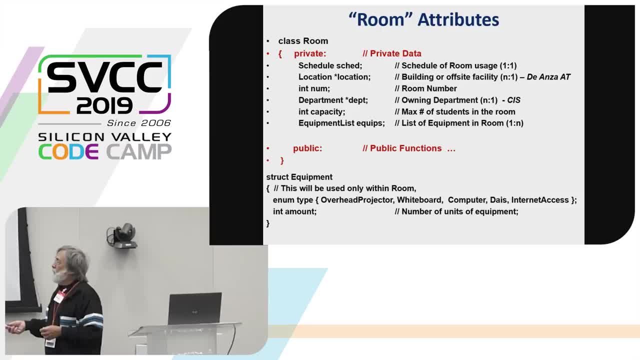 a capacity. it has equipment list where equipment is. there's an enumerated type of all the equipment that we have and amount. uh, it doesn't show a couple of things and again, this isn't directly this talk, but if you're looking at an object, you're and you're saying I'm looking at an object. 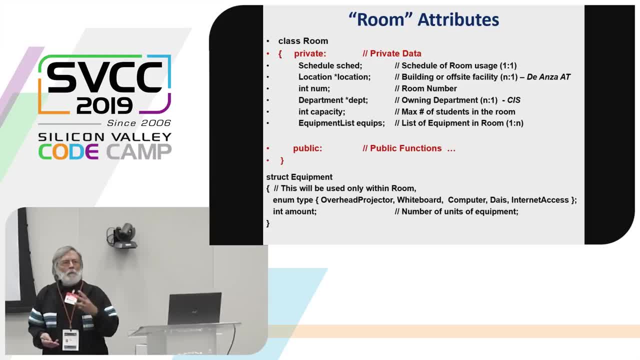 there should be three things you should be looking for. they're not always present, but you got to consider them and it's every object you ever have. one is the unique ID. what's the unique ID of this thing if it doesn't have a unique ID? I got to start thinking. 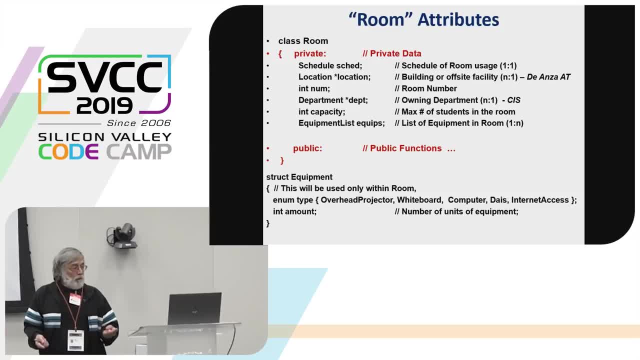 if it's an object. it turns out there's one object we looked at that doesn't that's seat. seat doesn't have a unique ID, but it it joins. so this, the ID of the seat, is the student in that section, but there's still an ID there, right? if your object doesn't have a unique ID, then it's. 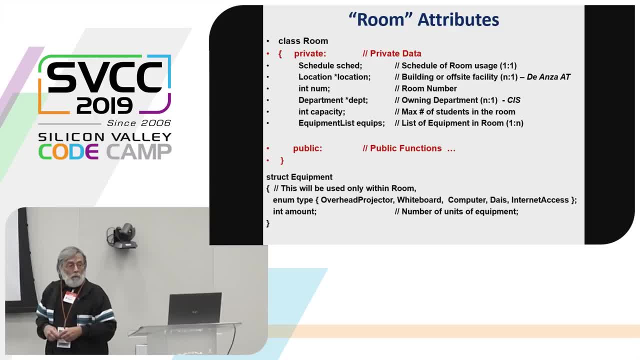 not an object. second is: uh, there's no number of seats. uh, there's no. it the capacity? oh, in the room? no, I wouldn't want to use a room doesn't really have the seats are tied to the section a room. yeah, that's true. how could a room not have seats? you, everybody sitting on the floor? 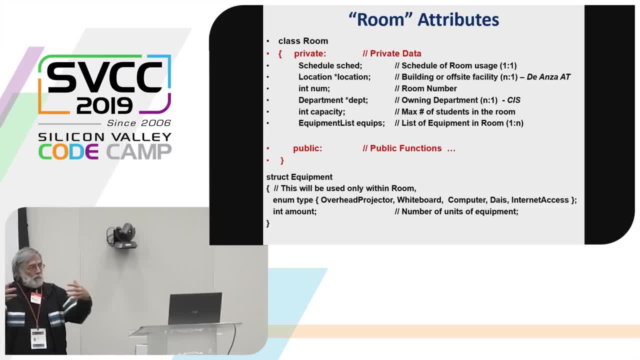 no, the but the seat abstraction is the thing that we call. that ties you. so it's a virtual seat and you're, as opposed to sitting on the virtual floor. yes, there there is. you're trying to you right, you wouldn't? you wouldn't say a room has seats, it has a capacity. thank you, you're absolutely correct. 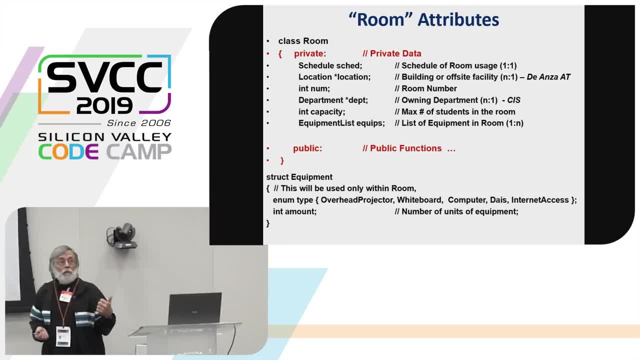 um, the other thing is. so one is: uh, does it have a unique ID? the second one is: does it have types? so, for example, on room, there could be a lab, that could be a lecture room, it could be. there would be different types. and whenever you get into types, that's the key to say, oh God, do I have? 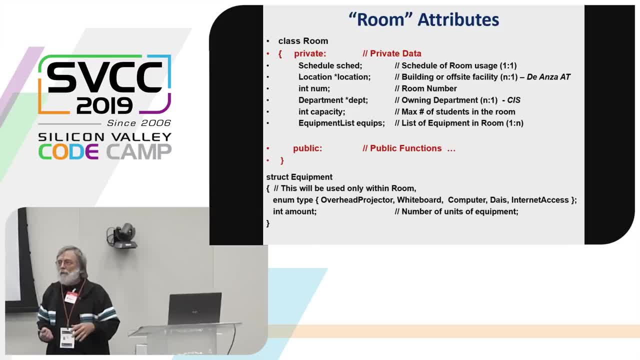 to subclass this right, because it has different kinds of types and there's ways- and I don't have time to get into design criteria- for deciding when you should subclass it, and one of the obvious ones is: does it, can it shift back and forth? uh, you know a part-time teacher, can you become a full-time? 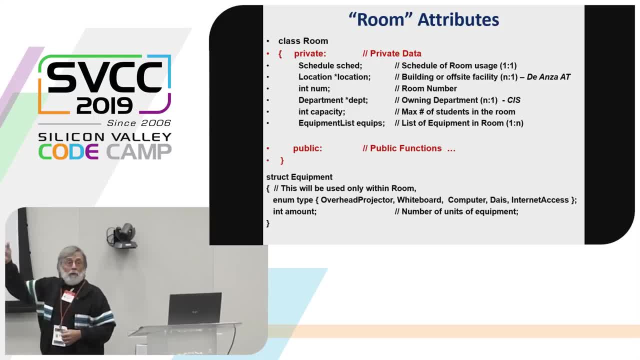 teacher, then don't subclass them, but the, but the. so that's the second one. and the third one is state. does this object have state room? typically doesn't, um, but a student certainly does, enrolled or not, or a section certainly does, uh, waitlisted, and so on. so those are the three things: type, state and ID. 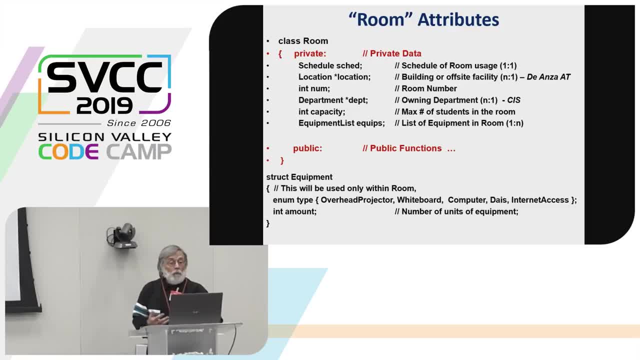 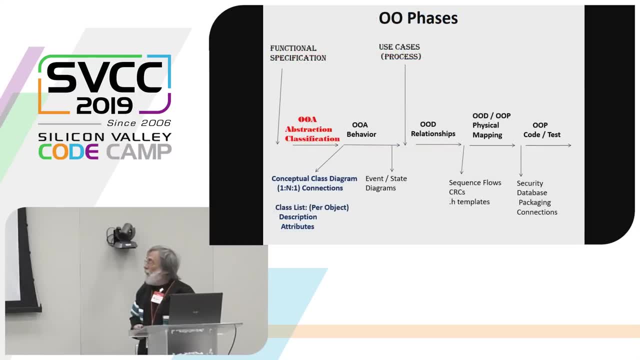 and and when you look at creating objects, those are some cool things to start thinking about, uh, uh in your objects that you defined. so we've um kind of uh come from here. we've said, okay, object-oriented uh uh, abstraction classification. we've looked at a conceptual class diagram, which is the high level. 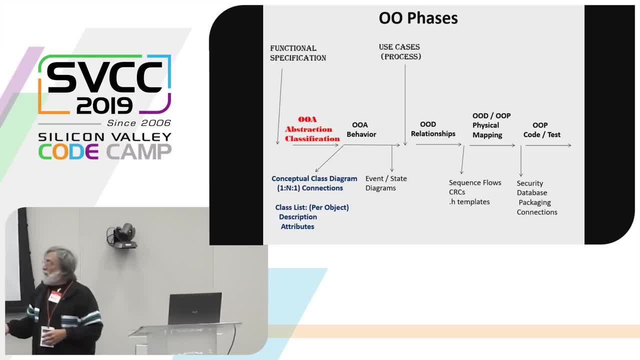 thing. it's an uml artifact and we've looked at a class list, which is again the thing we were just looking at for a room. it says: take one of these abstractions and figure out all the stuff that has to be in there. and now you, at this point, you've kind of 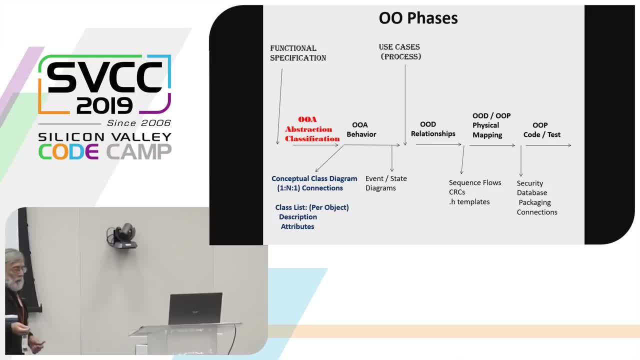 Oh, you've identified the basic set of stuff and you're now filling in. you're getting a better idea about what these abstractions are. Now. the next step, which we're not going to go to, is event state diagrams, where you start describing the 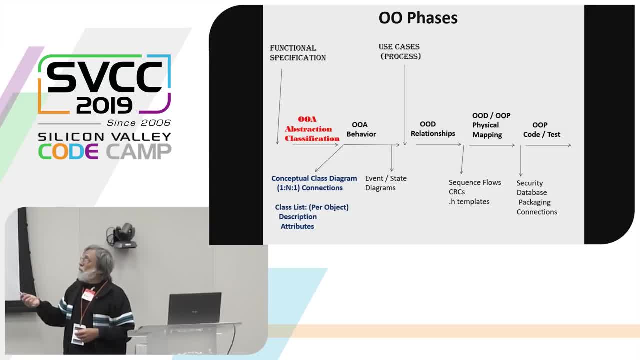 behavior and then again when use cases come in, like enroll student in section you, you have to then map to the objects, with the attributes and the interfaces and the behaviors that you've defined, how those objects handle each of the use cases. and that gets you into sequence flows. 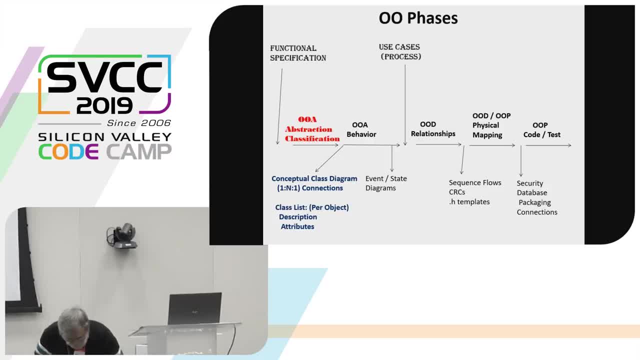 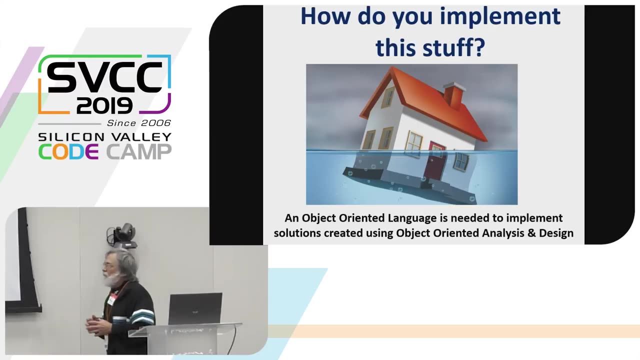 I don't need this anymore because I'm going to point that on tape. Great. So let's take a look at how do you implement this stuff, because everything we've been talking about has been kind of staring at the ceiling and thinking, Right, If we can't implement, 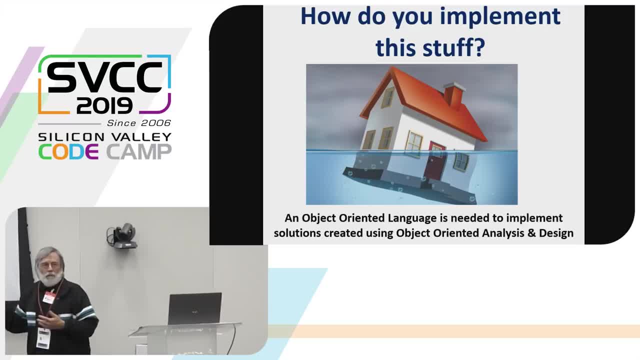 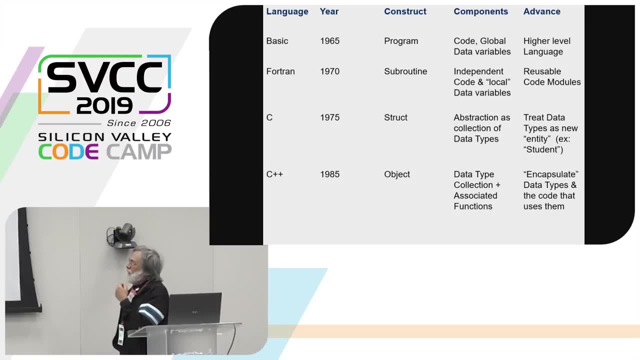 it, then it's like a house that we've designed, that we forgot the foundation. So this is in one slide right up through from the 90s, ok, and you could add Python, you could add Java and whole bunch of languages to it, and they had reasons. But the evolution of 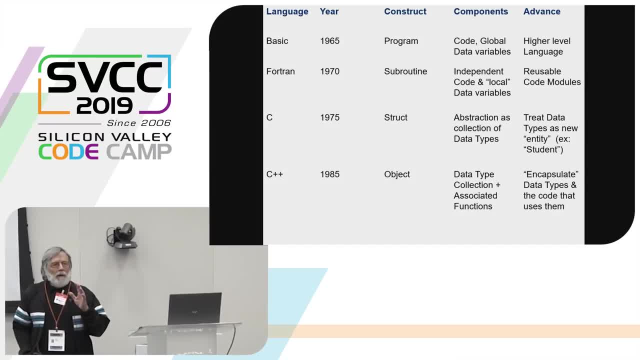 the twenty-year frame was all driven byCUPS object-oriented requirements. If you think about it, the basic, basic, which was the thing that Bill Gates is now a very, very rich man- was you had a basic program. It had line numbers in it. God help us. 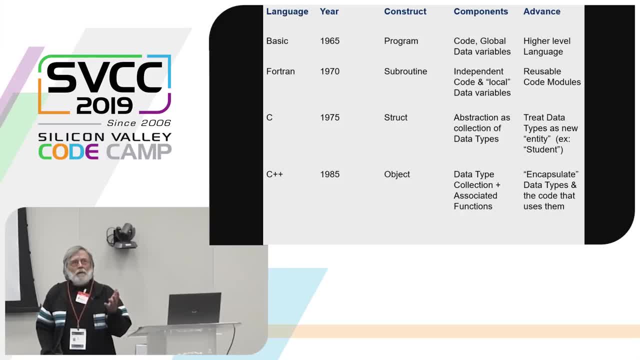 And you would write- this is where I usually use a board. you would write: go sub 600. And in the code at line 600 would be a bunch of code And then you would say return. This is considered a major step forward advantage from go to 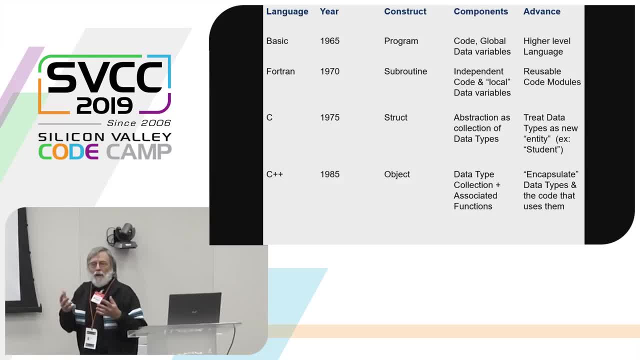 right, where you just go to back forth. But the idea was to take a chunk of code and reuse it. That was the original vision. That chunk of code was at 600. But worse than that, you could always renumber that. 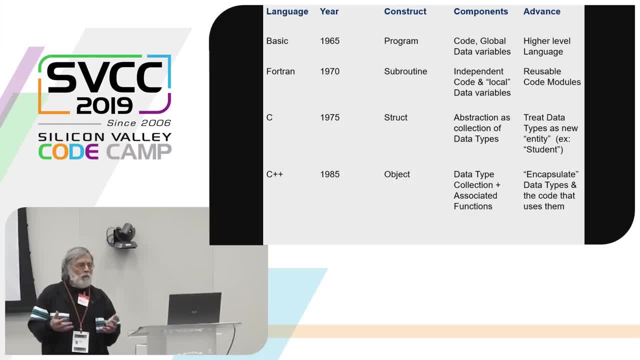 But what you couldn't do was change the variables, And the reason was that every variable in basic was global. So if you changed a dollar sign, any other application or any other sub program in that application just had a dollar sign creamed. It meant that you would have to when. 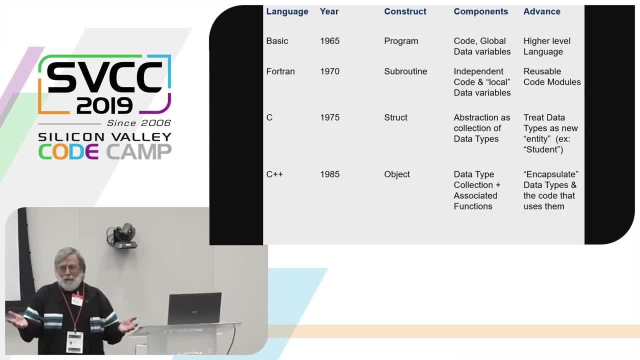 you try to resell your go sub, whatever the name of it was, to anybody else, you'd have to say, oh, and, by the way, here are the variables you can't use, which was ludicrous. And so Fortran came along. 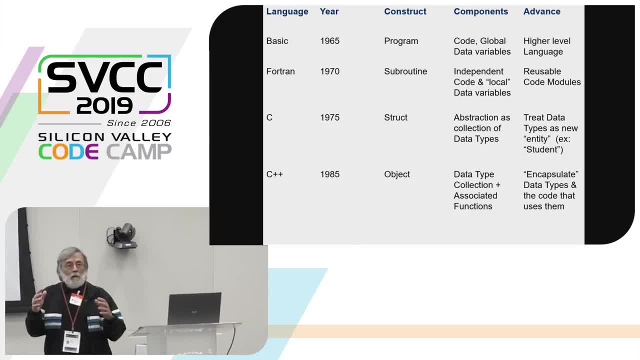 And Fortran said: OK, you know, we can fix this. And they did. Subroutines had a name That was cool, But, more importantly, subroutines had variables that were relative to the subroutine. So if you, in a subroutine, use the variable A3,. 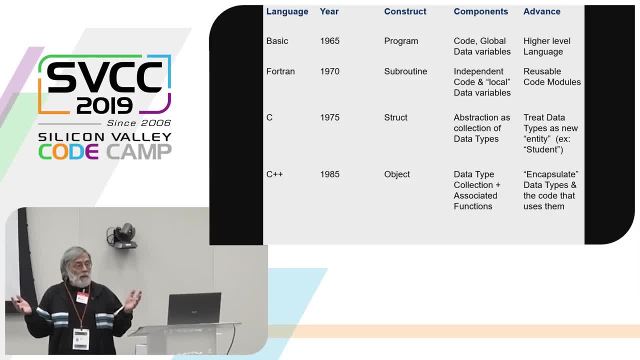 if you use a variable A3, anybody else using A3 was not going to get hurt, because that variable only had scope, was only defined inside the subroutine that you defined. So it meant that I could legitimately write for the very first time, subroutines. 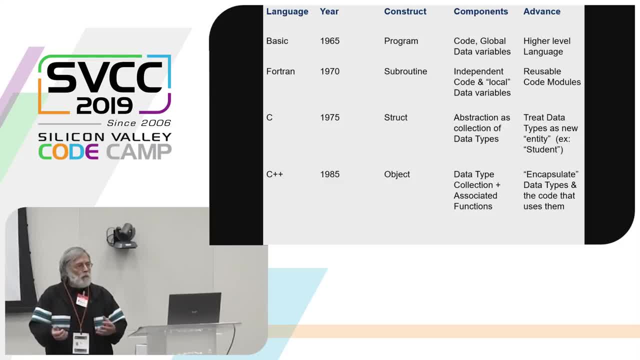 And I could give them a name and I could sell them or put them in a library and people could reuse them. It was the ability to cut a project into chunks and do some of those and deliver it- have separate people delivering it. 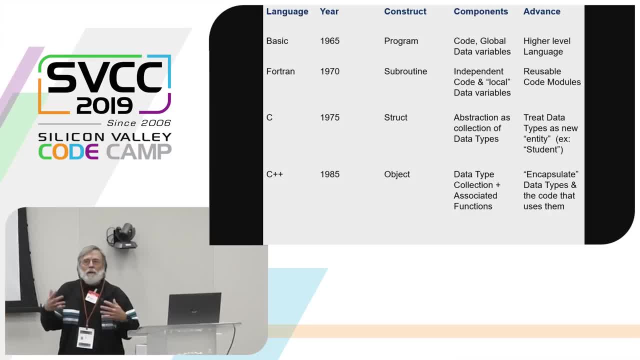 and then reuse it on other projects, And that was the beginning of subroutine libraries And that was cool. What you were doing was you were encapsulating the details of how you did it and you just had the arguments that were in the call. 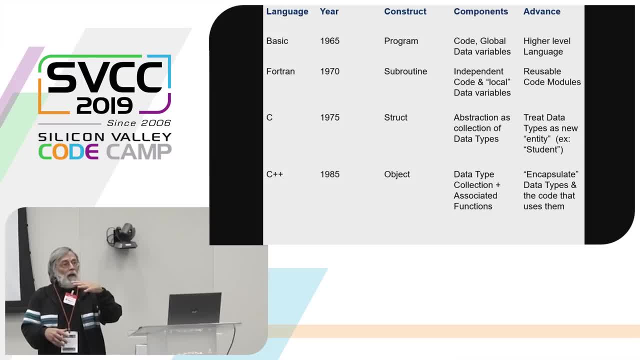 So the implementation was hidden and the interface was whatever arguments you used and whatever was going to be done to those arguments. And that was the state of things until C came along, And it was genius The moment I saw that. how many people have programmed in C? 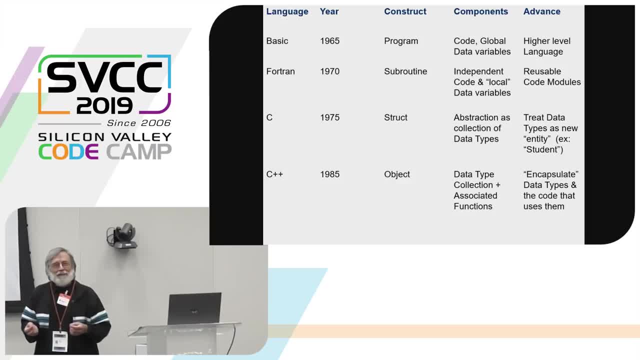 Oh yeah, Just great. So you're going to understand what I'm about to say. next, I saw it Before this. I'd been programming in a semi-language And I found out what malloc was. They said: if you want more memory, you ask malloc. 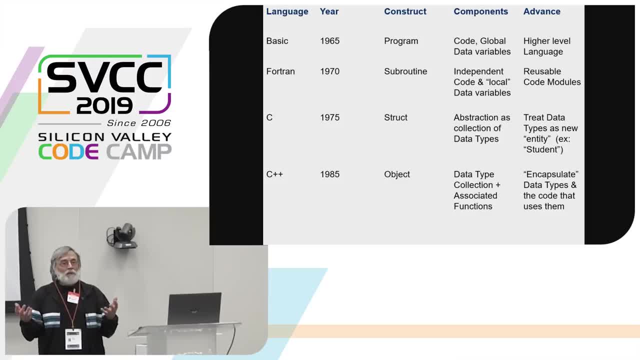 And I went right And I figured malloc was this ancient Semitic. god, Oh, malloc, please grant me, Because it was magic. It was magic, right, It was genius. OK, But more than that and more than the register variable. 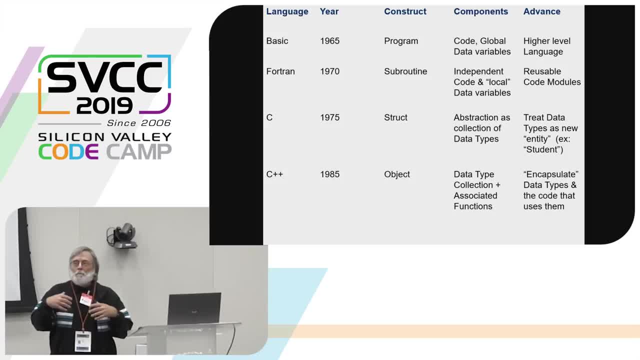 which meant I could actually put into a machine register something in a high-level language, was the struct. And the struct was awesome Because the struct said: you have a teacher, What are the components of that? And you could say: well, a teacher has an ID, has a salary. 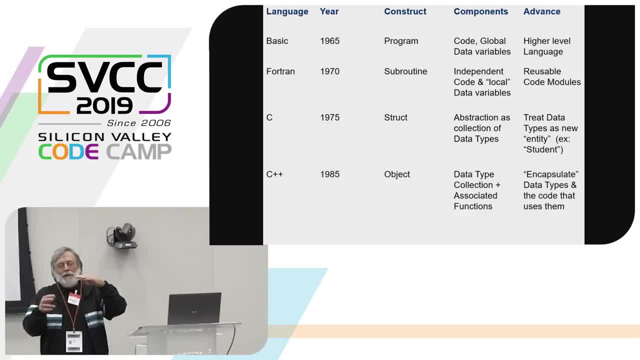 Now, in a better world, that salary would require a double precision, But it has a salary. Well, that would be an alternative universe in addition to the world, And it has. you know, And you could define. You could define the abstraction in the language. 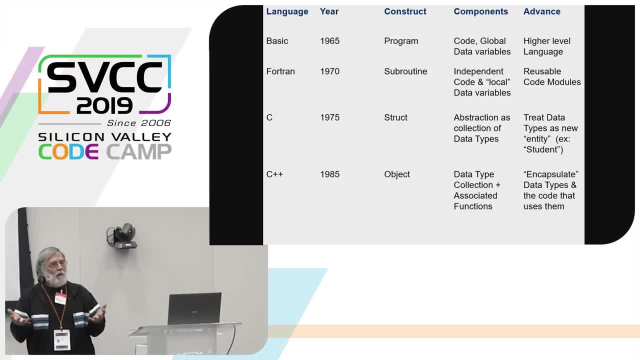 Before that you couldn't do it. You had the variables you had. You know you have to combine them into these overlap unions. It was disgusting. You couldn't represent what a student was suddenly with C. The good news was you could say: here is what this student is. 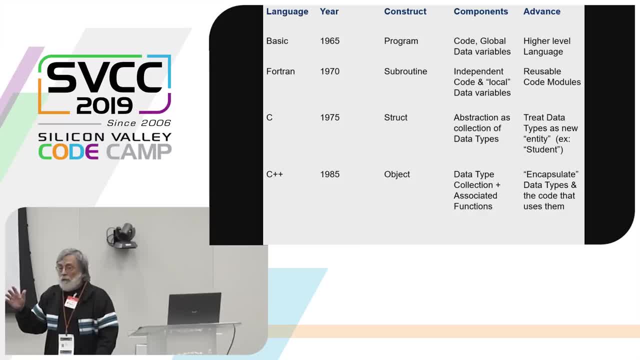 And you can point to it. You can have a ray of them, You can have arrays of pointers to them. They're like any other variable. Well, actually, no, they're not The reason that they're not like any other variable. 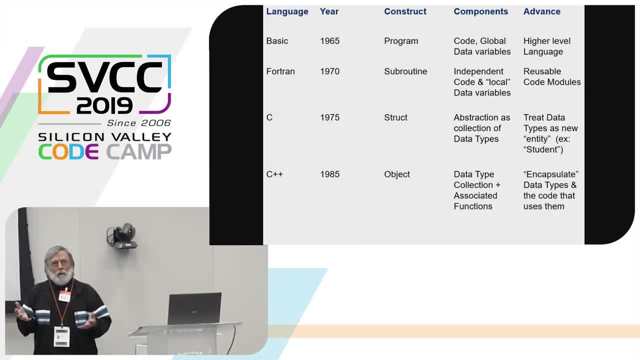 is because you can't operate on them directly. There's a thing called polymorphism, which I heard first time years and years ago. It was an object-oriented conference, when object-oriented was as hot as machine languages today. And, by the way, thank you for being here. 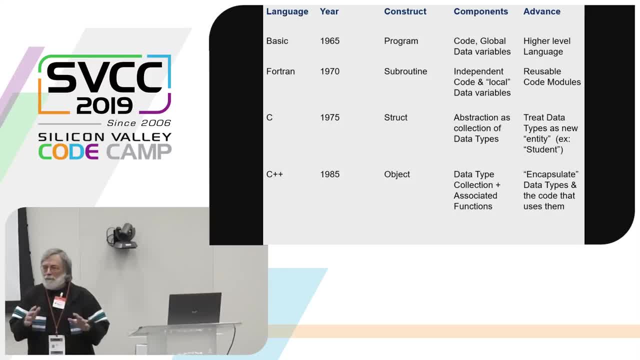 The words machine language is not in this talk And yet we still fill the room. I'm just so pleased. But they had a parrot there And the parrot was it. It could, It could say the words It was going: inheritance brock, polymorphism brock. 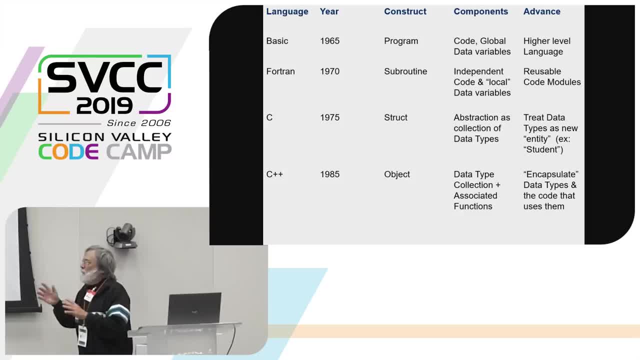 And then the guy said: we're not just parroting these words, We understand. Anyway, the point is that polymorphism says a very important rule if you're an object-oriented developer, which is: every operation takes on meaning. Every operation takes on meaning from the things. 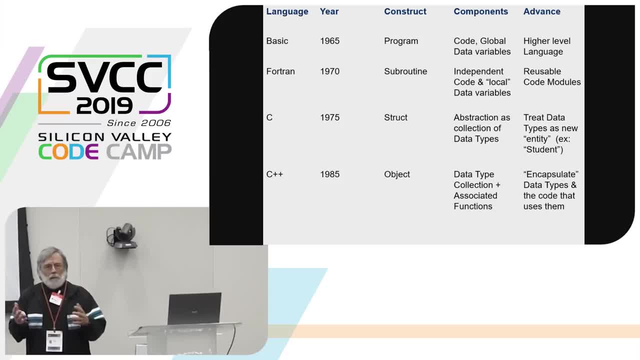 that it's operating on And plus you add two numbers. But it has a very different thing if what you're adding are two integers or two floats- Very different things, Different things happen. Conceptually it's plus, So what you start realizing is: well, adding a student. 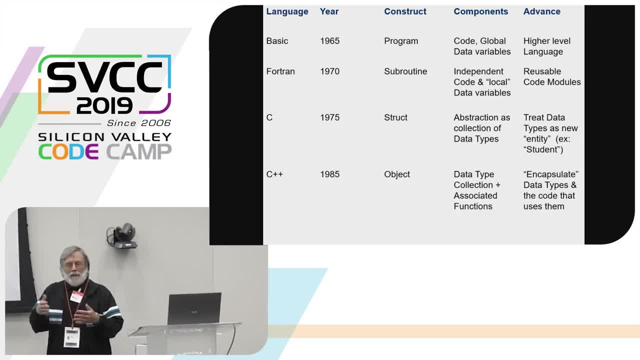 to a section is telling the section: please add this student, And it would be good, And you're going to be using the internals of both a section and maybe a student to do that. But then if any of those details change, everything breaks. 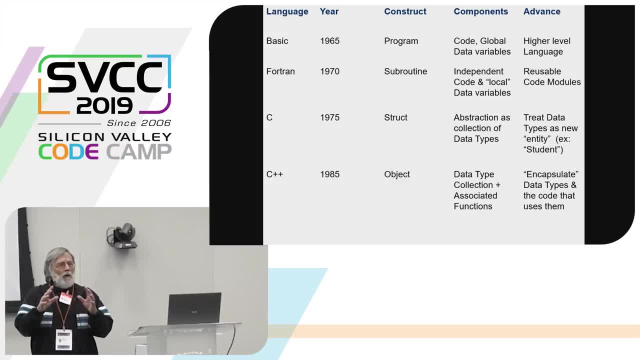 wouldn't it be cool to have all of the data inside of a struct private to the set of operations that use it? And that's what an object is basically. All of the data in the struct is now private, And all of the methods that use it. 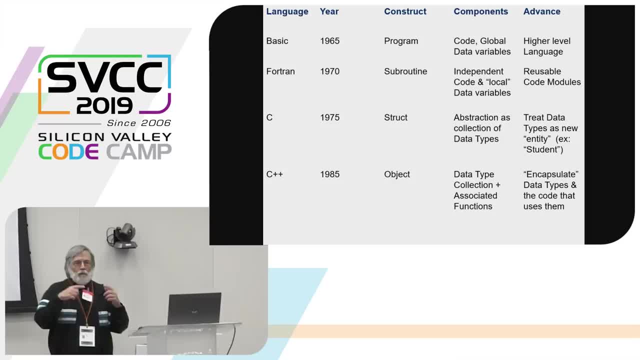 are now the public methods of that operation And can see. the public methods are the only things that can see the private parts of the object And it's shielded And the compiler will protect you against that. So what you had in all these cases? 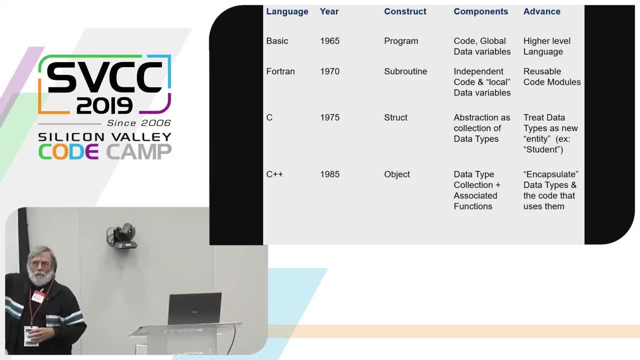 was. it was heading toward objects. First you could cut off a piece of code and return without knowing who called you. Then you had a name and arguments that were your own. Then you had data that represented the abstractions you were thinking of. 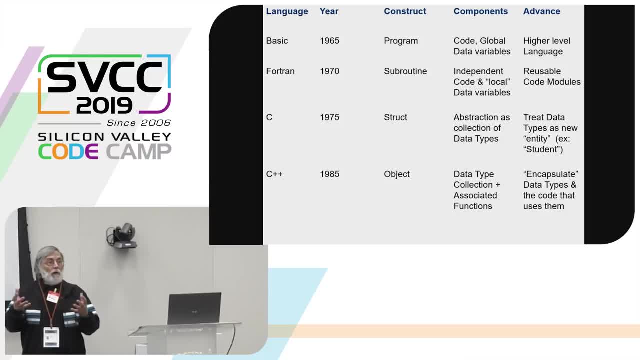 And finally, you had objects that combined the two, to say all of the good things we got about subroutines. we're now going to put all of the subroutines that had to do with this data And we're going to wrap it. 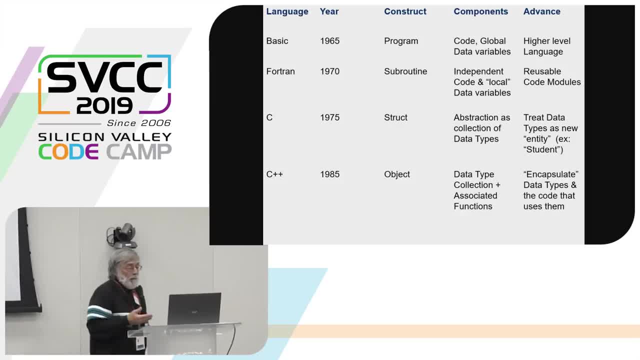 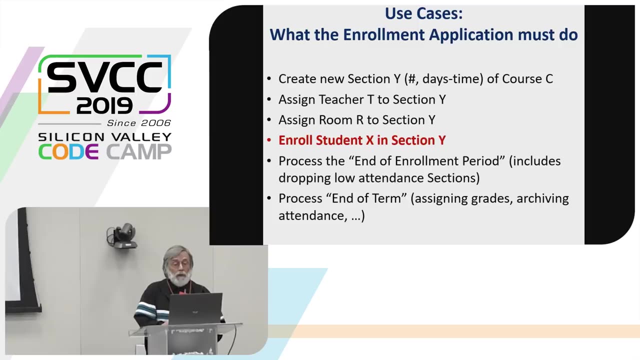 And we're going to call it an object And you're going to manipulate those, And so the languages were heading toward supporting the things that an architect and a software architect needed in the language It provided the foundation for the house. So this is a typical use case. 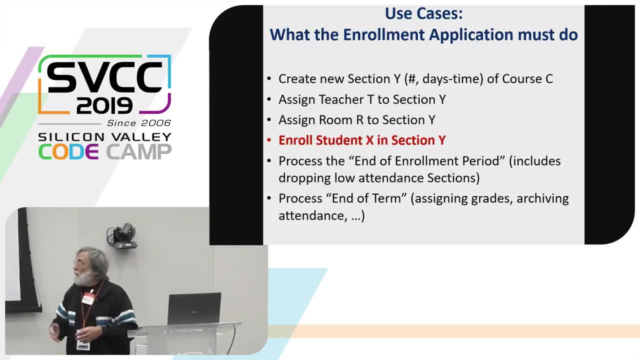 Once you have your objects and once you have your performance defined, and so on. this, this is what I wanted to say. Question: how are we doing for time We still have? are we almost out, or five minutes? OK, moving through. 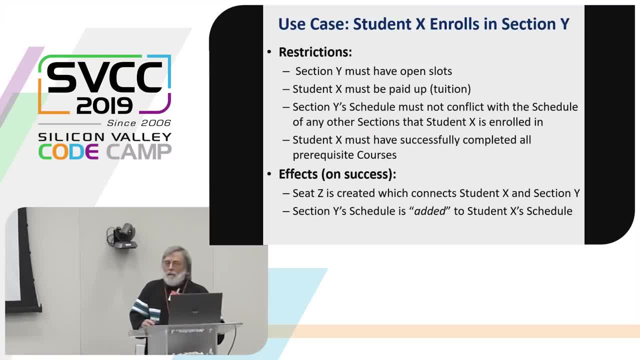 Thank you. OK, Just give us the history. Yeah, here's a no. I got no. there's a little bit more. I was, I was winging it. So the this is a typical use case, But this isn't really as critical to what I wanted to say. 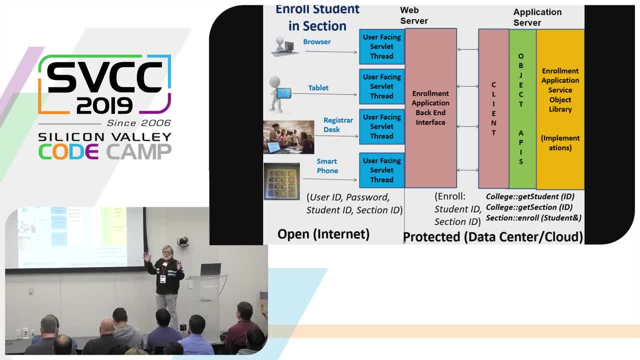 This is what I wanted to say. Where is this stuff working right? So you've got a three-tier architecture And your users are out here And they're going into a web service And typically there are servlets in. How many people know what servlets are? 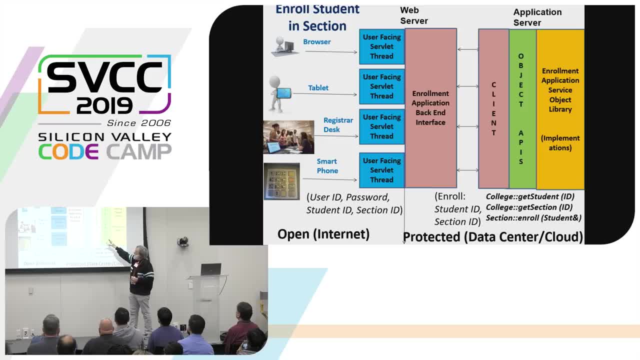 OK, less, but still good. It's threads and it operates in a web service, And so out here you're gathering things like user ID and password That set up a session, And then you're going to say: oh, by the way. 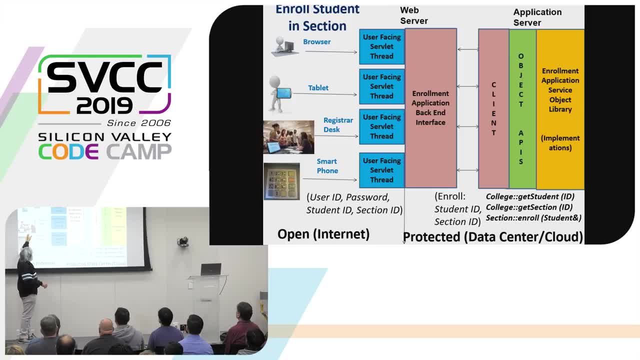 you're going to one of your applications. you're going to be sitting at your terminal or your registrar desk or tablet. you're going to go register me in sections you know, CS2807.. And that's going to come across the internet. 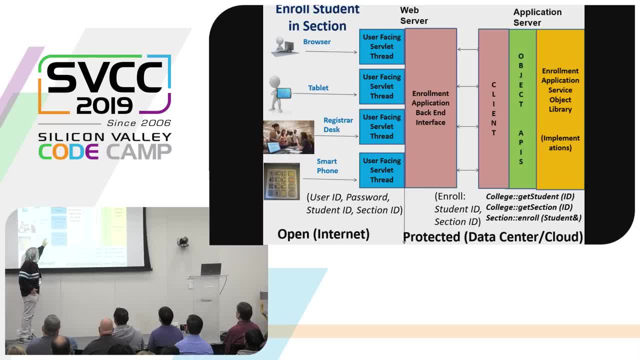 And it's going to be validated here in tier. this is tier one, This is tier two, And what could be bringing this over is JavaScript, Ruby on Rails, whatever- Over here, for the most part, you're now, and so that will then put a stack of things to do. 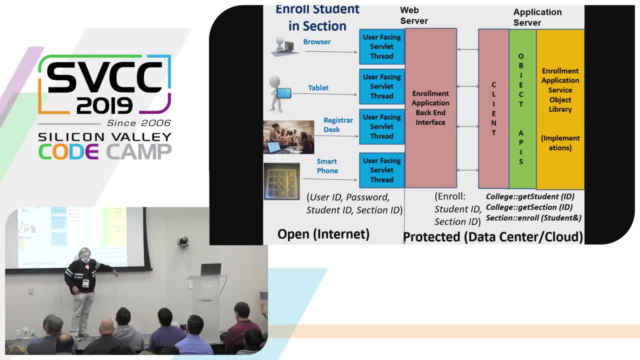 There's a thread sucking that off and shooting it out to tier three, which is the application service. What comes across This is typically REST and JSON between the tiers, between the web service and the app service, And they had the author of JSON speaking yesterday, which is cool. 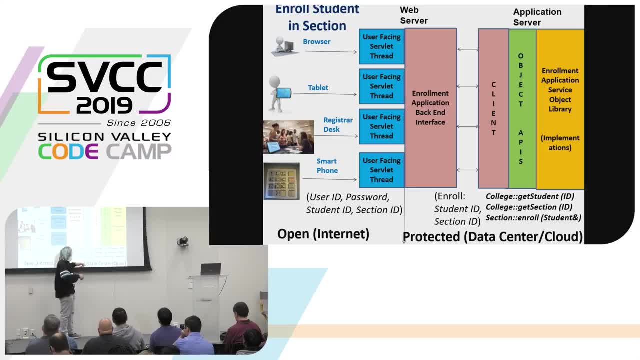 And then what you get is basically enroll student ID in sections. So these are strings. That's all that comes over. That's your command, That's your use case. Enroll that student in that section. The client is the main line of the program. 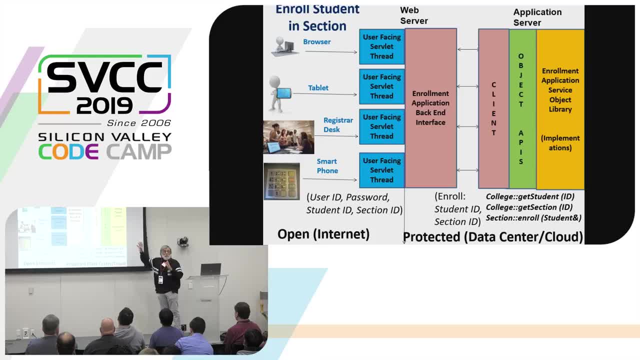 This is an application Application service, And that's the thing that a lot of people don't see. The client receives the commands coming in from the web service, the requests coming in. Each request is a use case. It's a thing that- and there's maybe 30 of them- 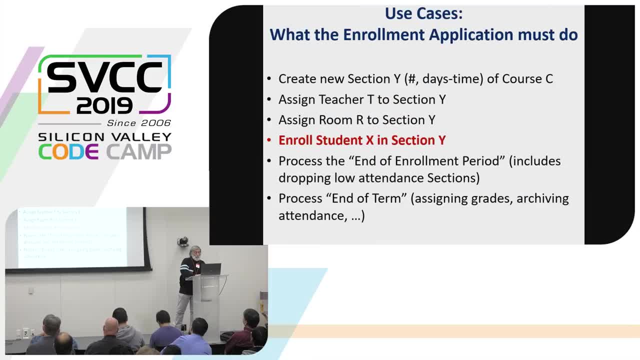 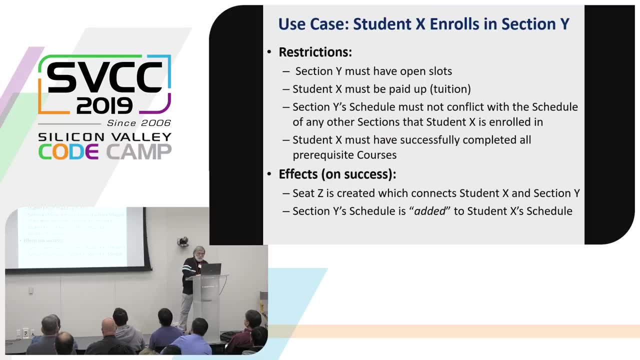 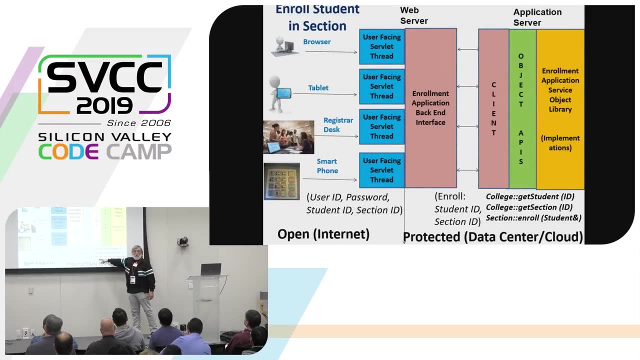 for this particular application. Here we go, use cases: Assign teacher to section, assign room. Those are commands coming into our application. The client is the main line And to do enroll student in section. what the client says is it asks the college get me the student object given. the ID is 1234.. 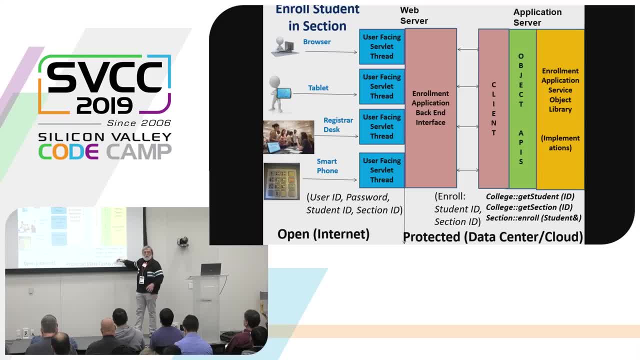 Then it says to the college: get me the section whose ID is CS2873.. It's got both objects. And then it says to the section: enroll that student. The client is the ones making commands on the object library. The thing to understand is that the object library 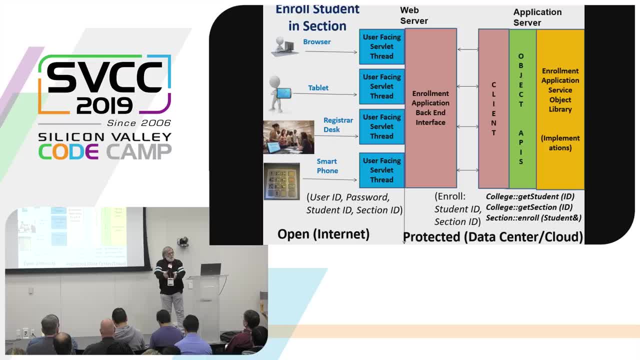 unlike a regular object library like date, where you say what's the date, here's the date. Here you say enroll student in section And it looks like a pinball game- Objects calling objects calling objects to do that enrollment, Because you're doing all the things in the use case. 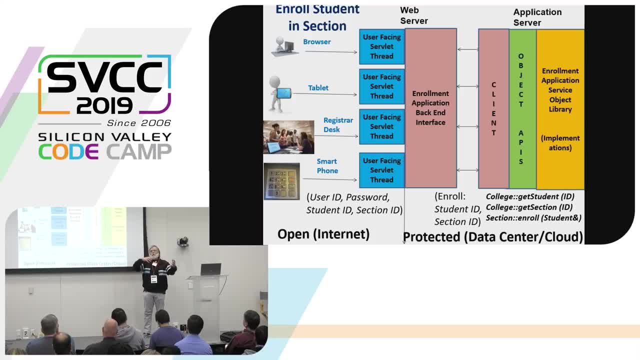 Are the schedules OK? Is the student paid up? Is the student quality? Have all the prereqs? All of that's being happened because we've understood and we've designed the objects to handle methods, And most of those methods are being called by other objects. 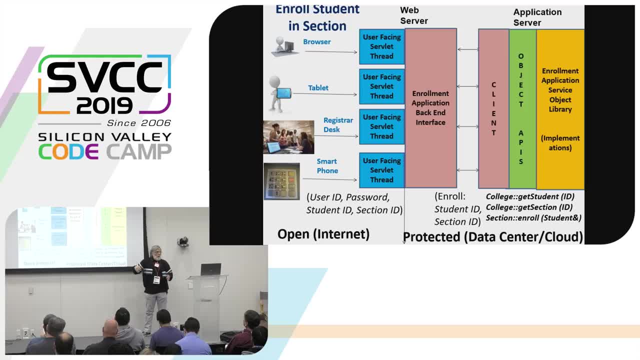 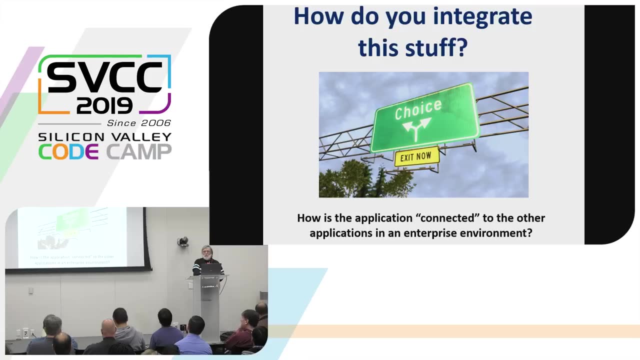 And eventually what comes back is yes or no. And now the question is: this is one application in an application service in an enterprise with many, many applications. How do we connect it in to the other applications in an enterprise environment? There's only a couple more slides left. 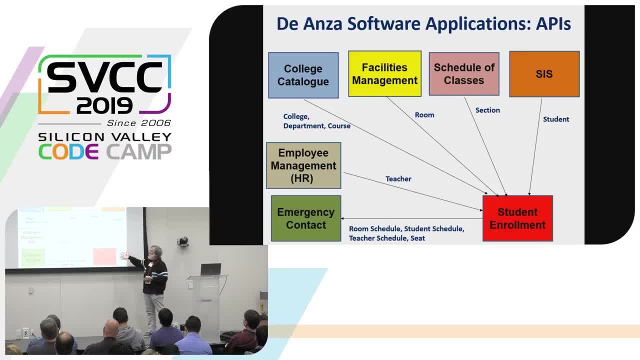 So you think about the things that we draw on in student enrollment. OK, OK, You know, here are some of the applications. There's a ton of applications, even in a simple college right. There's a student information system. There's a student portal. 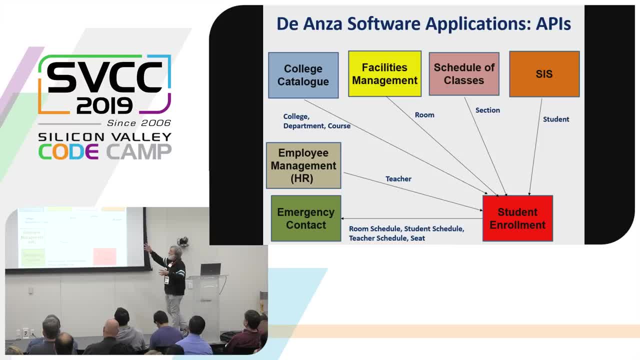 There's a thing that schedules classes. There's a facility management system that takes care of the rooms. There's employee management system that has things about the teachers- All of this. we're going to be drawing on this. How do we get all the information? 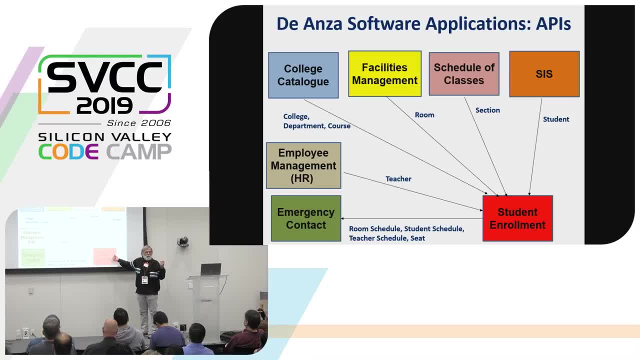 that we need about a student. We have a student's ID So we can go and get the information we need about the student, Because somehow we're linked into these systems. And there's two ways to do that. One is through a message broker, which 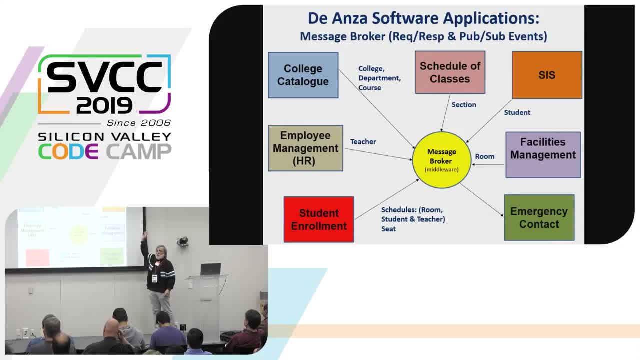 involves middleware, where we make a request And the message broker figures out where it goes. This is an architecture where each application has its own data And the only way you can get at it is through requesting it, And so we are basically sitting in an environment. 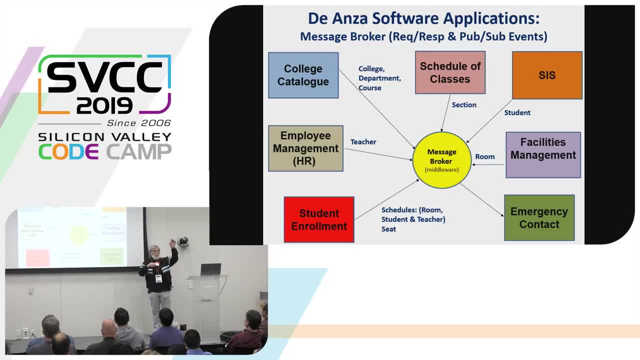 on an application server where we are calling the message broker to call other application servers giving them the requests. The one thing You know if you're an application server is the request wouldn't have gotten to you if it wasn't valid. So it solves a lot of the security issues. 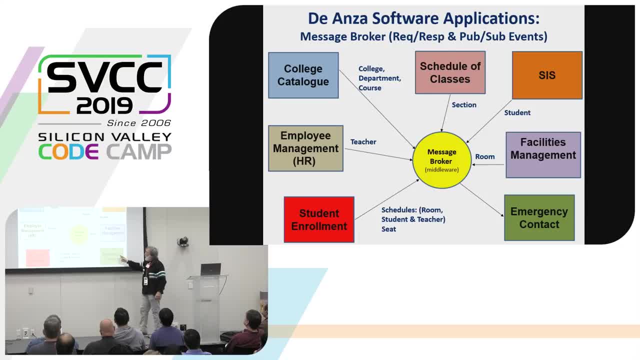 that you might otherwise see. And also we have things like the things that we maintain are the schedules and who's in a room, So the section's in a room and so on, And there's an emergency contact system that says: armed shooter in school, who's in that room? 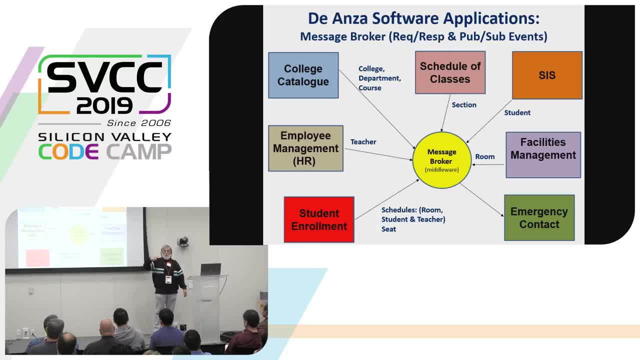 And they're going to use our stuff, our schedule, because they know that room has a schedule. It's this section. OK, who's enrolled in that section? They get data from us. All of these things play together And this is the other way to do it. 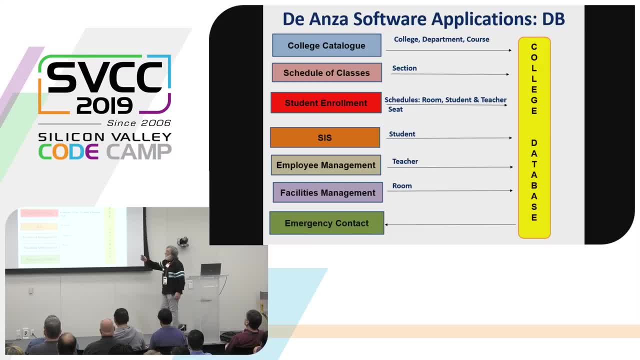 You have a common database in tier four And your applications make it's easy to make SQL requests to get the data. It's not so easy to tell the database. I'm updating these fields, But this is a second alternative to you know. 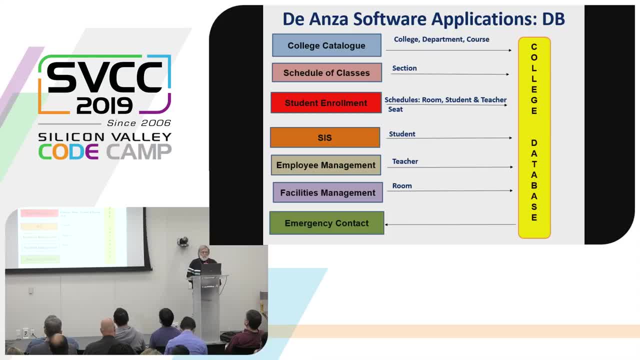 if you enrolled in a section, you're changing data in multiple places. You know like you're changing data in multiple places, Like you're being billed for it, Your schedule is changing, The section seat is filled. All of those are changes that are recurring. 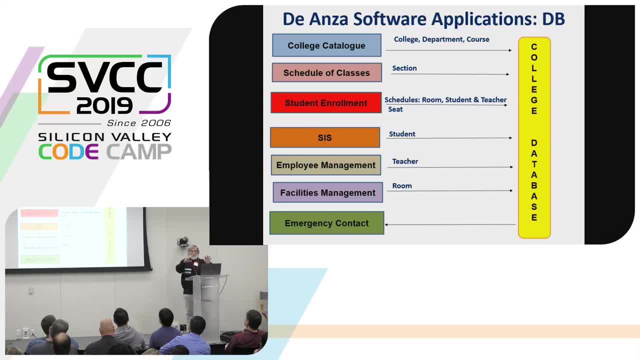 and have to be reflected in the database, And they can be reflected by the individual objects that own those databases, Or they can be reflected by you going into the database system. So whoops, yeah, one second. So how to become a software developer. 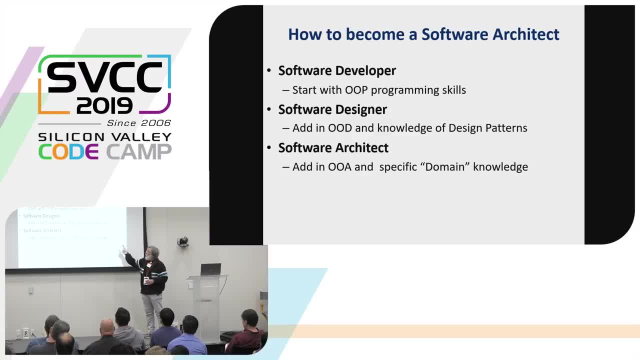 There's exactly two more. There's one in the next one, which is a lollapalooza. So the software developer: you might start with getting OOP programming skills, learning about design patterns, And then everything. a software architect. 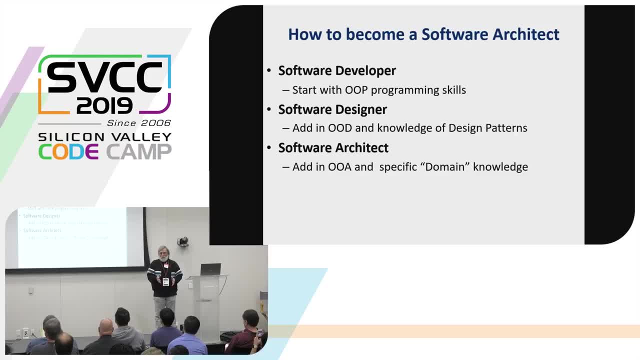 is, by definition, in one domain. If you're, you need the adjective- You are a retail software architect. You are a travel industry software architect, Because you are architecting in a space of applications. What I just showed you was something that an educator, a 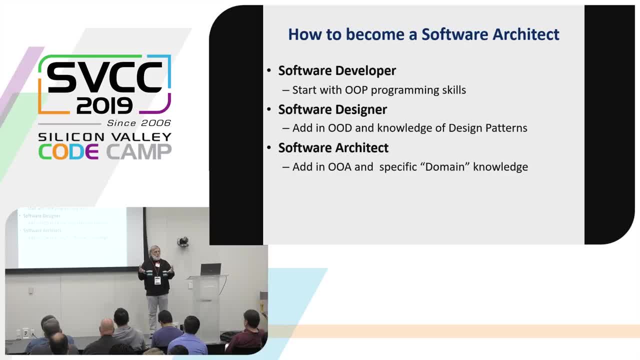 vocational software architect would live and breathe. But other industries wouldn't know. And so you know, you are. you know how to design houses Or you know how to design bridges, But the two don't necessarily carry over. I wanted to show you. I'm hoping this is the next slide. 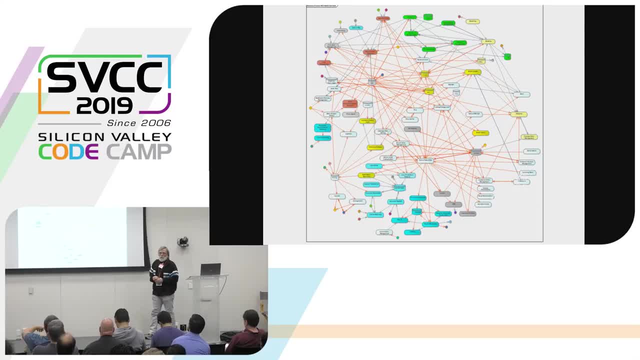 It is. So here is the model for retail. If you are a retail architect, you live and breathe this stuff And you can. this is where I wanted the light pen, of course, But what the hell? You look at this and you go. what is this? 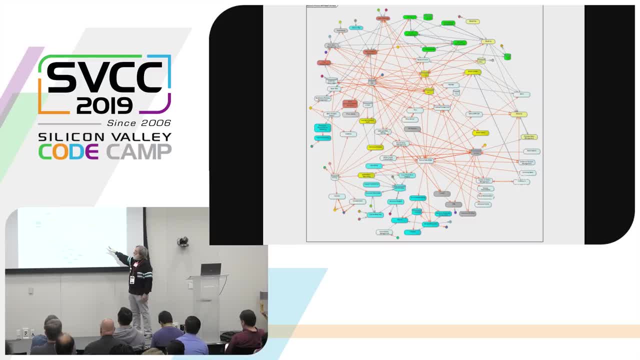 These are the systems and the data stores for the things that are in retail, And an architect knows this and knows how to fit stuff in. So here's: you can look at this thing with 100 things coming out of it. That's point of sale. 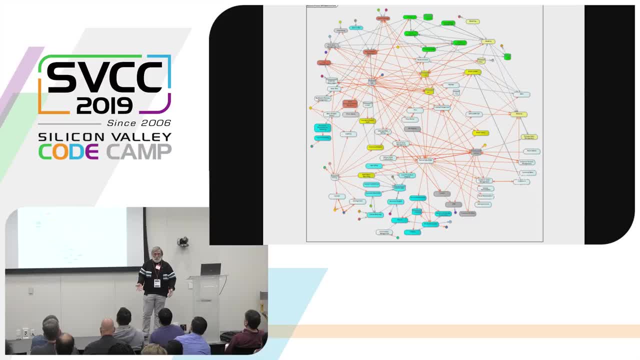 All God's children want to know what happened at the point of sale. All the systems want to know. Because you're going to decrement inventory, You're going to reward the clerk who's really moving sales through if it's in a store. You're going to want to deal with coupons. 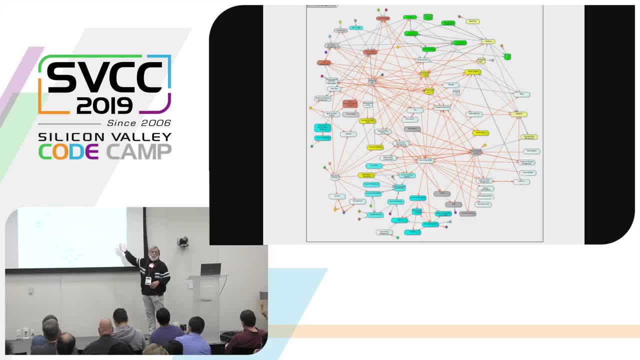 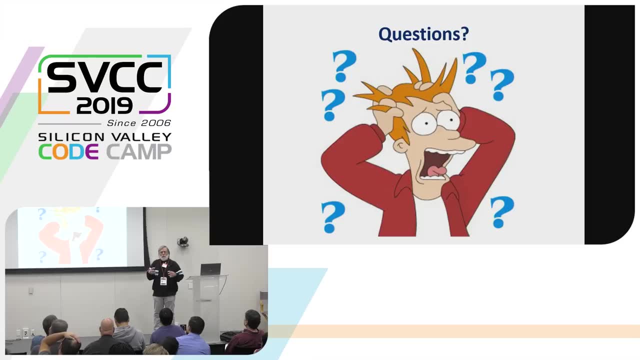 You're going to want to deal with loyalty cards and discounts. You're going to want to deal with again keeping track of inventory price optimization. We've detected that it's raining outside, So let's increase the price of umbrellas. 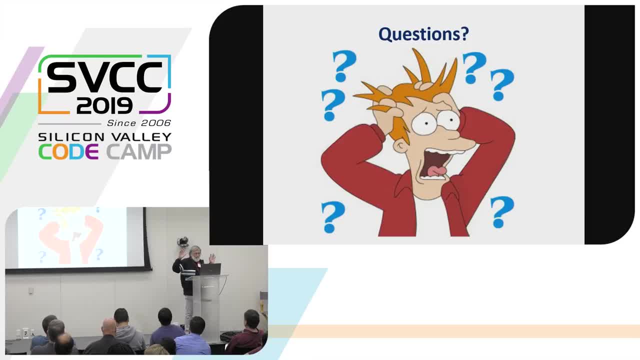 Yeah, hey, that just did it by itself. That must be. my time has run out, But that last slide was supposed to convey the fact that everything we're talking about- working your way up to software architect- it happens inside of an industry. 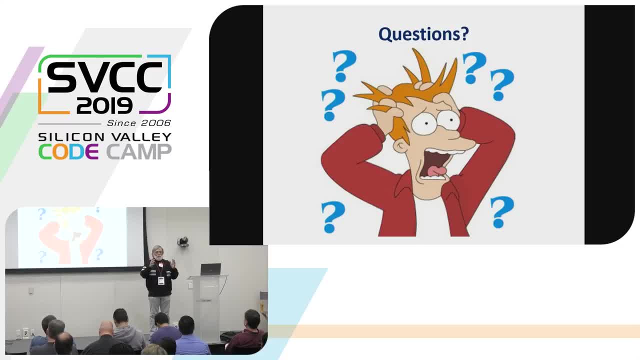 And your career path is in that industry, So you better pick one. And they're different, They are very different, And the 30 seconds left- and I'm going to do this because it's interesting- Like retail is just kind of a basically. 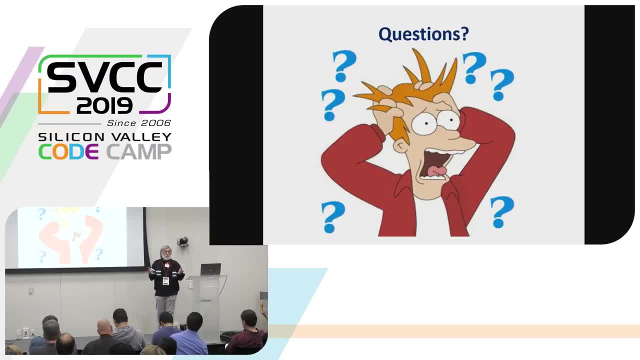 a business model- Basically a bunch of white guys smoking cigars. OK, Education and health care are very different. You've got people in those industries who care and want to make a difference, And they also have one thing that other industries don't have. 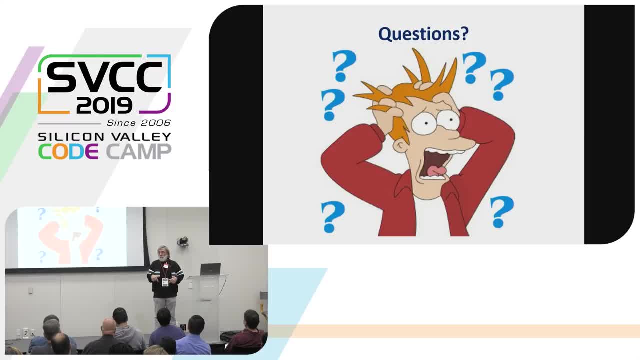 The end users cooperate- If you're in insurance or you're in travel or so on, and you find a good solution. you don't tell anyone, Whereas in education and health care, you're up on the stage talking about it. So again, it's a good one to do. 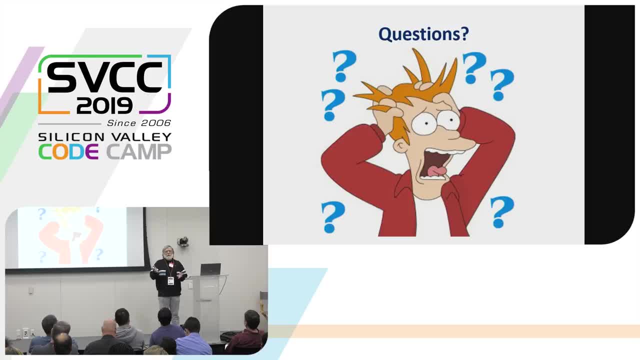 And the other one: how do you tell if you're talking to an extroverted research scientist And the answer is: he looks at your shoes when he's talking to you instead of his own. Point is: you can find out a lot. 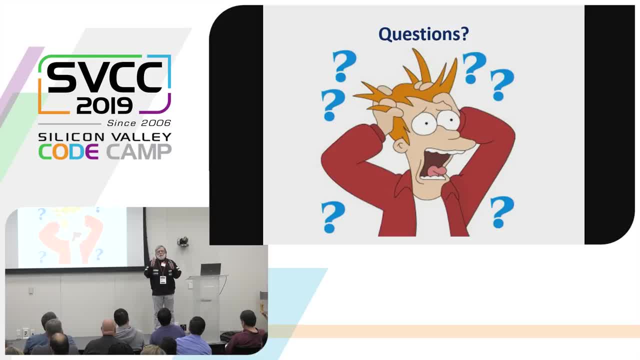 Different industries attract different types. So my last point is: if you're looking to become a software architect, pick your industry And then start working your way up, And that's how it's done. Thank you very much for your time. Thank you.